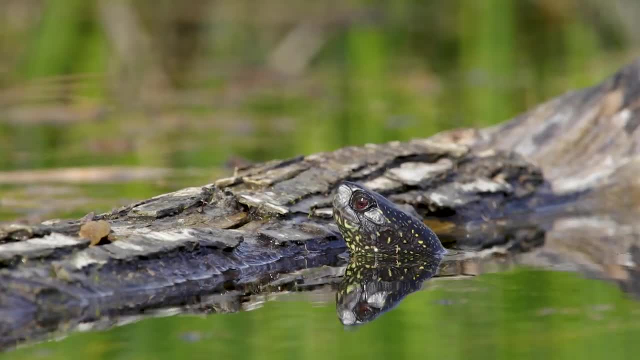 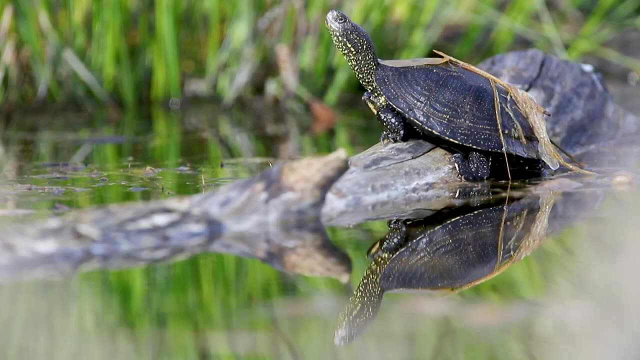 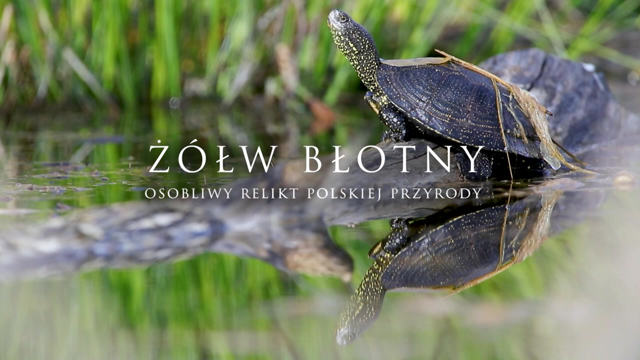 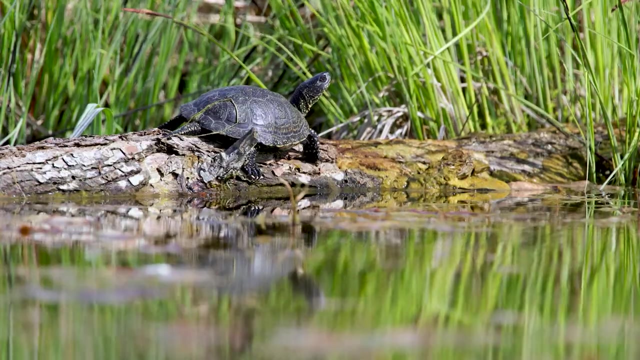 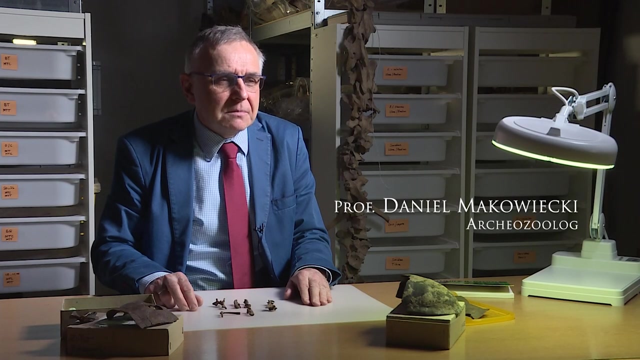 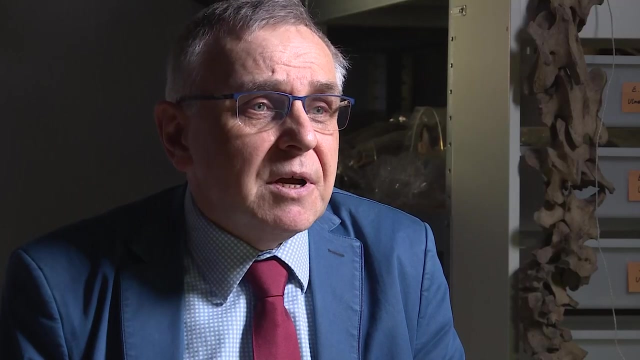 This is the best time to make observations, as the coastal vegetation is still sparse. The European pond turtle, a unique relic of Polish nature. The history of the turtle, the oldest one, can only be studied through the findings of it during excavations. 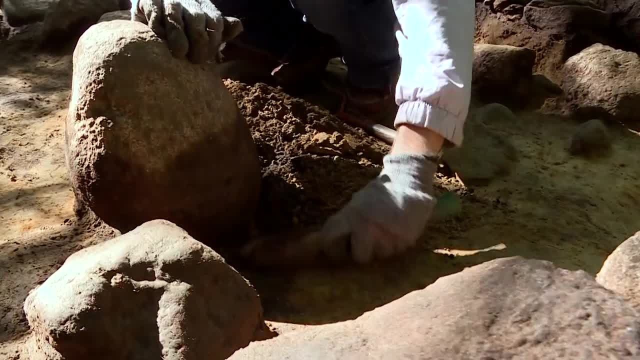 It appeared as early as the Ice Age. but in these obviously warm times, We know that the closest place from which the turtle was discovered was the ice age. The ice age is the time when turtles were first discovered. The area from which it spread to central, northern and western Europe was the southeastern. 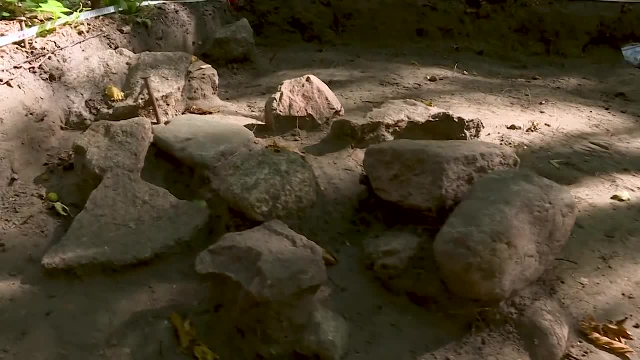 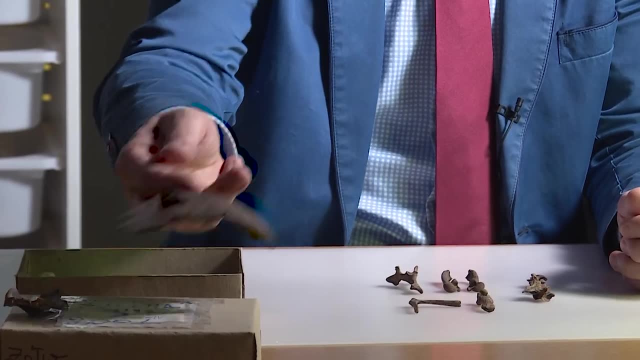 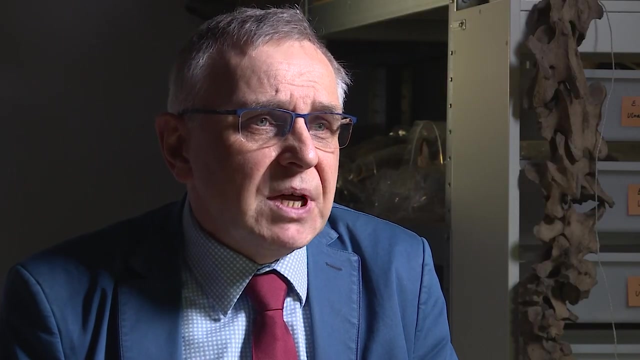 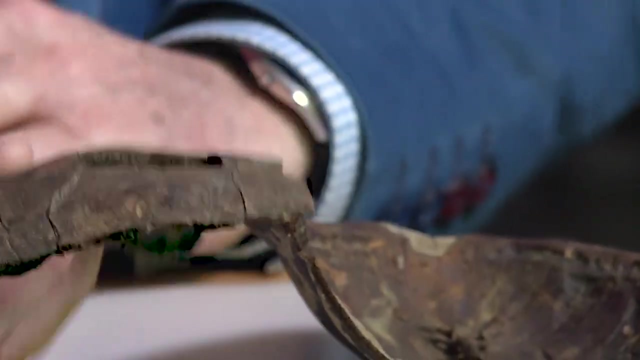 Balkans We have the first discoveries of the European pond turtle around 12 or 11 thousand years ago. But the best time for the colonization of these areas was in the pre-boreal period, That is, after the end of the ice age and the onset of what we now call the postglacial. 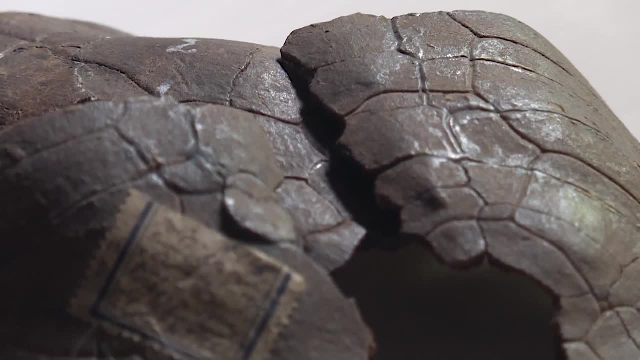 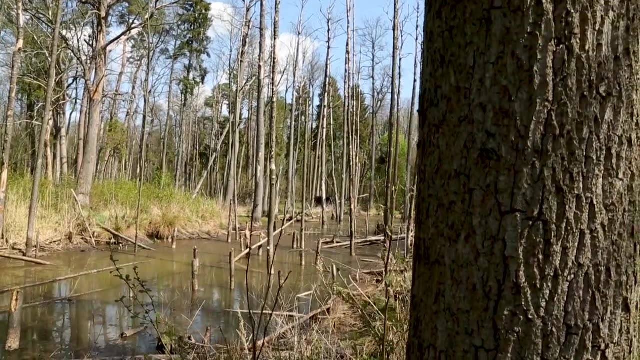 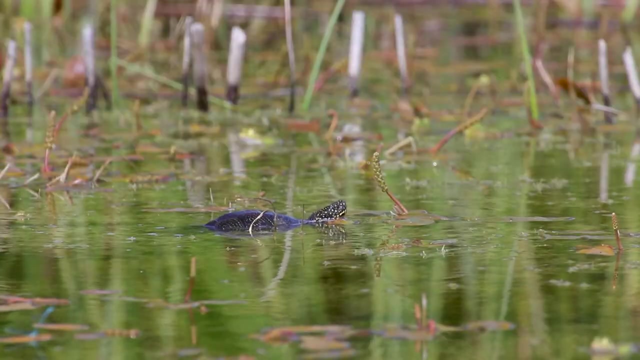 period, the Holocene. In Poland, the mating season of European pond turtles begins in April and lasts about two weeks. The courtship and copulation, called amplexus, has been maintained for a period of nearly 1,000 years. 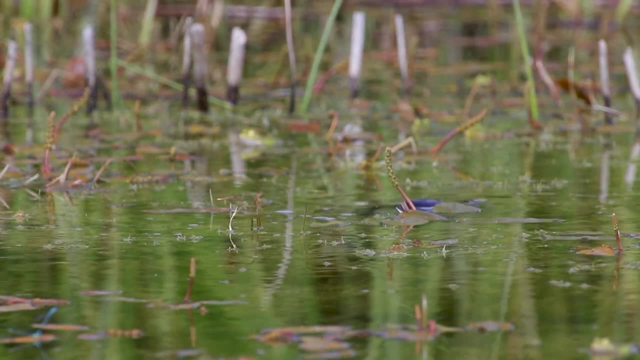 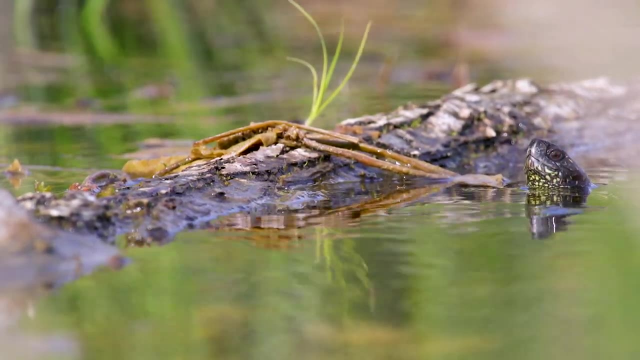 The wild term in the region of the Eastern and Western European platea is the mostיעigen time of the European pond turtle period takes place in water. The couples can be seen swimming just under the surface of the water. The female has a smooth plastron. The male has this well in. 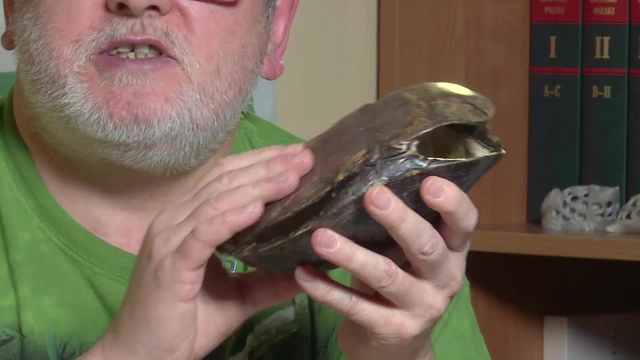 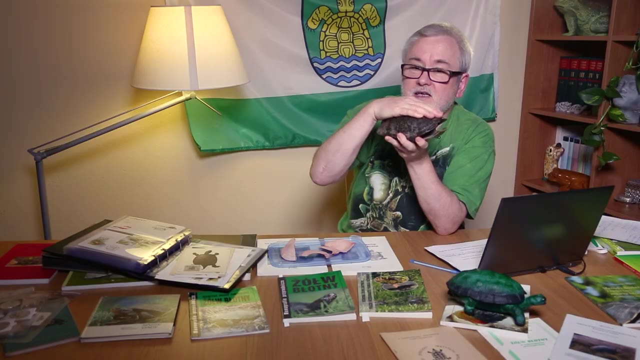 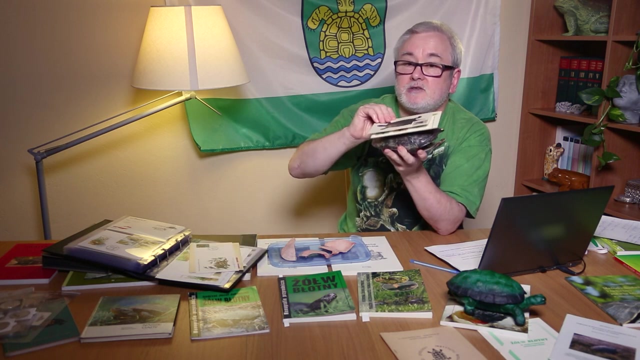 inverted commas, small but really not large hole. This is one of the most important features because, thanks to the fact that the male has a depression here on the plastron, when he enters the female he doesn't slide off her because, let's imagine, it's completely straight, just like here. so he would slide down. 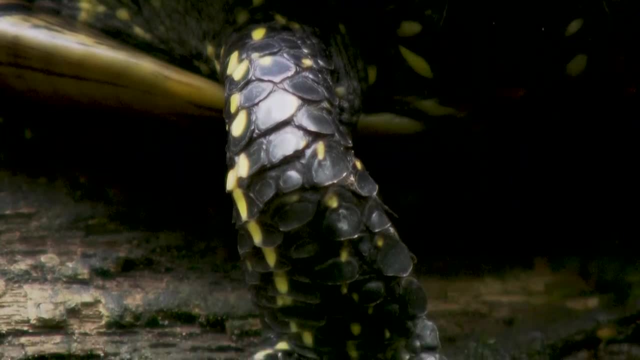 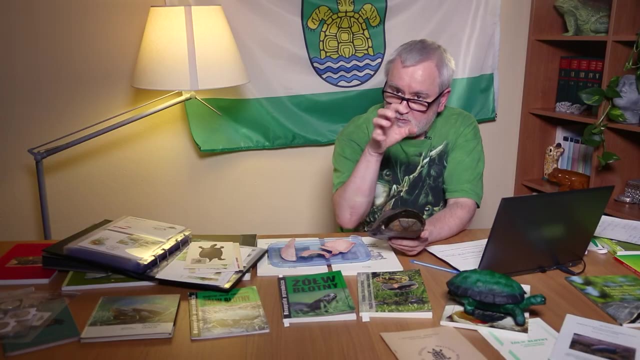 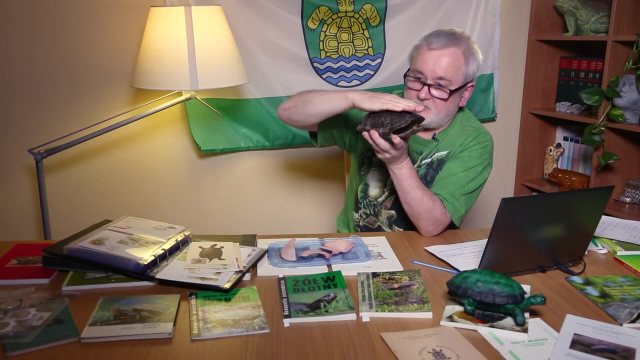 all the time. The male has longer claws because he gets on the female. This slight hole of his on the plastron does not allow him to fall and, in addition, it more or less looks like he is holding on tightly with these claws. These claws are. 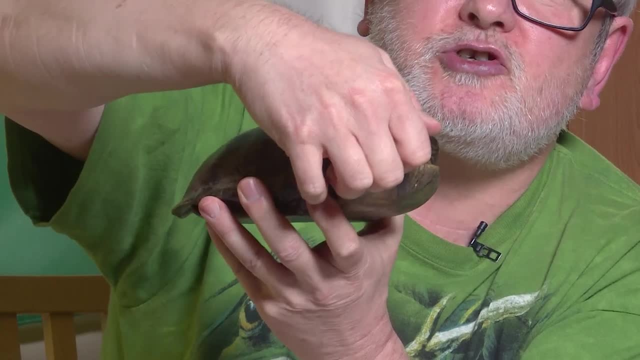 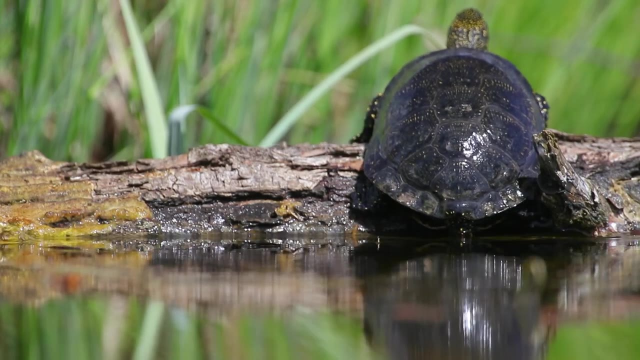 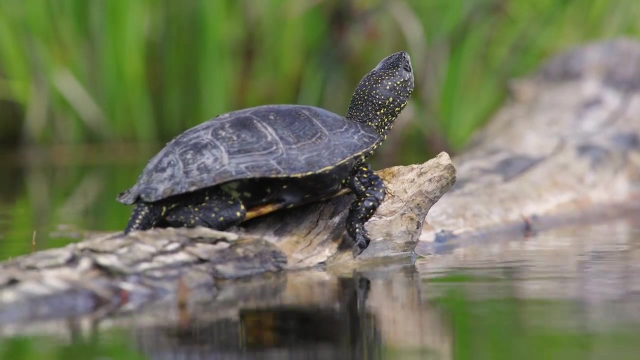 very important and actually I think they only serve to curve the claws themselves make copulation. The males during copulation are also helped by forelegs with digits ending in strong claws. The European pond turtle is a predator that hunts in water. The prey of adults consists. 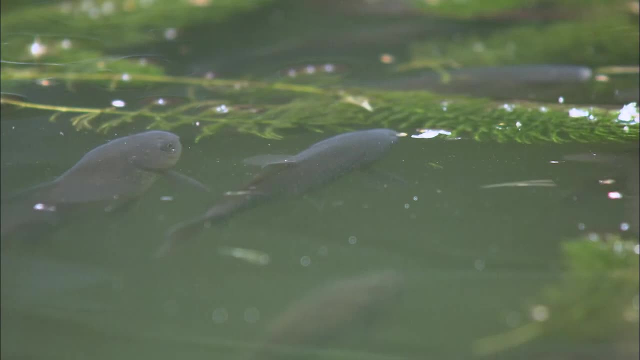 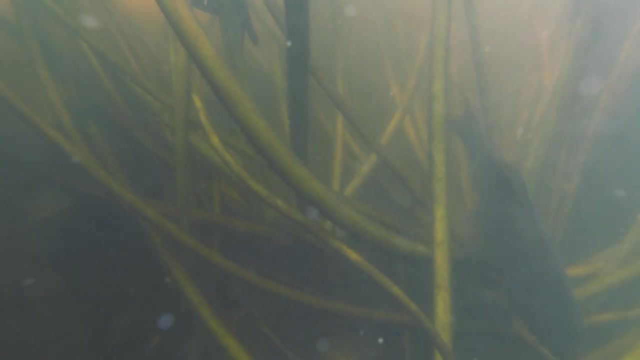 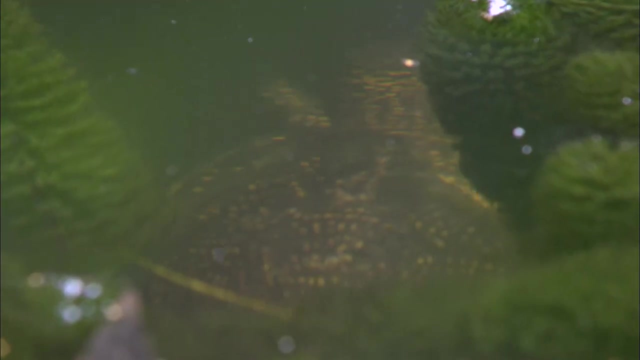 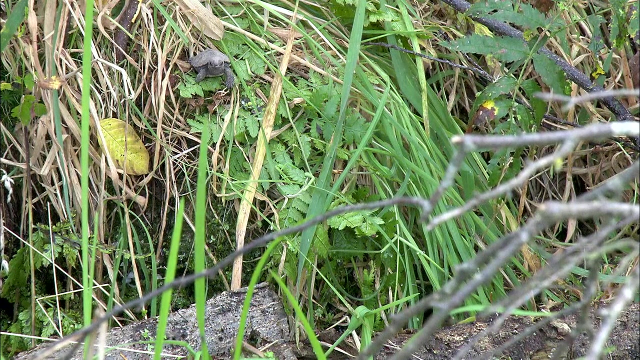 mainly of mollusks, larger insects and small fish, which they catch by suddenly throwing their heads forward. Prey is torn apart with claws and horned jaws. Turtles do not disdain carrion either. Young individuals feed primarily on insect larvae and small 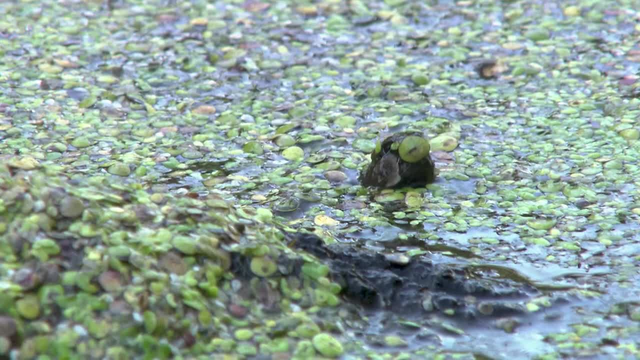 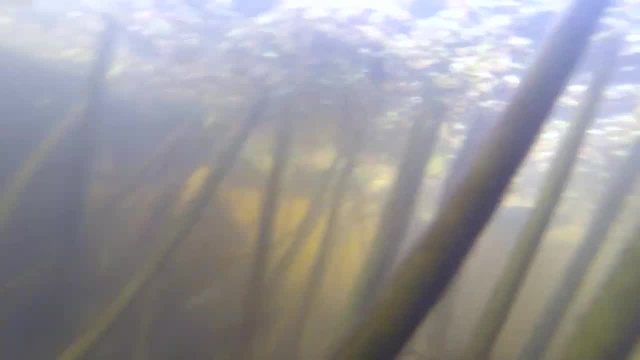 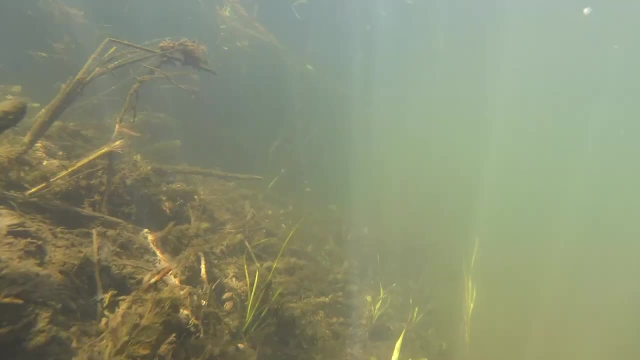 fish. Vegetative foods make up a small proportion of their diet. The European pond turtle is classified as a semi-aquatic animal. The European pond turtle is classified as a semi-aquatic animal that spends most of the year in water. The lungs help it to stay in an 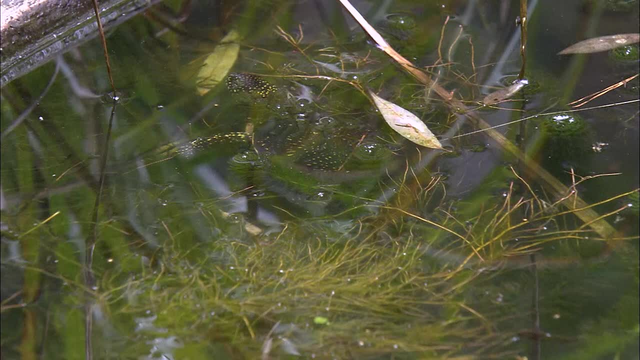 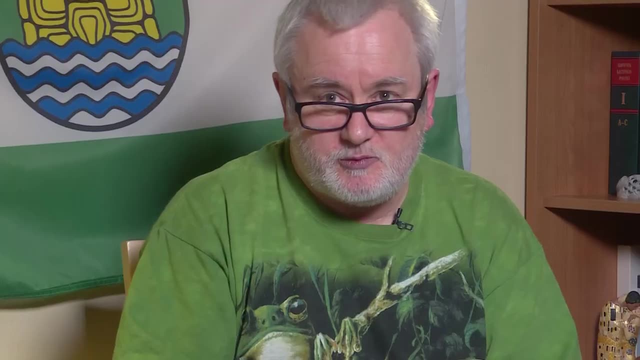 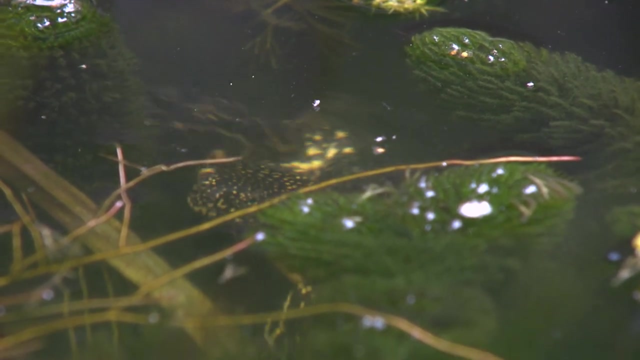 aquatic environment. They are an organ similar to the swim bladder in fish. Such an individual can remain underwater for as long as 40 or 50 minutes under the right conditions. Turtles are able to swim thanks to their digits, which are bound together by an inter-digital webbing, and their flattened and smooth 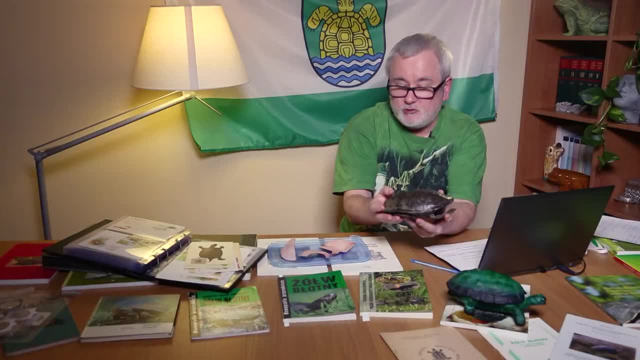 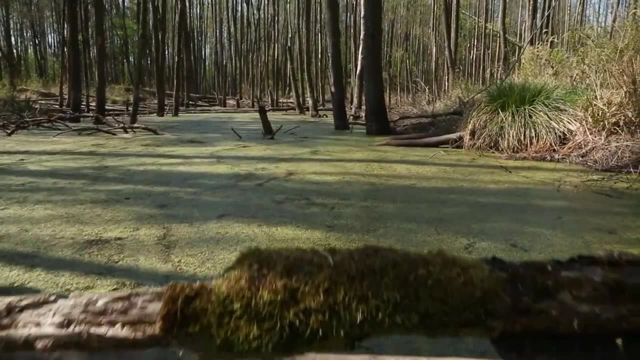 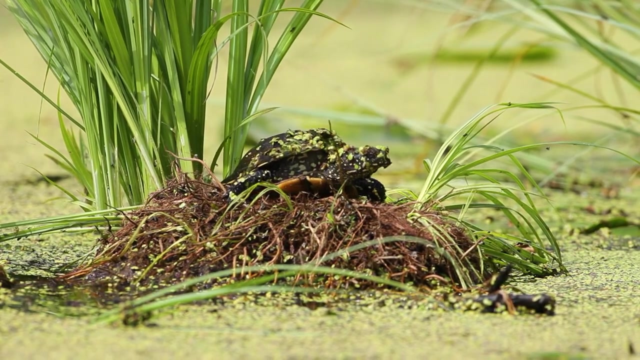 carapace. There are no outgrowths that would get in the way, because it often lives in swamps in alders where there are tree trunks and branches, and if something were to stick out here it would sneak under the water between these branches and it would constantly get snagged and have to retreat. 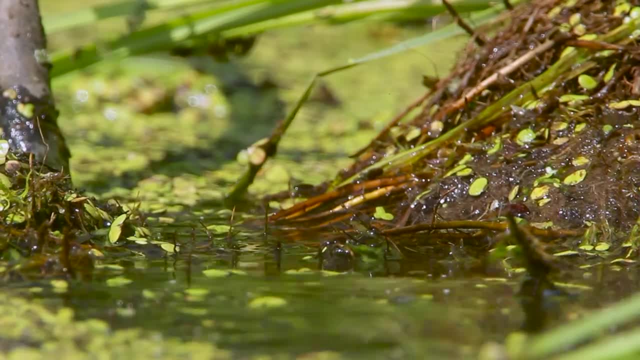 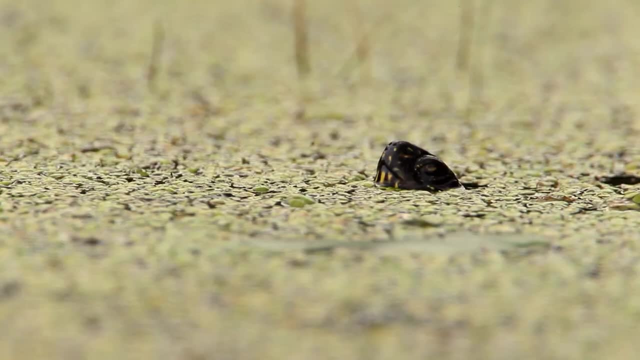 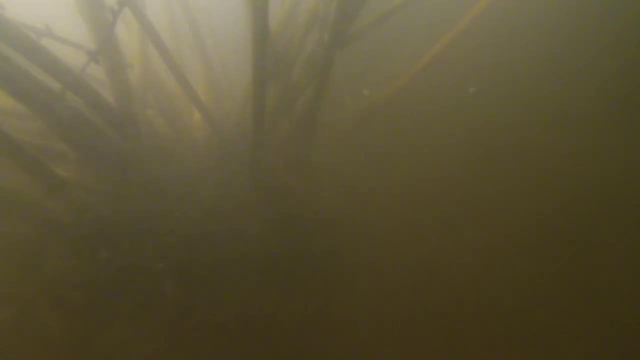 Its protective coloration, in the form of yellow spots, especially on its head and limbs, makes it almost invisible in its environment, especially in my home, the duckweed, The turtle, has a very well-developed sense of smell. It enables it to search for food in poorly clear water, as well as to identify the 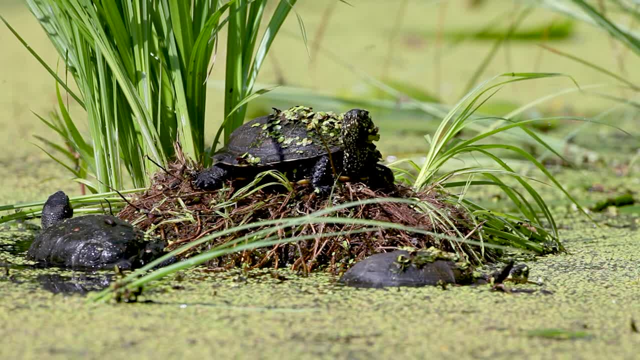 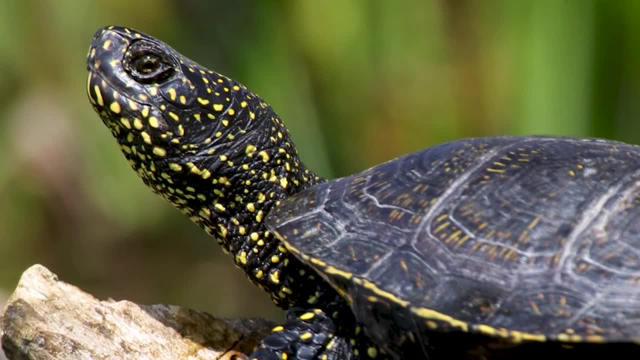 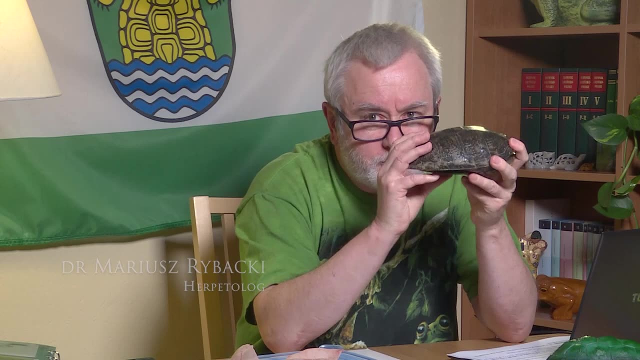 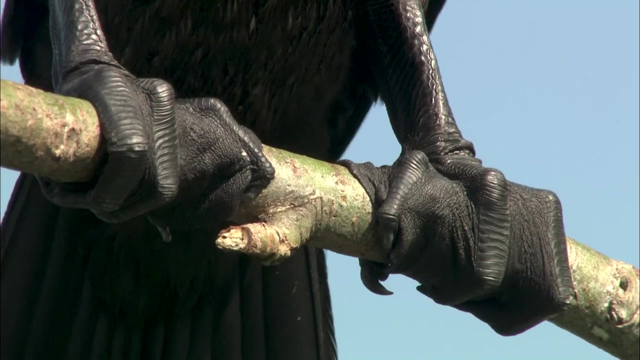 odorous substances secreted by the female during the mating season. The ability to see actually at various distances is as high as 40 diopters, so this indicator is very good. Of all the senses, sight is the best developed, Apart from the European pond turtle, the cormorant, the grass snake, the 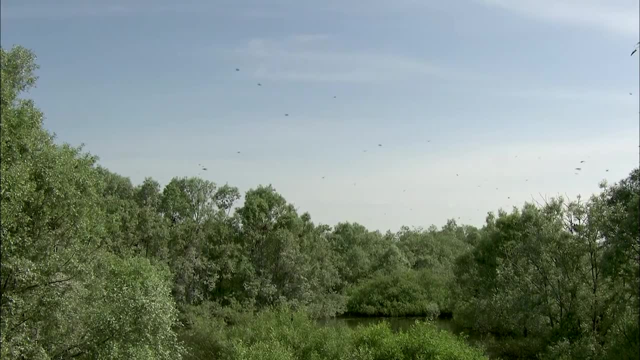 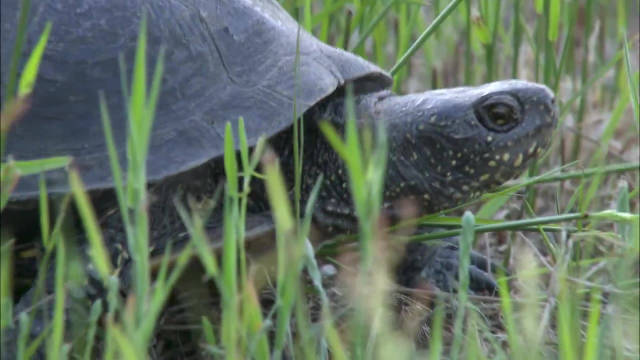 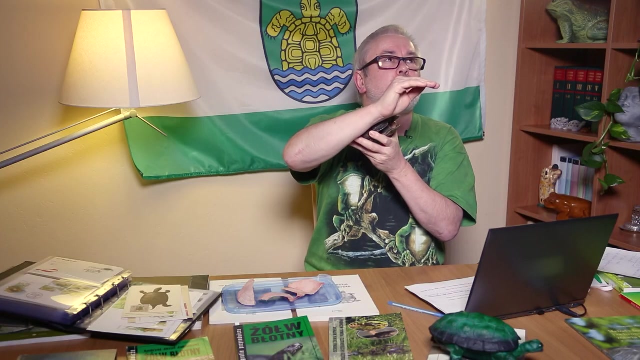 kingfisher and, to a lesser extent, the otter, are also endowed with such unique adaptations. The female: when she goes out looking for a breeding site, she holds her head up and it's like she's looking for those poles with temperature, With higher temperature, because that's an indicator. 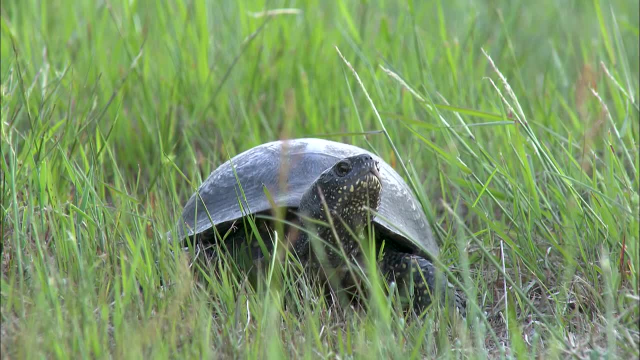 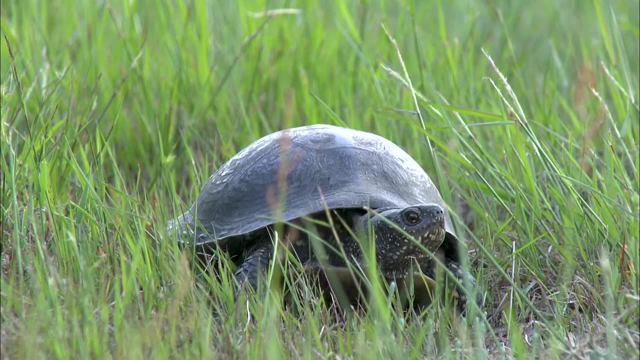 for them. Aha, the breeding ground is there Because, after all, these breeding sites and the surroundings of these sites are changing, Because some other vegetation or someone cut down a piece of forest, she's targeting these poles and that's, as far as infrared is concerned, the most important thing, right? 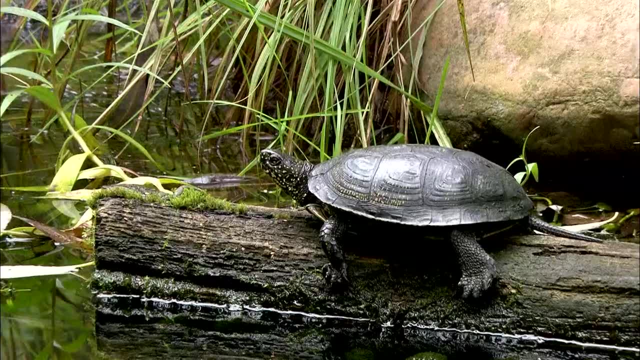 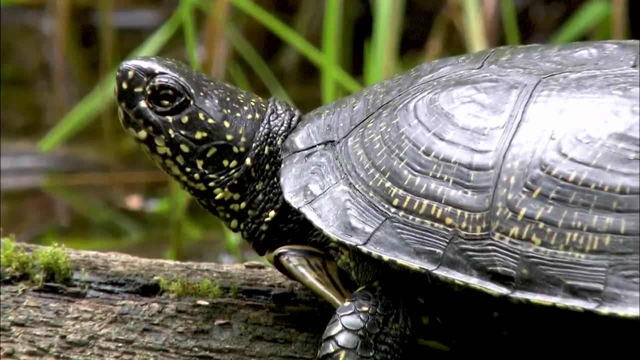 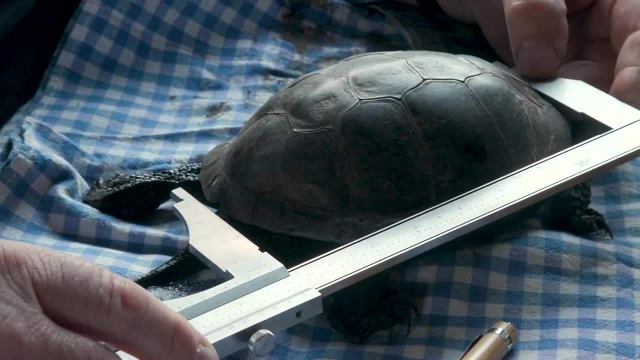 now in the reproductive success. If I can't find a breeding site, then my eggs won't develop. A very important feature, especially for females, is the ability to see in infrared. The nominate subspecies found in Poland is characterized by dark coloration and larger body size than the. 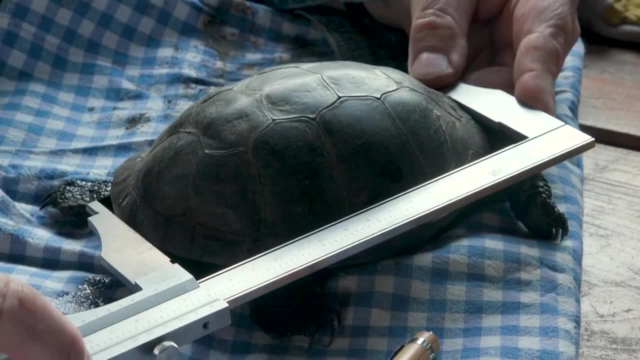 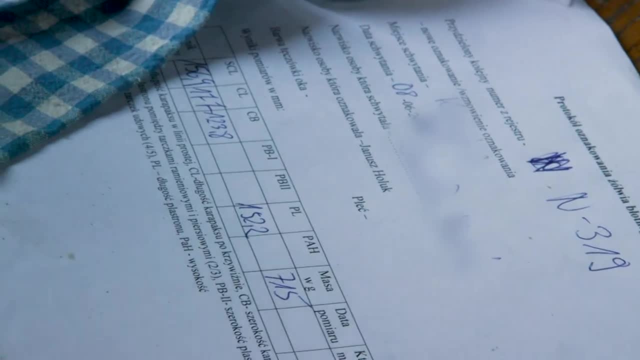 southern European subspecies. The length of the carapace, that is, the dorsal part of the shell, ranges from 14 to 18 centimeters in males and from 16 to 20 centimeters in females. Females are heavier than males. Their average body 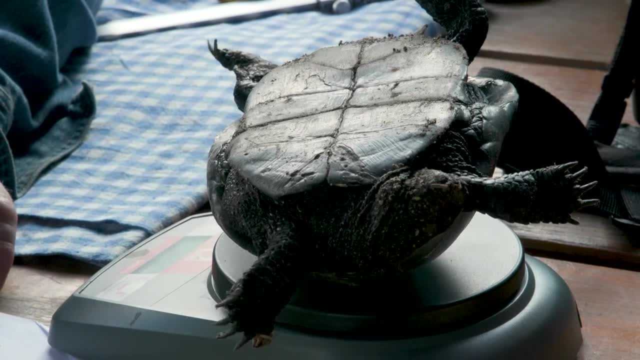 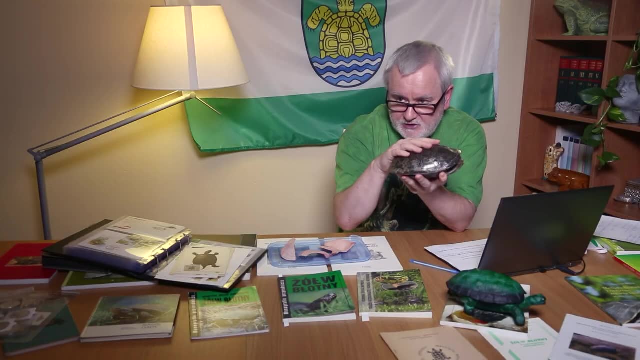 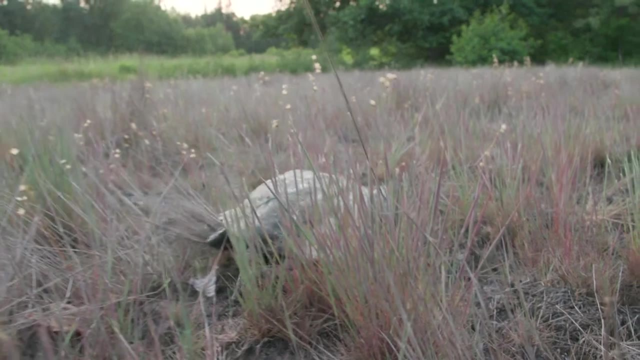 weight is about a kilogram. Males weigh, on average, 700 grams. The female has a carapace more arched that is higher than the male, because it is she who produces the eggs, She is the one who leaves her peaceful, dwelling in inverted commas, this swamp where rarely 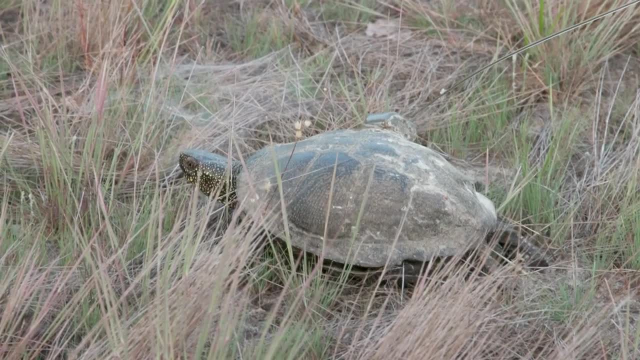 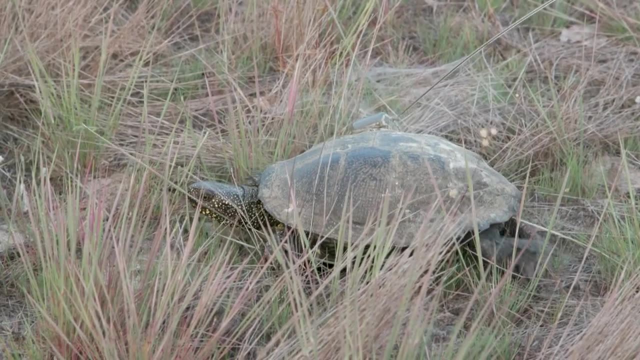 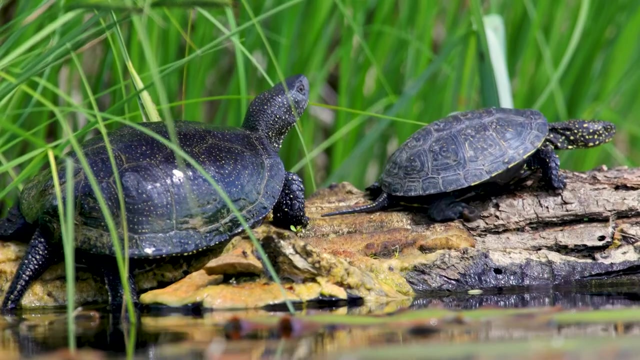 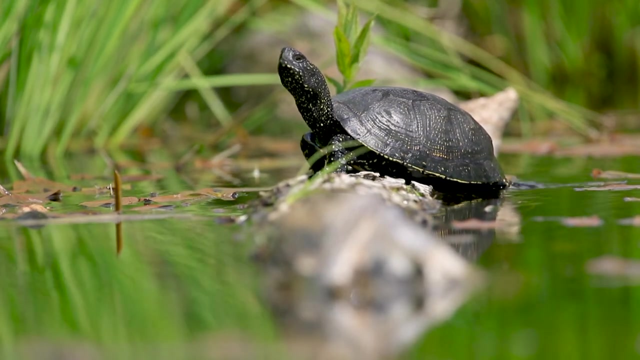 does anyone penetrate such a swamp and the male will stay there. The turtle has four legs that have five digits and hind legs with four digits. This reptile has contrasting coloration. The body coloration in one population can be very variable. The dorsal shell carapace is dark, brown, almost black and sometimes 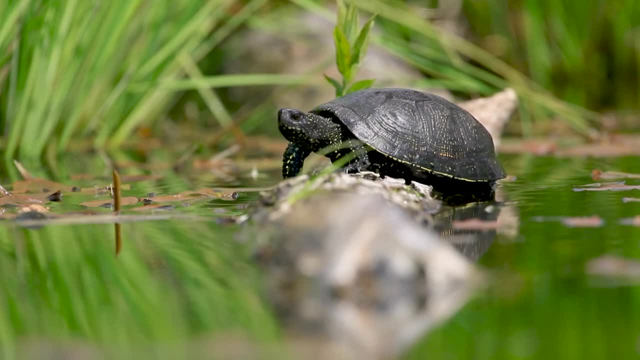 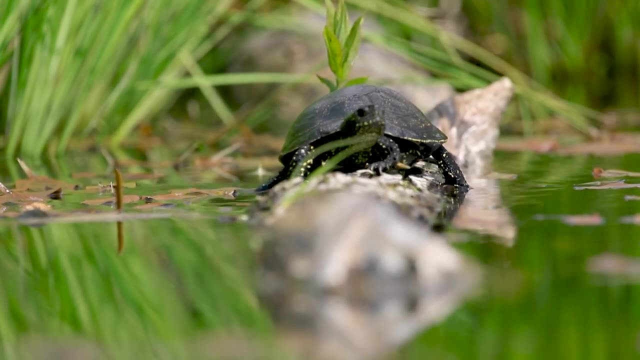 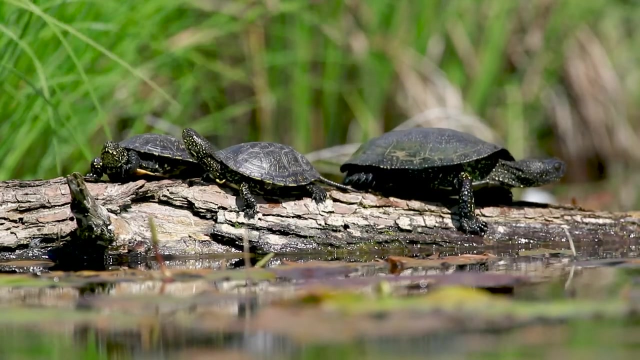 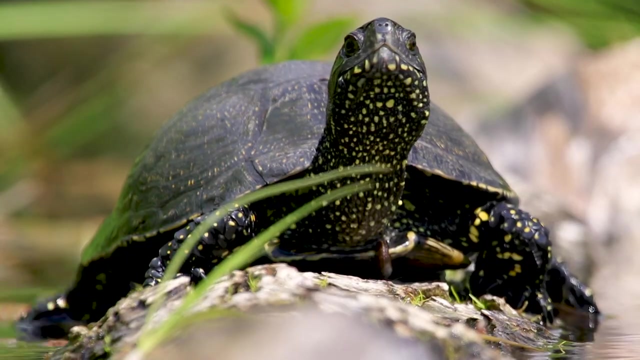 graphite black. On its surface there are often visible yellow spots in the shape of rays or radial lines on the shields. The abdominal shell plastron is, in males usually black or almost black. in females lighter or darker, with light spots. The dorsal and ventral shells are connected. 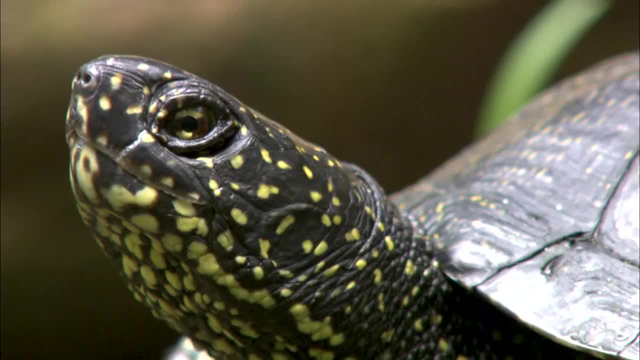 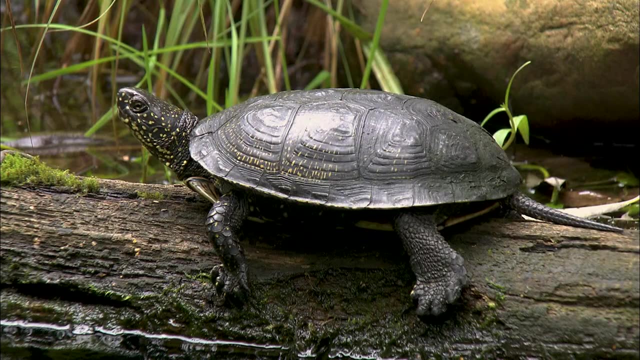 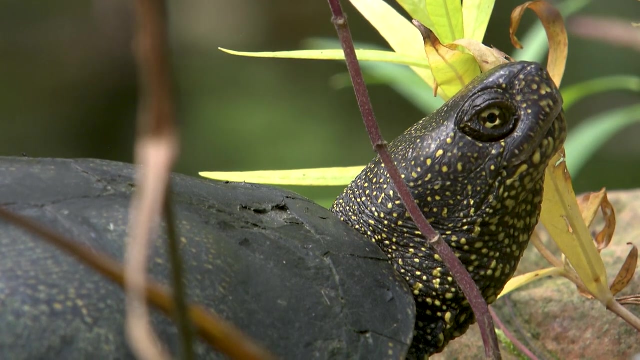 by an elastic bridge. The head, neck, paws and tail are black, with numerous small yellow spots. Females have far more of these spots, especially on the head and neck. The iris of the female and all sexually immature young is usually yellowish, while that of 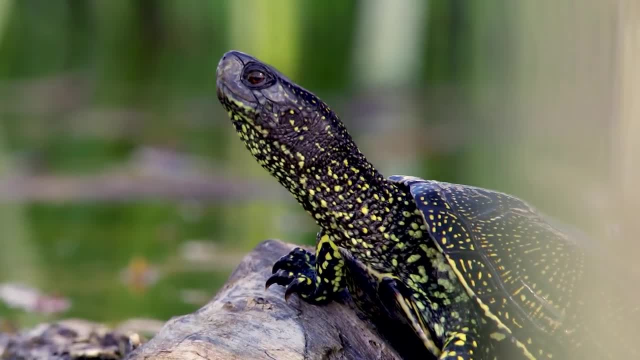 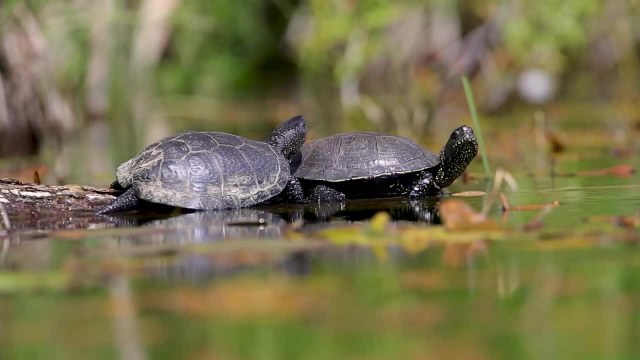 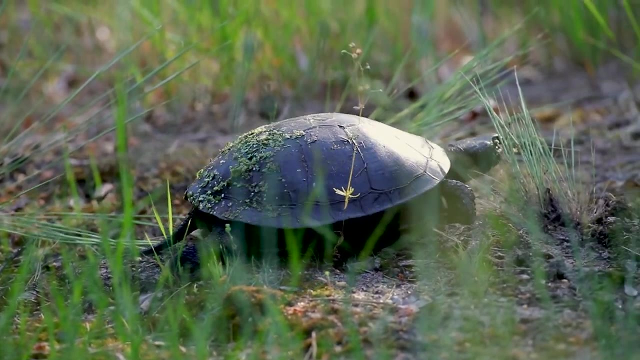 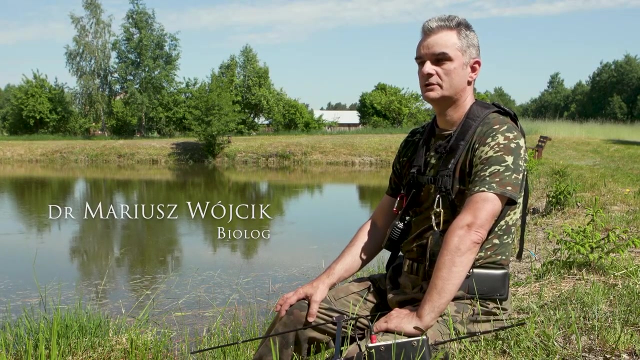 the male is orange or reddish-brown. The European pond turtle is a lowland species and its habitat is mainly water, which only the female leaves in order to survive. Its typical habitats are swamps, various wetlands. It is also a species that avoids contact with humans. 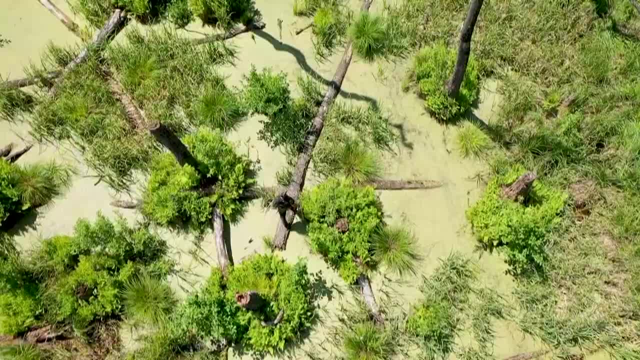 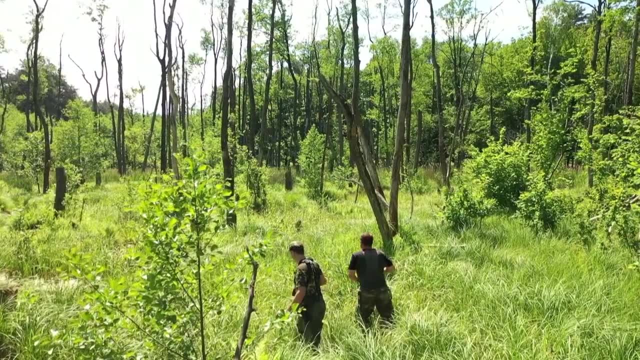 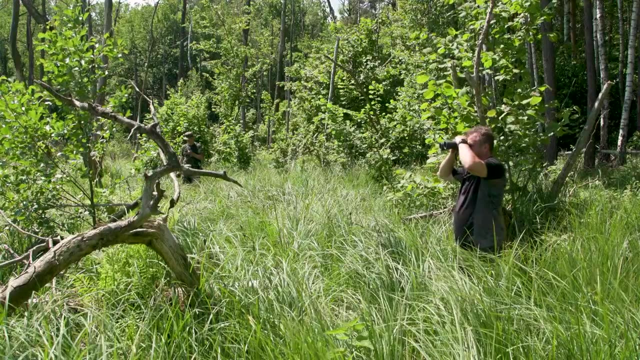 It is very vigilant and is usually difficult to spot and find in the field. The largest numbers of European pond turtle sites are located in shallow lake bays and mid-forest marshes. We are in one of the favorite habitat types for turtles. It is an alder which, as you can see, is dying. 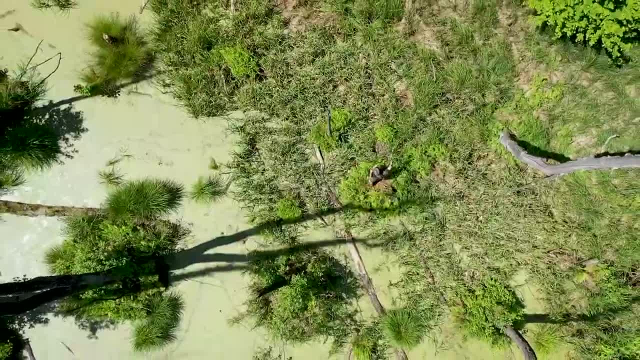 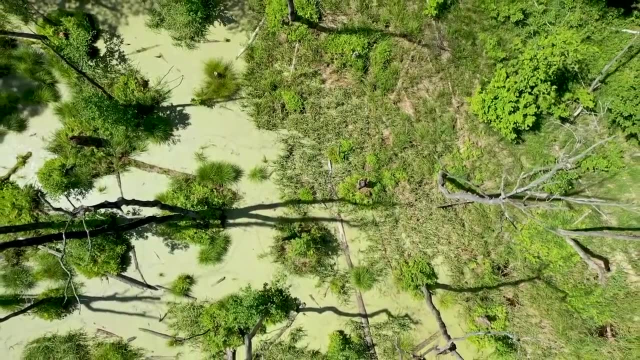 And it is dying because here I am standing on the ground. This is a beaver lodge. Beavers very often build dams which raise the water level, and then the alder trees die. This very natural area forms a kind of ring around it surrounds this pine overgrowth. 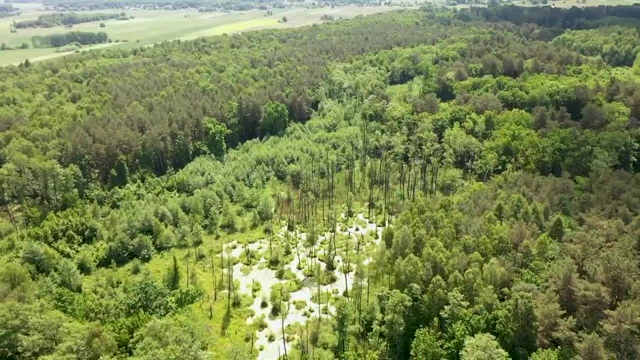 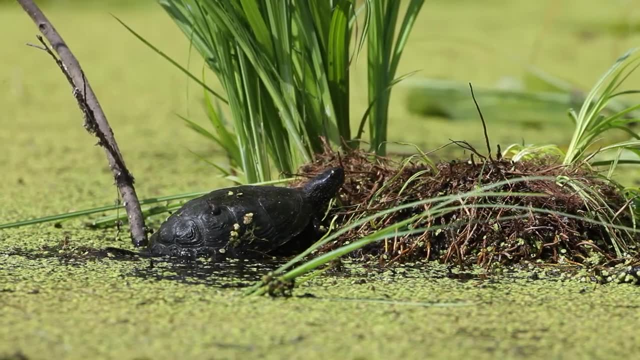 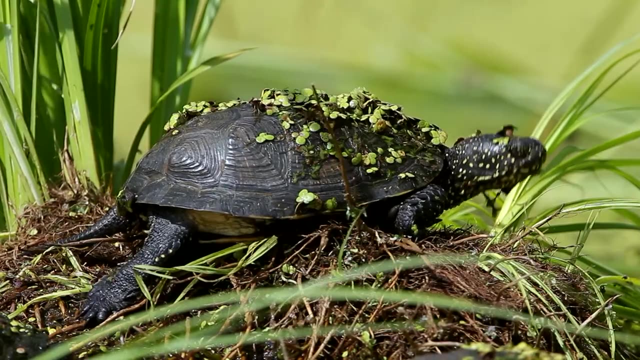 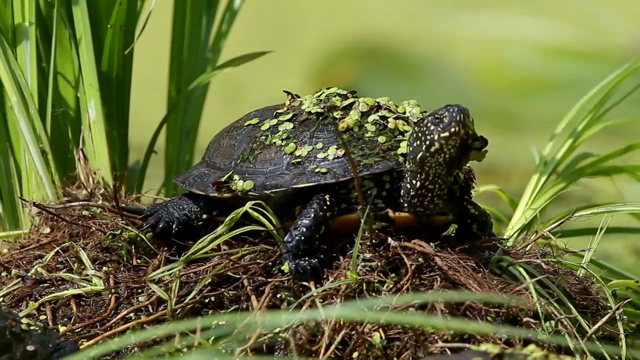 and in this habitat turtles are very often found, while right next to it there are artificial ponds where individual turtles also stay. Its location in the middle of the woods ensures the safety of these animals, And the presence of forest clearings provides the necessary breeding sites. 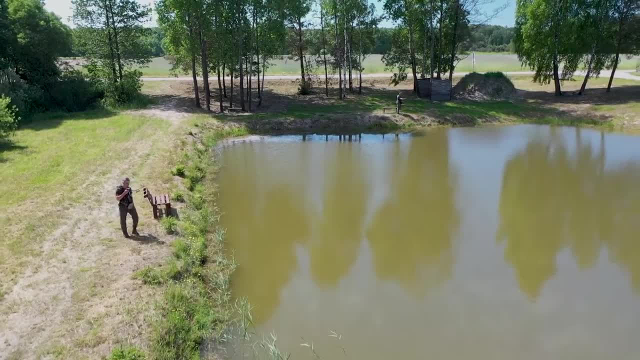 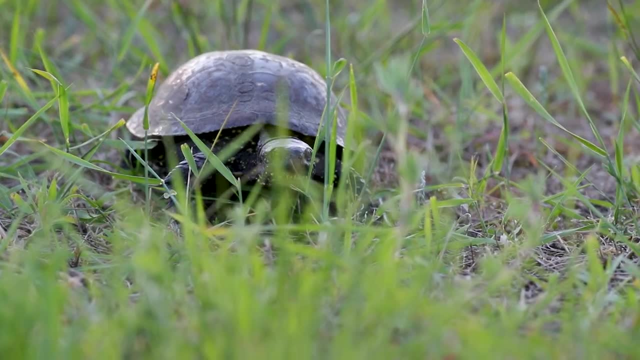 Stopover for turtles that are typically found on the other side of this pond in the marshes. This over here is a female. They come just before the breeding season to go out near evening, dig a hole and lay their eggs there. Young turtles prefer a slightly different environment than older turtles. 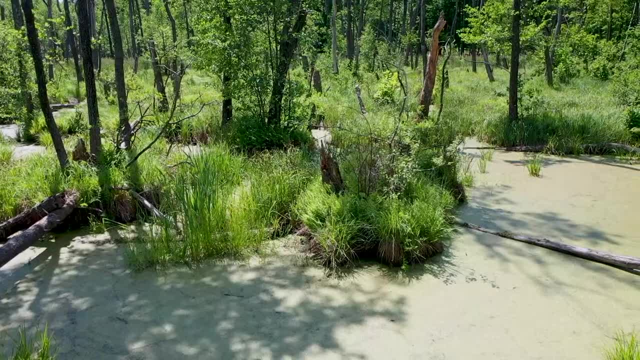 This is a female. They come just before the breeding season to go out near evening, dig a hole and lay their eggs there. This is a male. They give birth to 3 kittens. They are very active. For safety reasons they prefer wet alder swamps and small ditches and streams. 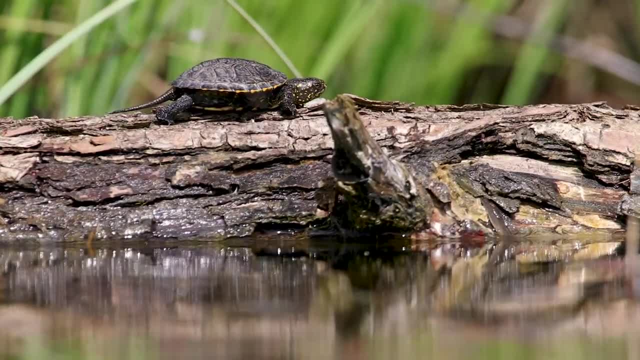 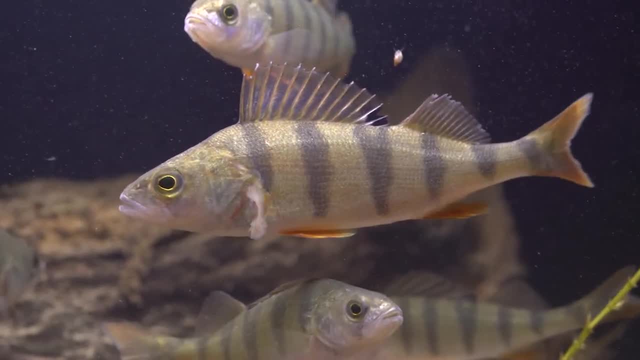 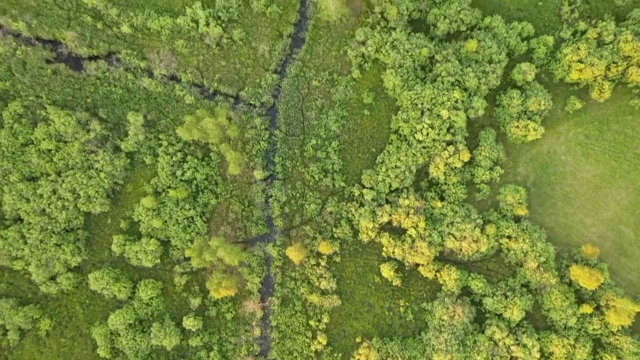 They find more hiding places there, and the lack of open and deep water protects them from attacks by predatory fish. Watercourses are also important migration routes for these animals. The turtle is, of course, considered to be a symbol of slowness, but it was able to move. 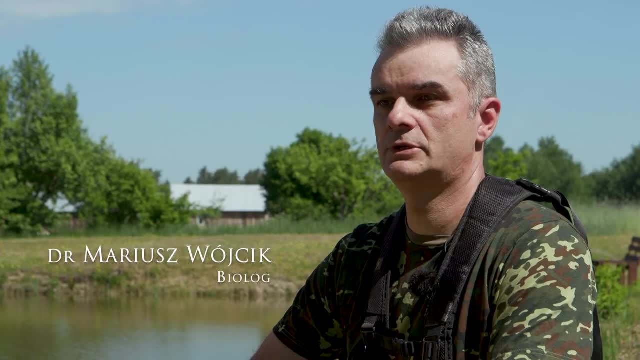 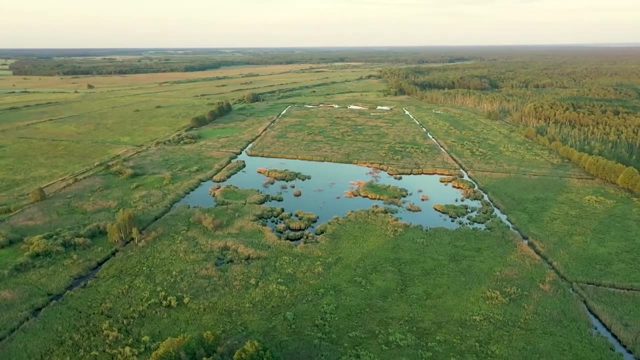 quite efficiently. They use the facilities that we know best we humans have made for them, that is, there is a series of drainage, ditches and turtles can move up to several hundred meters a day. Usually such movement takes place in spring, when the 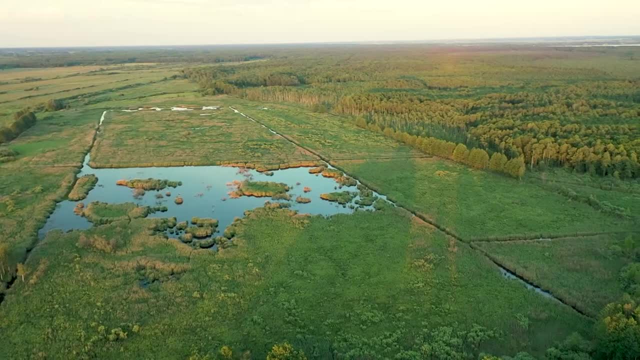 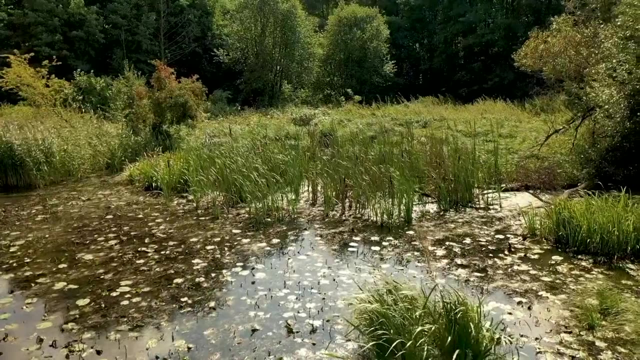 males are looking for females. The second moment is when the females come to their breeding grounds. Most reservoirs and watercourses in which European pond turtles live are of a eutrophic nature. They are usually shallow, with a thick layer of bottom sediment. 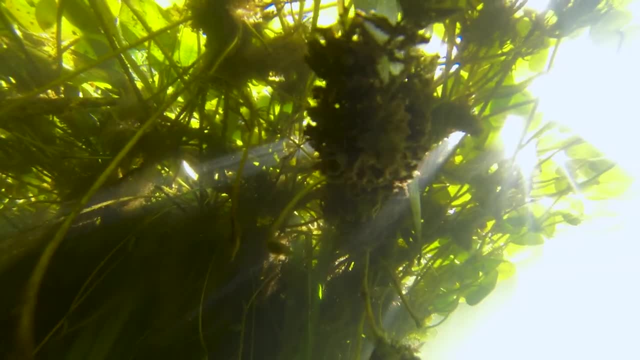 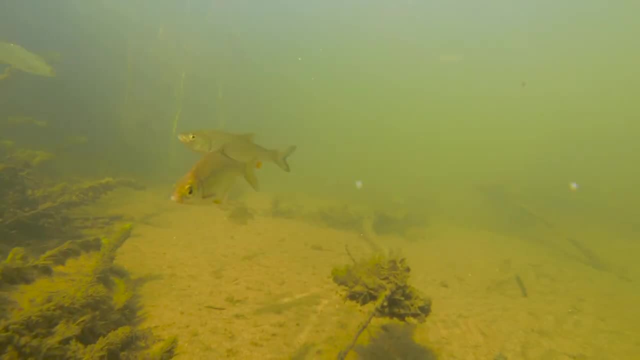 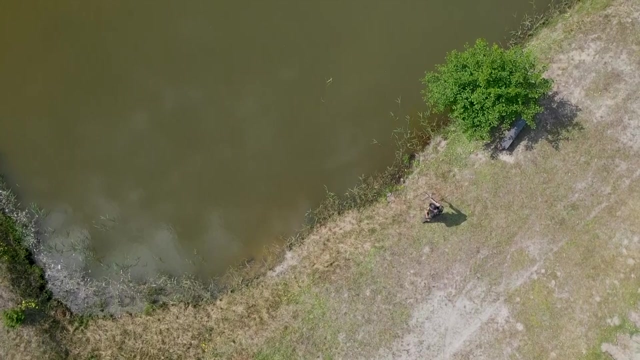 well-developed coastal vegetation and muddy banks. Such places heat up quickly and are abundant in food. Turtles can also be found in artificial reservoirs such as fish ponds, clay pits and other post-production reservoirs. They are just as likely to inhabit small rivers with calm currents, canals and even drainage. 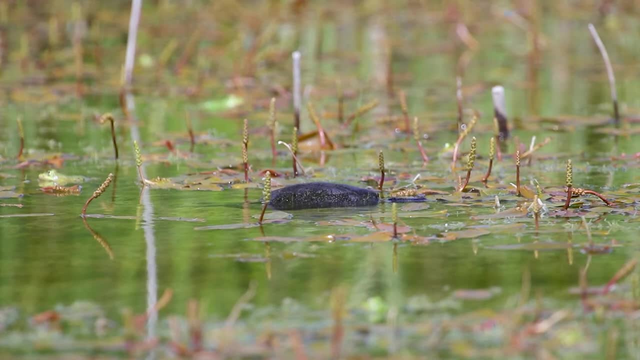 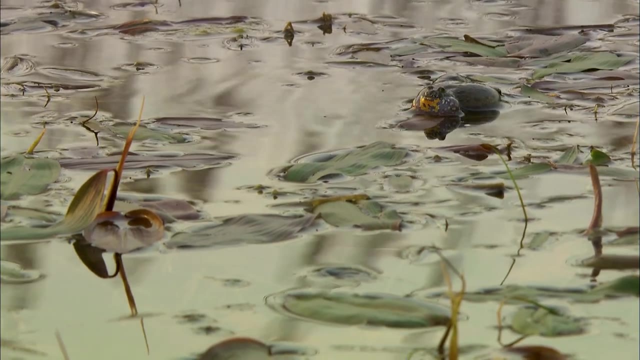 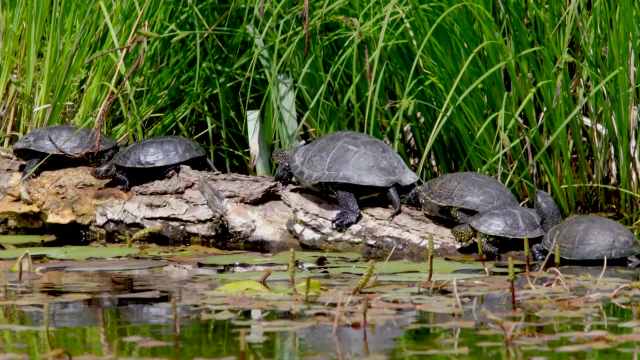 ditches, which are important migration routes for these animals. Sometimes the places where turtles are found are far from what we imagine an ideal turtle habitat to be. Sometimes they inhabit very polluted and degraded reservoirs. The turtle is often referred to as a shield or umbrella species. This means that, by protecting 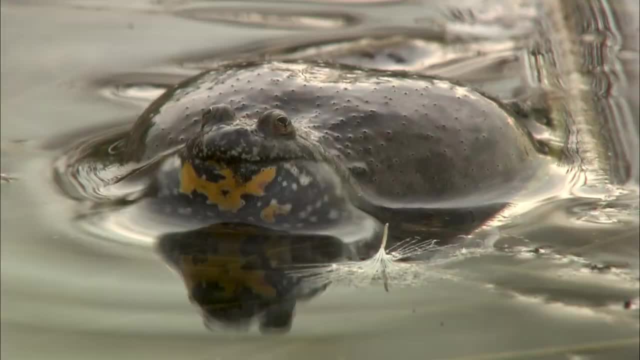 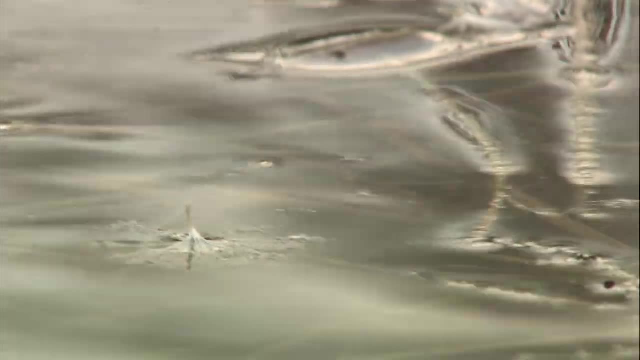 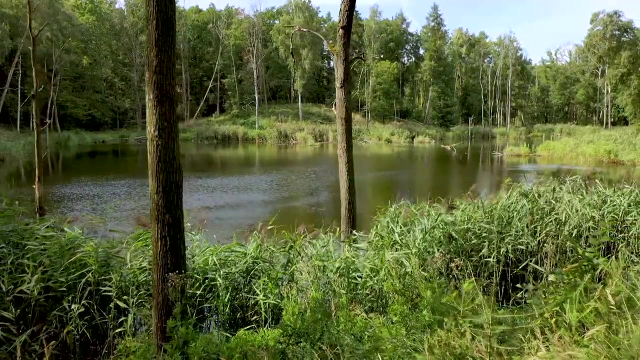 turtle habitats we protect the biotopes of many other animal and plant species that are often threatened with extinction. For several decades, turtles from North America have been a serious threat to the European pond turtle. Turtles from North America have been a serious threat to the European pond turtle. 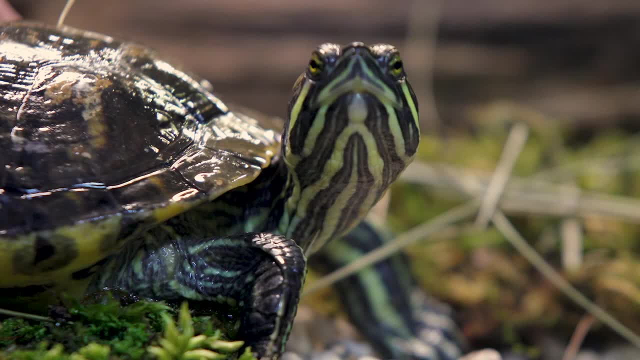 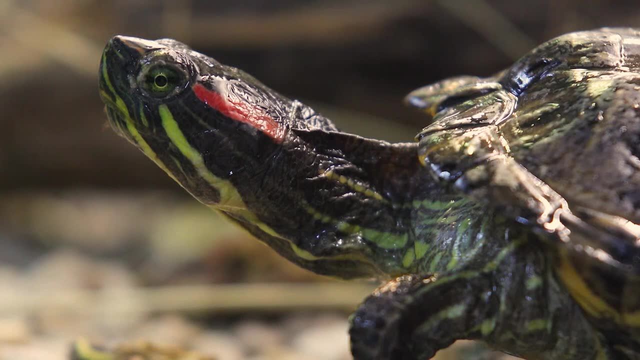 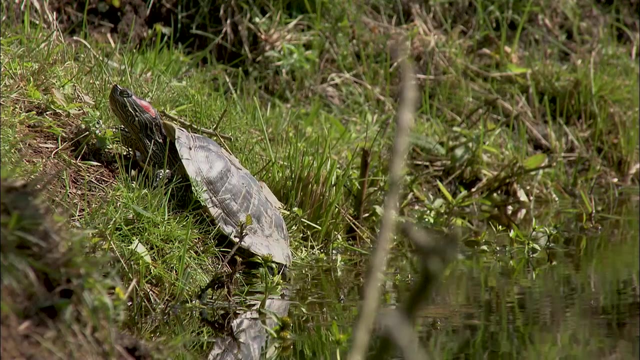 Turtles from North America have been a serious threat to the European pond turtle. They belong to a group of ornamental turtles and the red-eared slider turtle, which has been classified as one of the most invasive alien species worldwide. It arrived in Poland as early as the 1960s. In the 1990s there was a huge 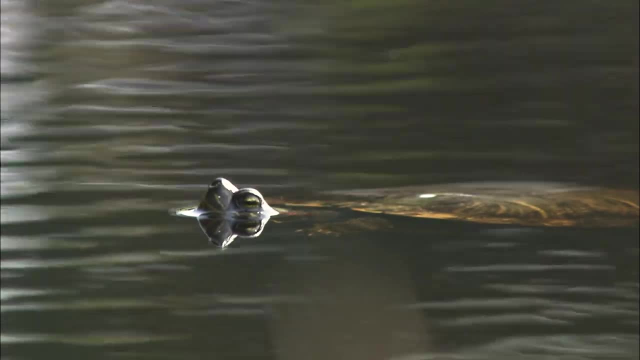 increase in its numbers when nearly 450,000 individuals arrived in our country. Turtles from North America have been a serious threat to the European pond turtle. Turtles from North America have been a serious threat to the European pond turtle. They belong to a group of ornamental turtles and the red-eared slider turtle. 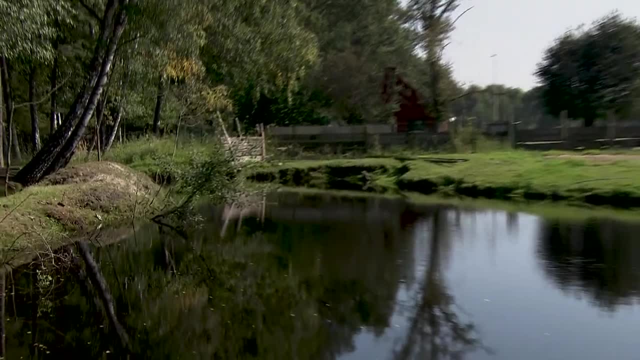 Currently ornamental turtles are found. They belong to a group of ornamental turtles, and the red-eared slider turtle Turtles from North America have been a serious threat to the European pond turtle in almost all over Poland, except for the northeastern part of the country. 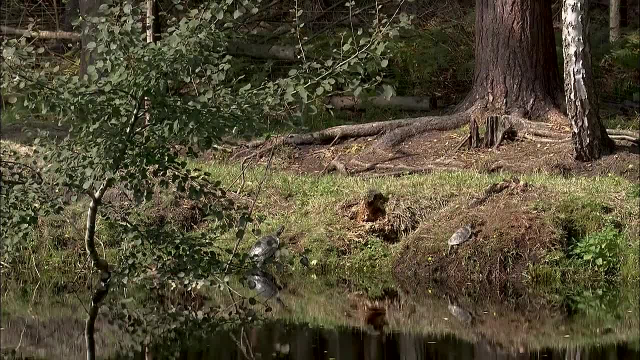 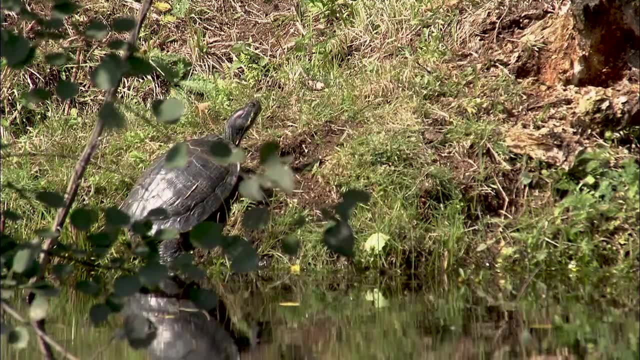 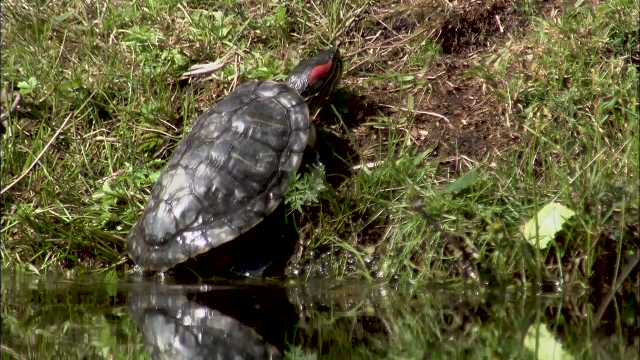 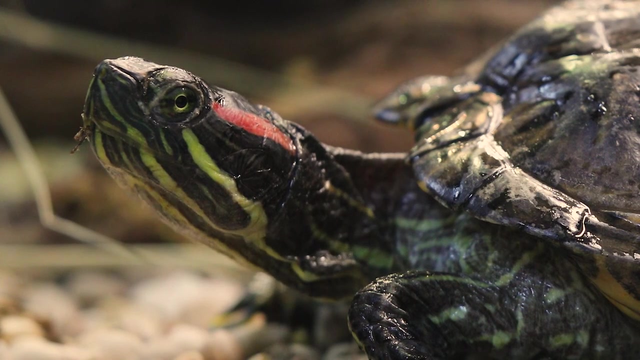 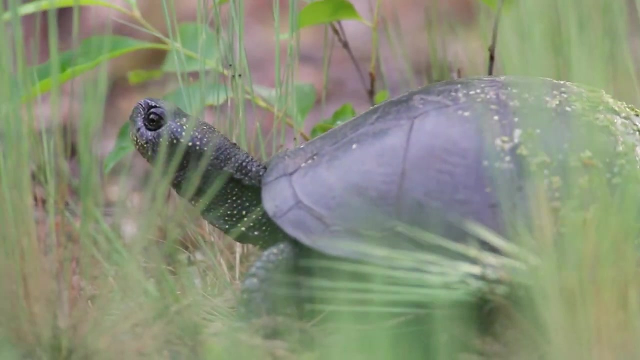 Turtles from both owners hunting Dinosaurs with Fer cuisine deer hunting European sea Darwish carry dangerous parasites, including nematodes and bacteria. They can also carry salmonella, which carries a risk of infecting humans with this bacteria In northern and central Europe. the European pond turtle is now a very rare animal and has 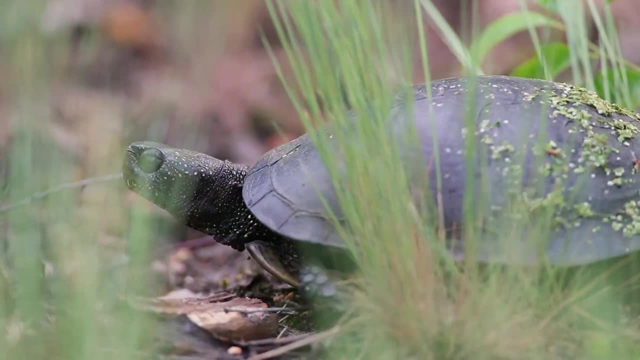 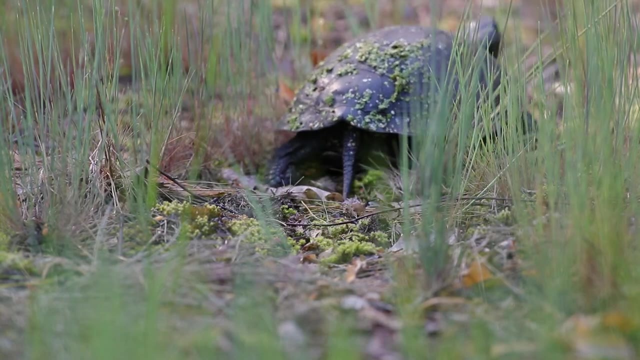 been included in the red list of threatened animals. in many countries, The main reason for the disappearance of this species was humans, who have destroyed its populations and habitats for hundreds of years. In many regions of Europe, it was caught en masse for culinary purposes. 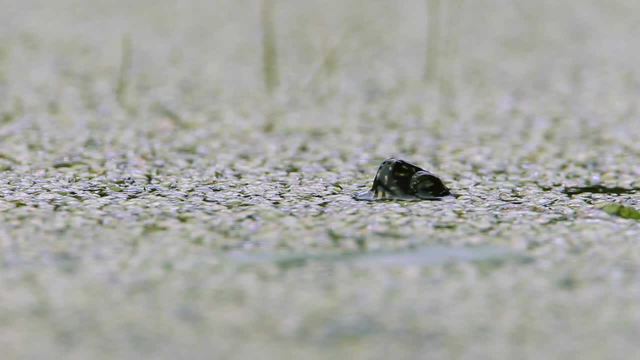 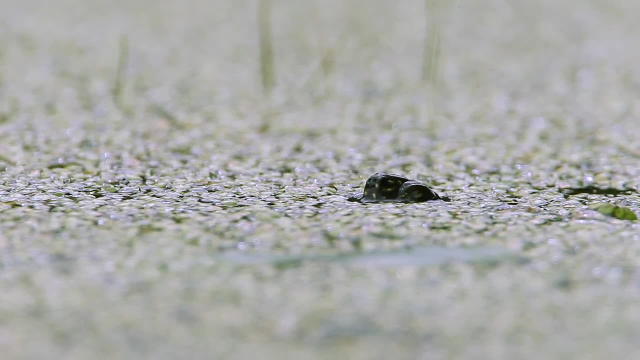 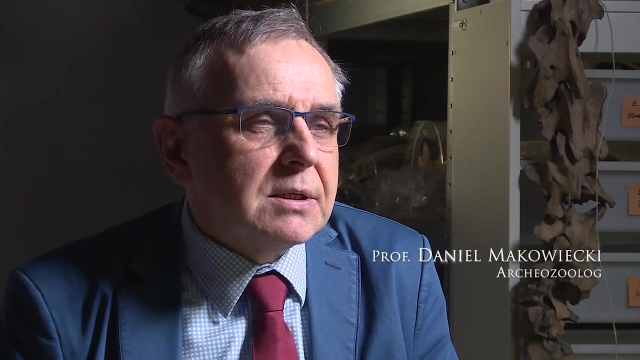 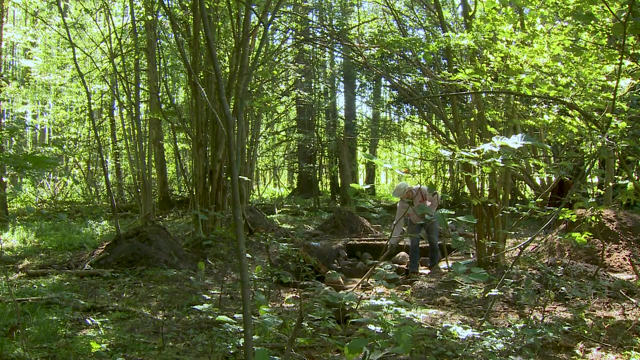 Looking at this oldest history of the turtle through the prism of finding its remains. as archaeologists, we most often find it in places that were once inhabited by humans. So if these are such places, we wonder why this animal, this vertebrate, this reptile? 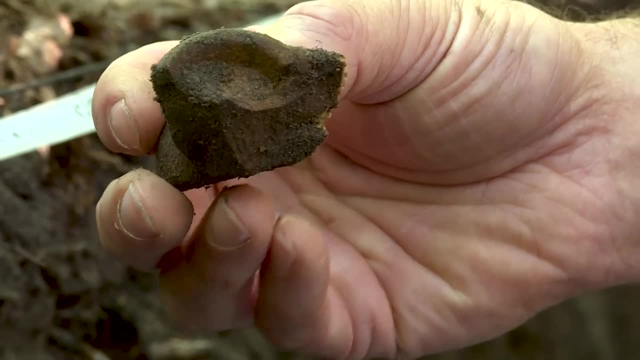 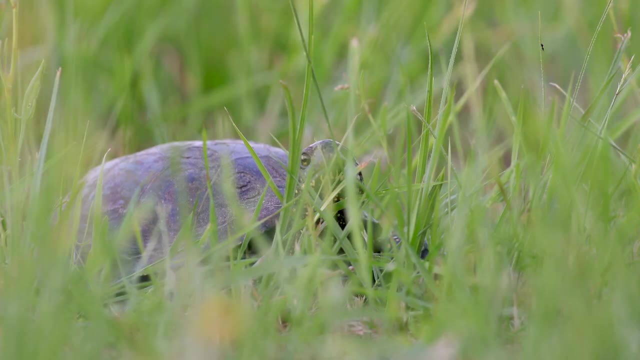 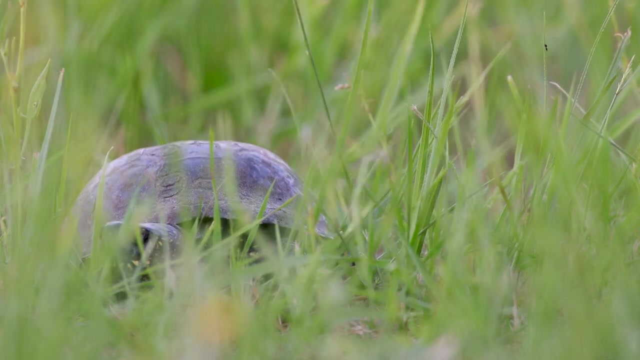 found itself in this place, We can, on the basis of our various indications, this archaeological context, that is, the environment in which these turtle remains were found, assign three types or three modes of human use and interest in the turtle. The first is a very prosaic one, because it is related to food. 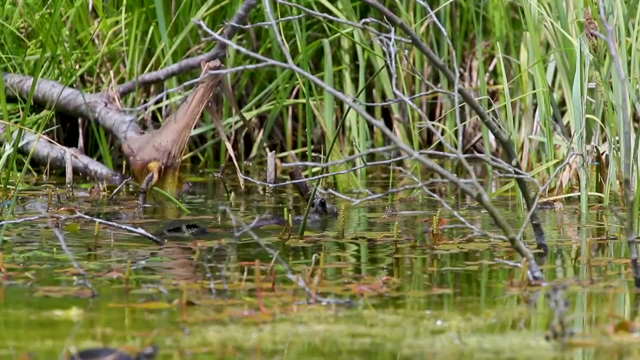 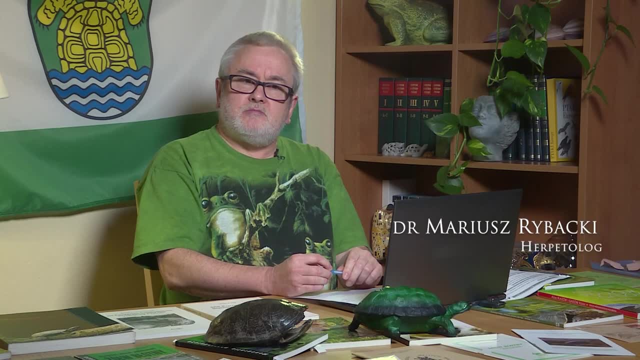 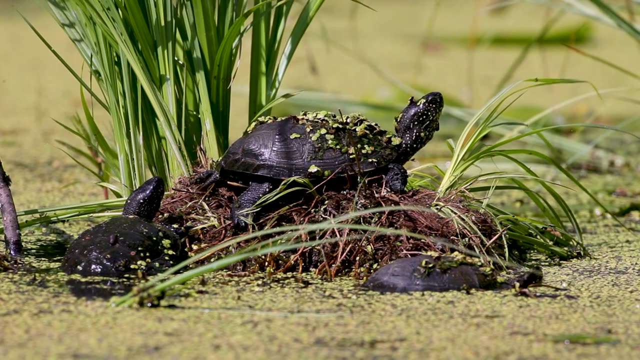 To simplify matters, the turtle was considered a fish in the eighteenth century, whether in Germany or Poland, in fact all over Europe. Because it was a fish in inverted commas. the fish were eaten during fasting. So for example in Mecklenburg in one year about four and a half thousand turtles were caught. 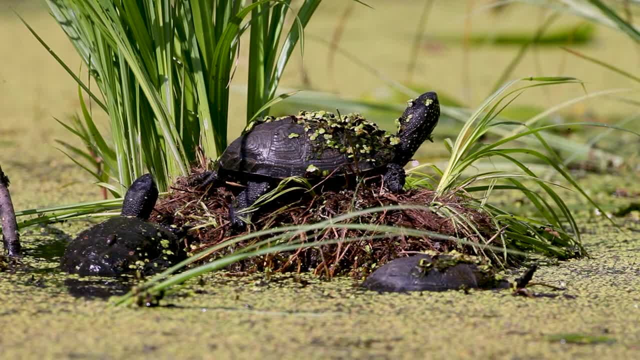 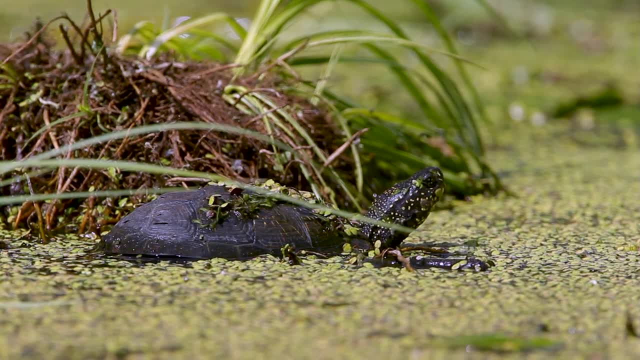 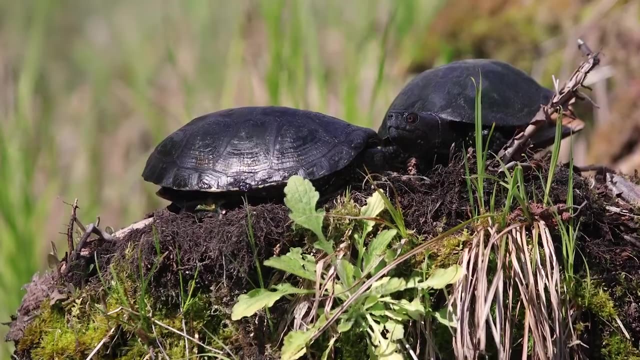 to be sold in Berlin because there was the biggest market there, which meant huge quantities. Now it is estimated that there may be two, some say two, maybe three thousand. in Poland, One year there was 4,500 turtles. We have no doubt that the European Pond Turtle was an animal that was caught when it laid. 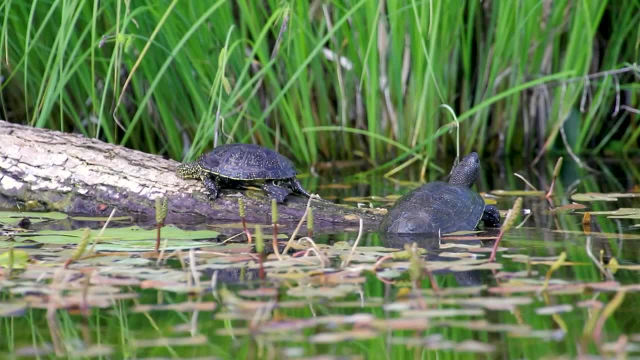 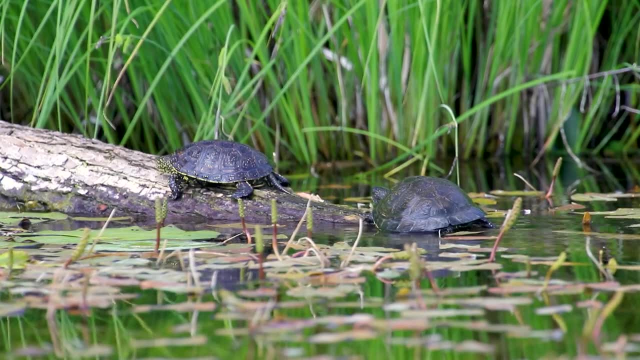 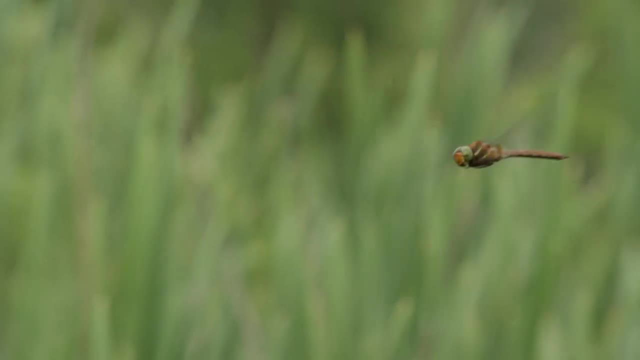 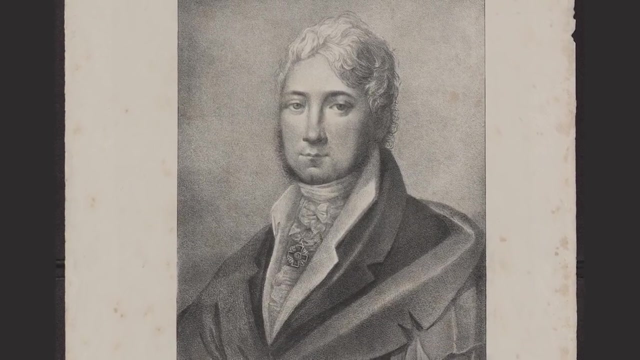 its eggs in the land zone and was caught when there was fishing and when there was a shortage of food, when it was spring, when the whole world was just coming to life and man obviously needed this food. Ludwig Bojanus, a German who worked at Vilnius University, wrote his famous work Anatomy. 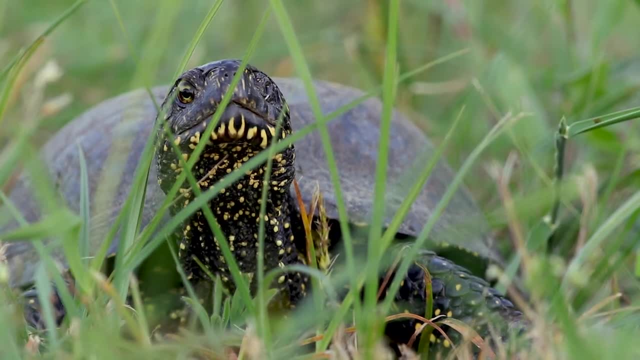 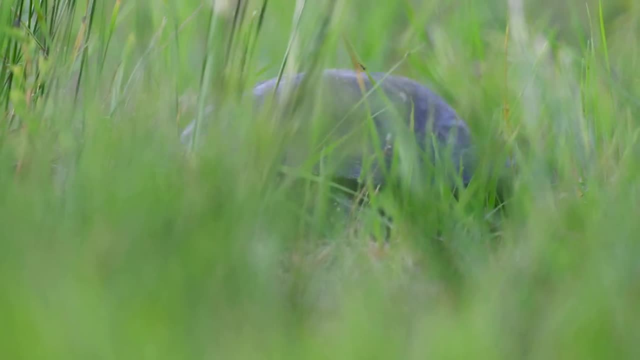 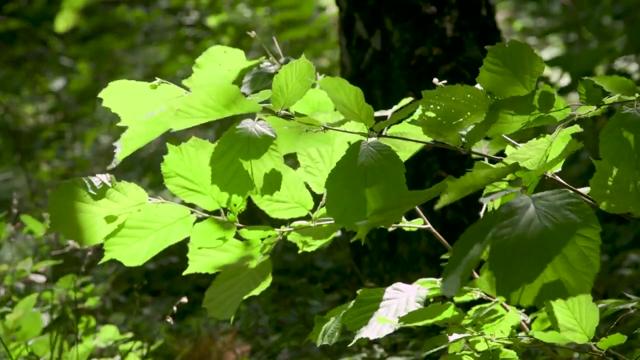 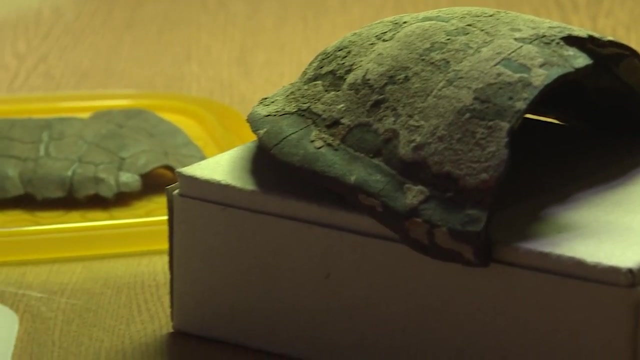 of the European Turtle For this work. he used more than 500 adult turtles, mostly brought from Polesie. The 500 turtles went under the scientist's knife. His work is still eternal, but what a loss in population. We have also found turtle remains that allow us to believe that the turtle had another. 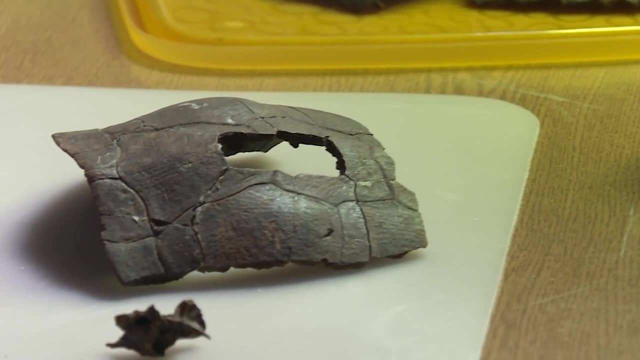 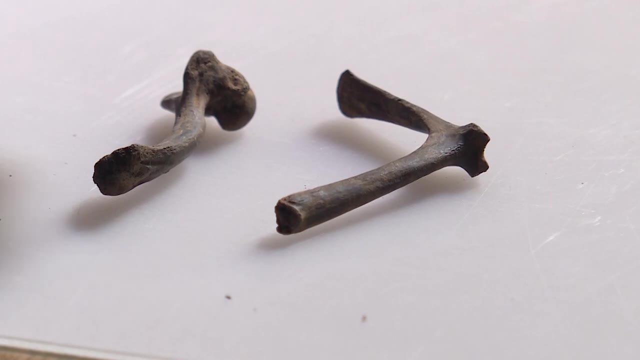 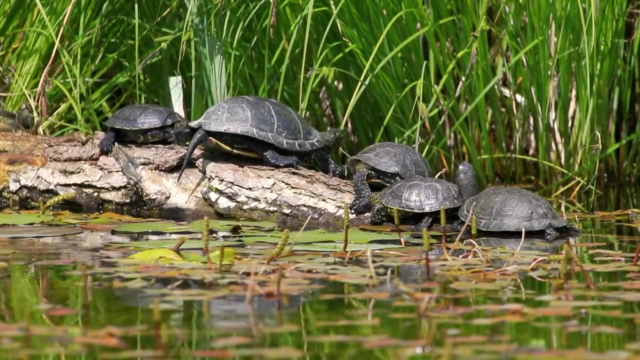 function, a function in beliefs, a magical demonstration of a connection to a world other than our own. This magical function does not preclude treating the turtle as a pet, an animal for company, an animal that probably aroused curiosity and interest. Turtles were sometimes bred for entertainment. 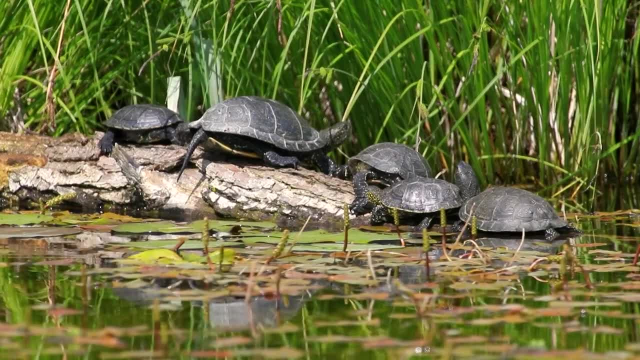 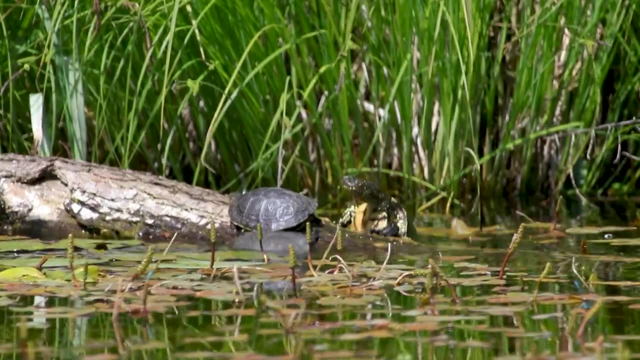 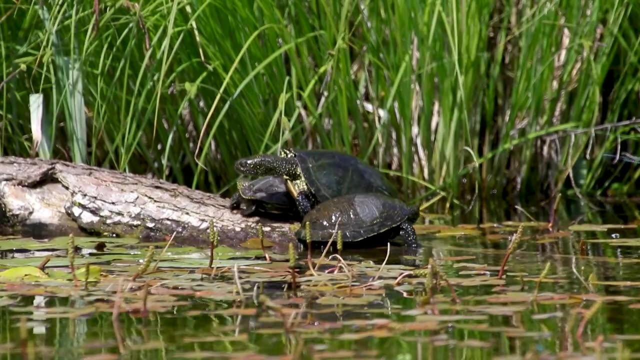 For example, the Missourians sold turtles in Konigsberg in the 18th century Inns. innkeepers bought them, kept them in a container of some sort and when someone came to drink beer or wine they could touch the turtle or look at it. 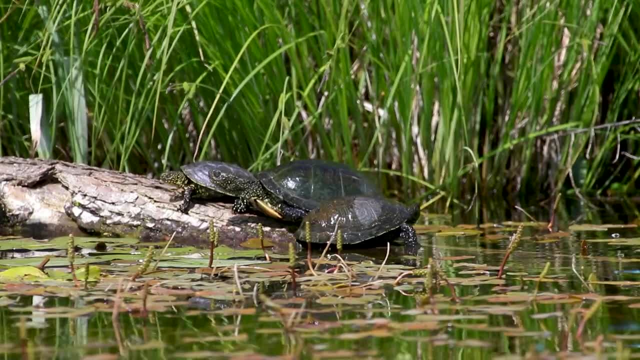 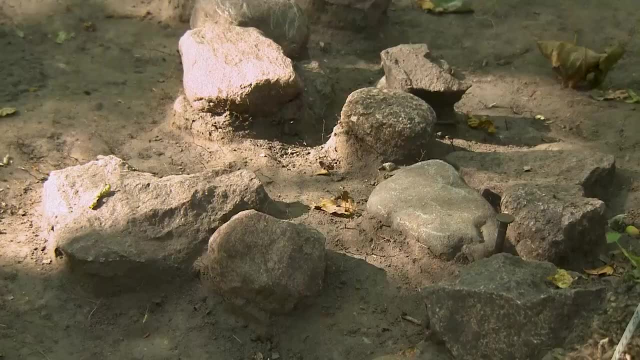 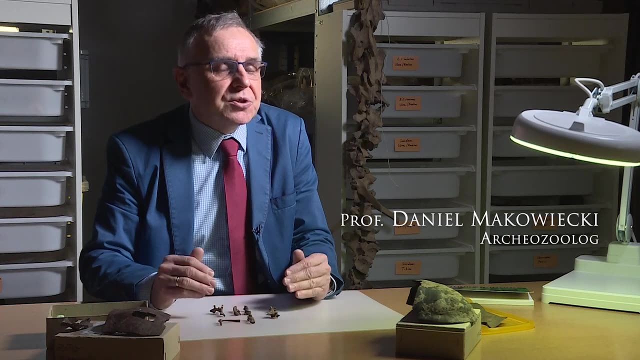 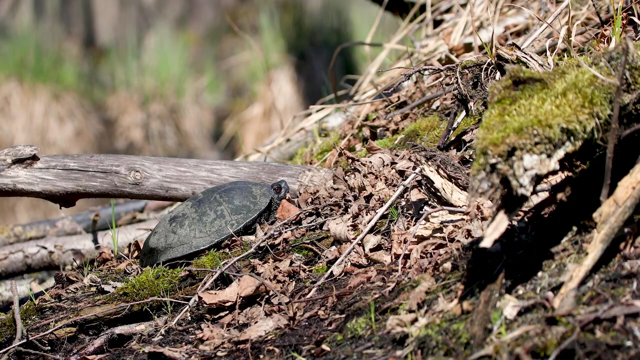 What evidence is there for this? The presence of turtle remains, including carapaces and skeletons in human graves, be they children or adults. So these three functions of the turtle, the triple significance we can attribute to it, And when we can also think that it was an animal which, due to its appearance, was quite 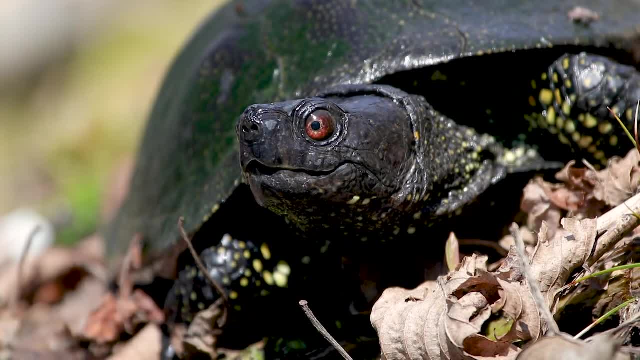 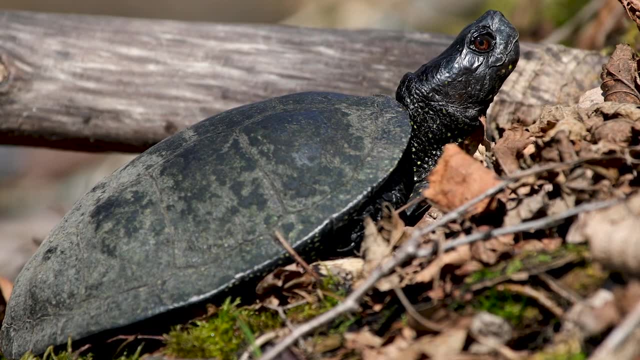 mysterious and was perceived as such. and what is mysterious and in the end, not as common as other animals, caused such interest. Hence the emotional function attributed here to the turtle. So we can attribute to it the triple significance. So we can attribute to it the triple significance. 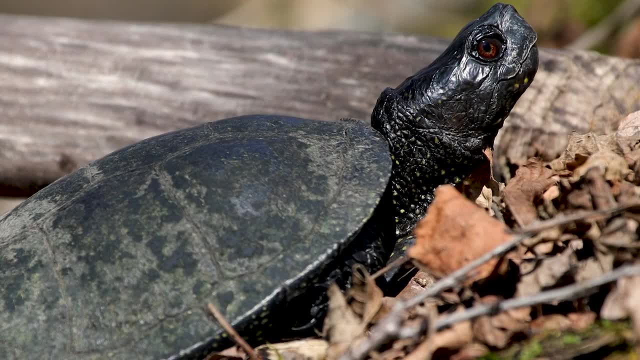 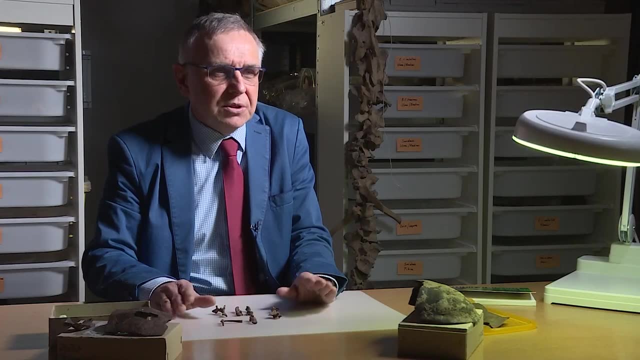 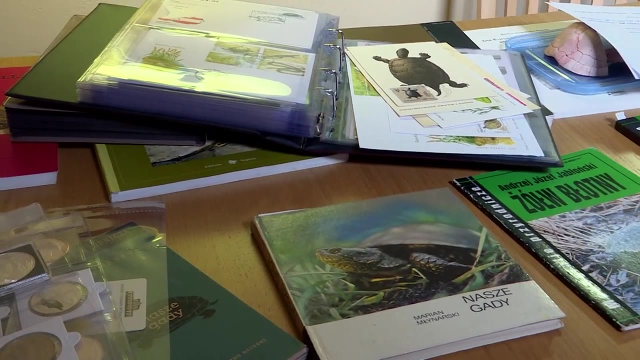 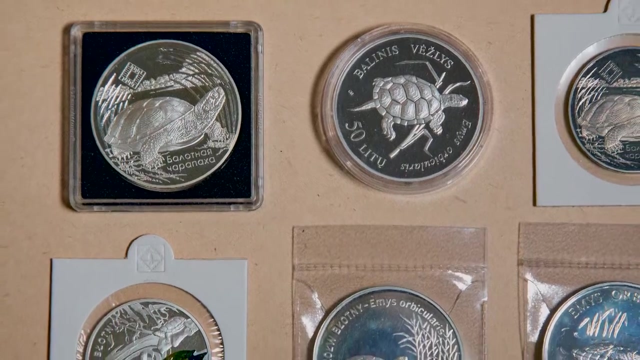 So we can attribute to it the triple significance. The turtle whose skeletal remains we find in excavation and archaeological materials seems obvious. And there's also culture, in a completely different dimension, a more hobbyist one. So the European pond turtle in philatelie, numismatics and heraldry is marginal. 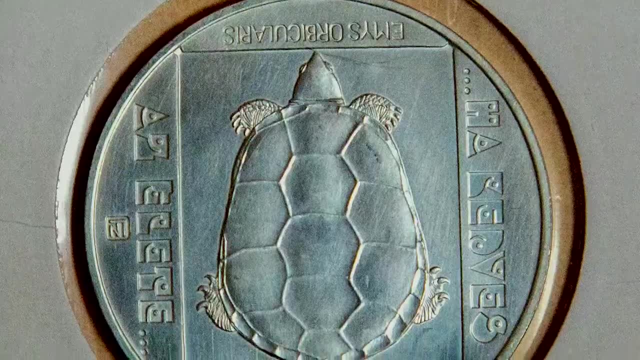 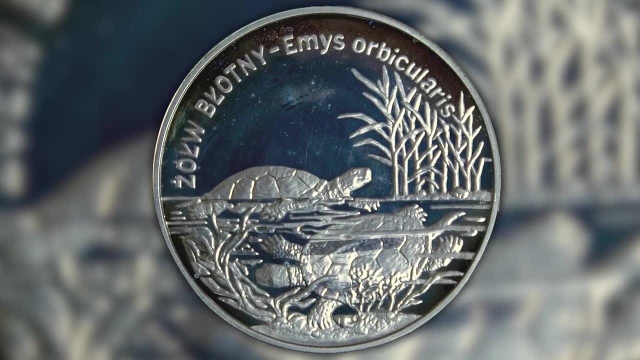 The turtle is, of course, in Majority. In the early 19th century it was the most popular local animal. In 1921, it was the most popular with our european pond turtle included turkey in 2001, poland in 2002 and then we had belarus. 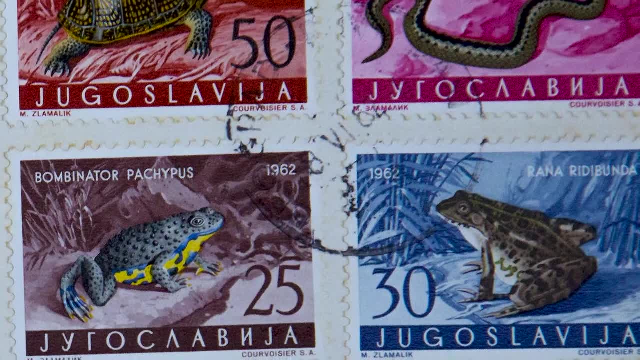 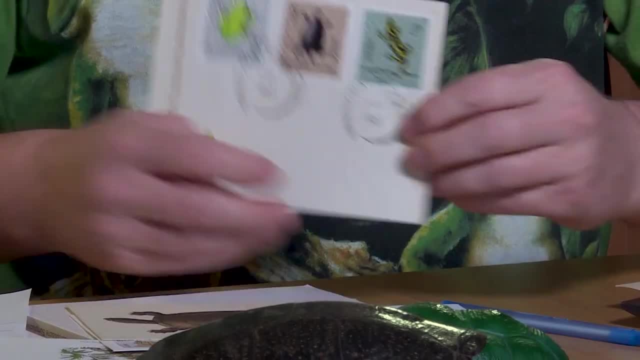 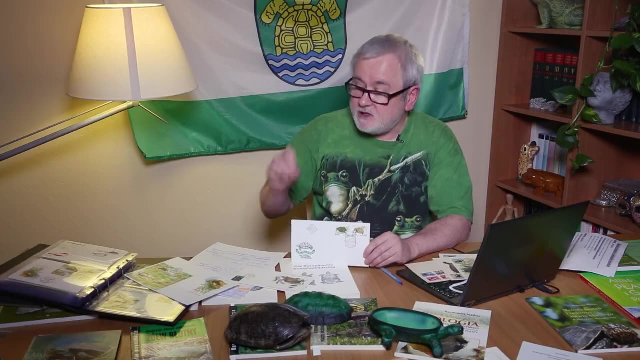 and lithuania. the first stamp ever released in the world was yugoslavia in 1962 and poland in the following year, 1963. it was a series of amphibians and reptile stamps. in bulgaria we have a stamp drawing and another stamp- heraldry- such a hermetic and actually difficult topic in 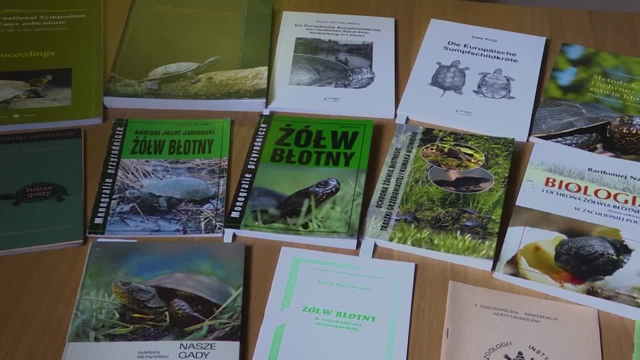 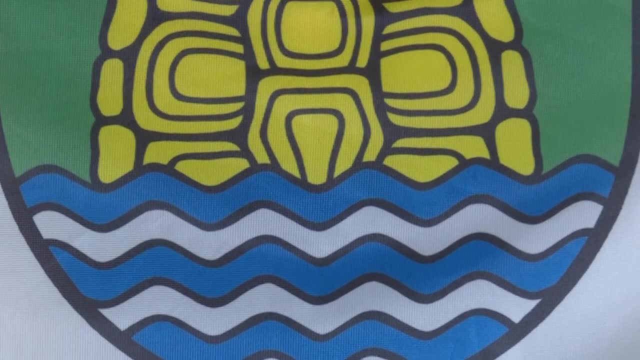 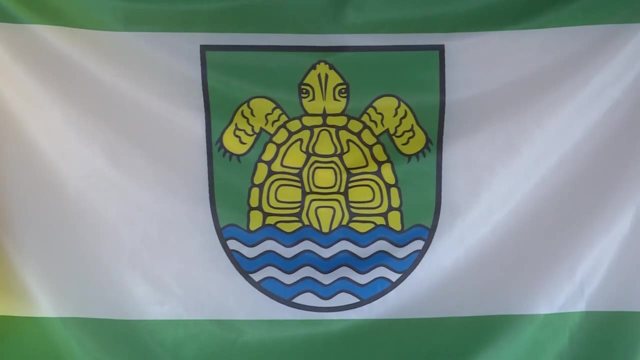 searching for this turtle subject, because it hardly exists. there is the grunheider commune with the turtle coat of arms. this is german brandenburg, literally 25 kilometers from the polish border. from swobice more or less, this coat of arms was borrowed from the brandenburg electors who had long appreciated the importance of the european 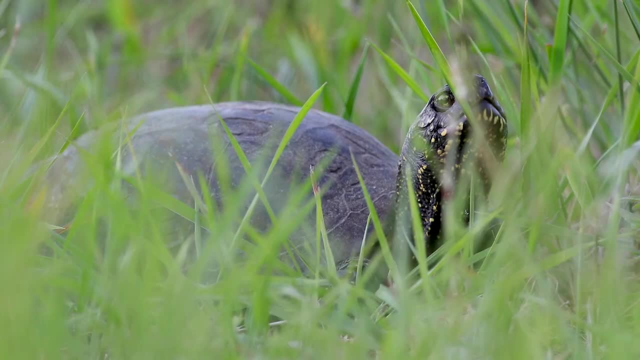 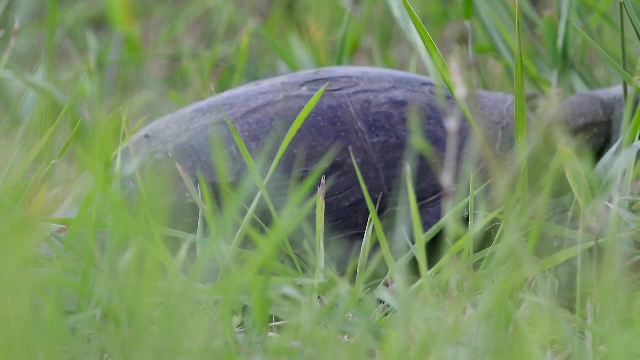 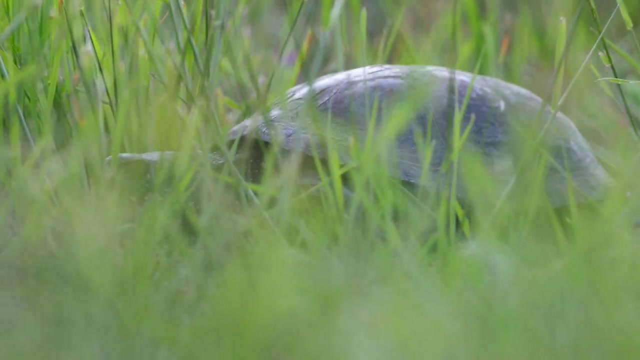 pontoon, when the european pond turtle was numerous. it was caught and then eaten, and these inhabitants did not have a coat of arms. so how to use it? well, someone came up with the idea: and this coat of arms with this animal, which is interesting, rare, attractive, that this will be. 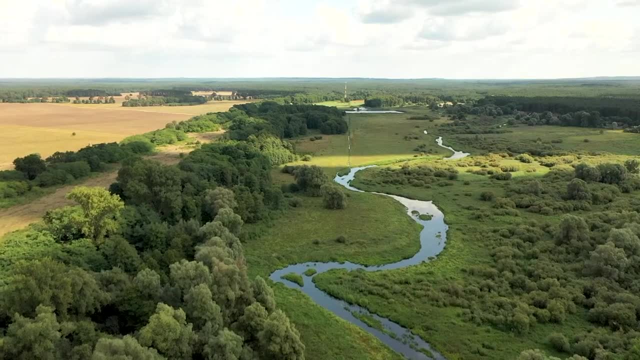 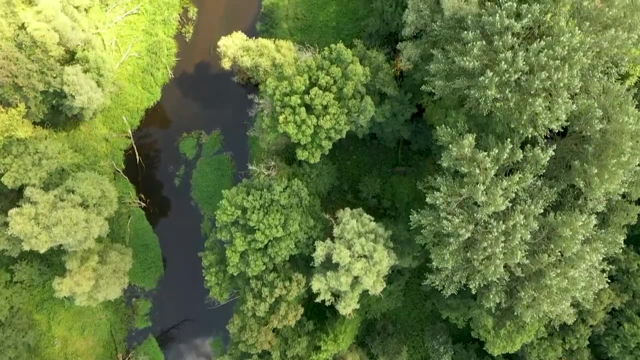 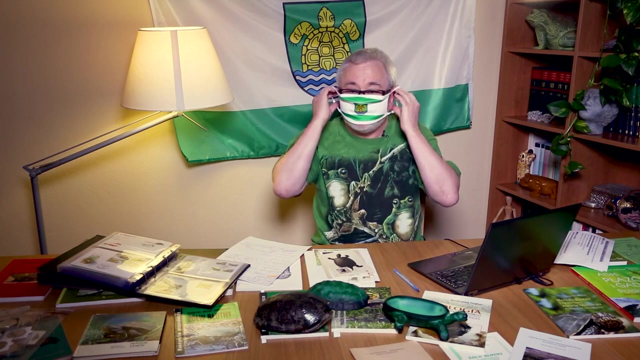 the new symbol of the commune, and they just set themselves up for a completely different view of the turtle. the turtle now advertises a clean environment, those people who live among forests, lakes and so on. and- a curiosity about which i did not know- i found something up to date: this coat of arms as well. 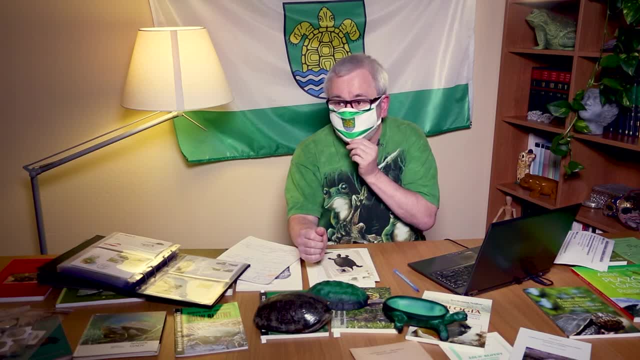 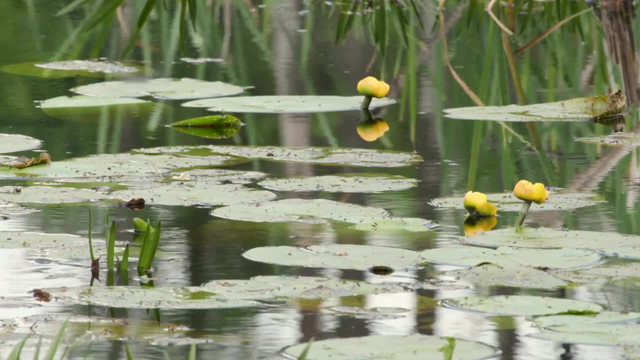 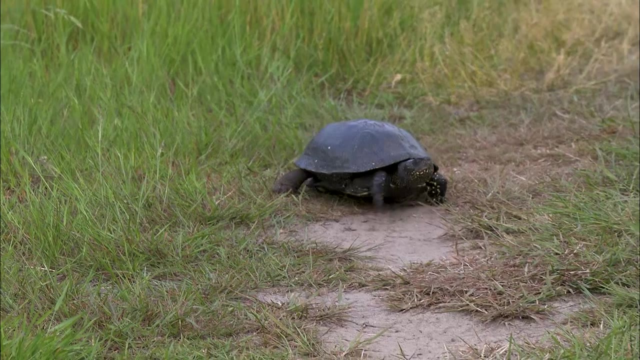 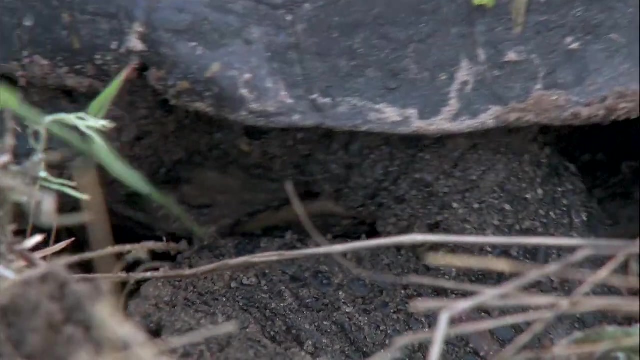 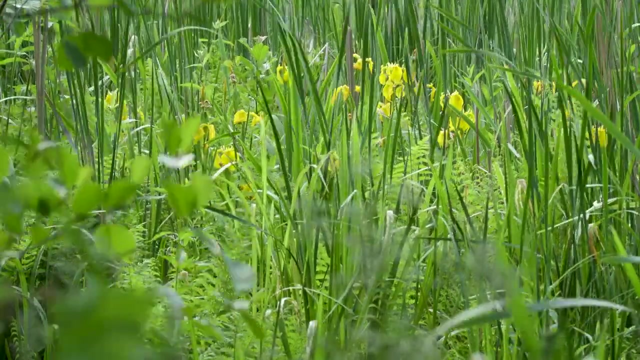 about our turtle. this is how it is advertised. In the third decade of May or early June, the females leave the water to lay their eggs. This period coincides with the blooming of the yellow iris. Yellow irises are therefore the most important indicators of European pond turtle hatching. 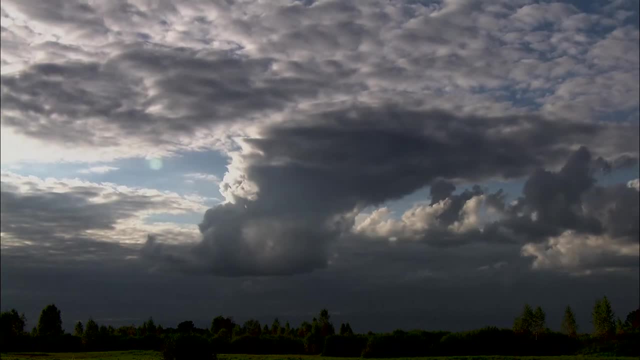 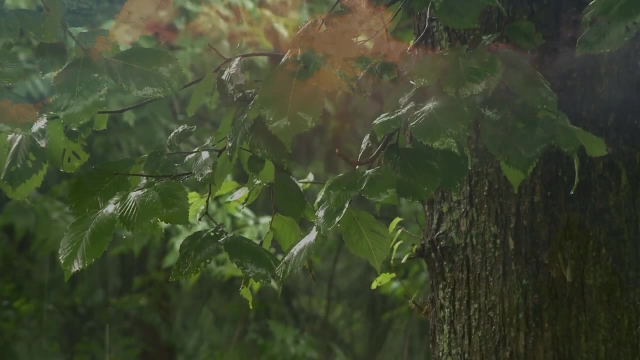 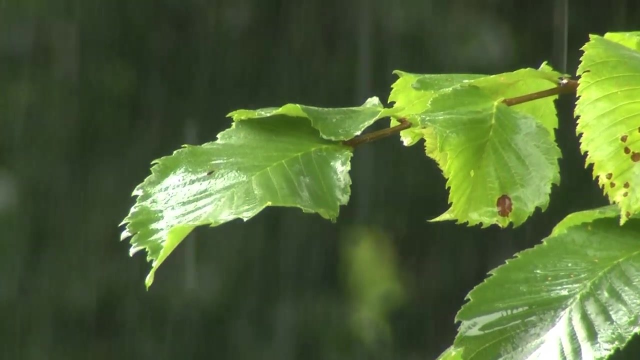 This is also the time when the marsh Labrador tea is in full bloom and when the mosquito and the blackfly are at their peak. Egg laying very often starts just after rainfall and storms. The ground moistened at the time makes it very easy for the females to exhaustively. 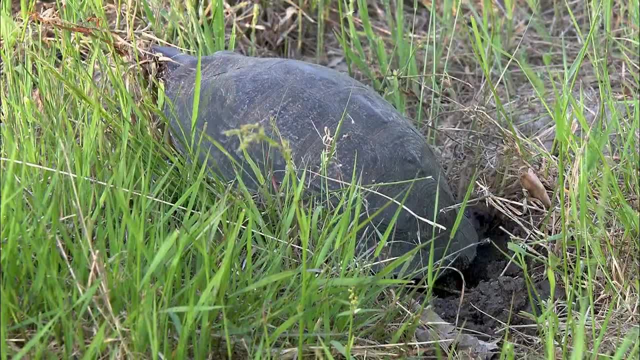 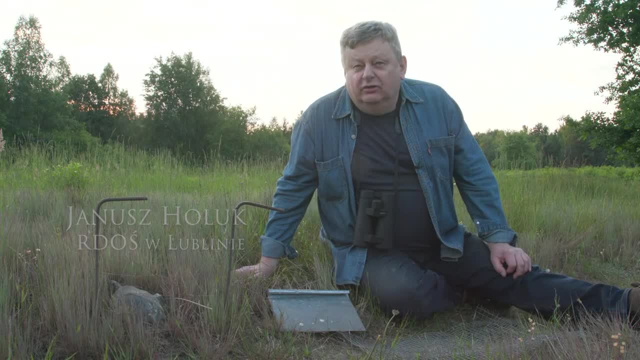 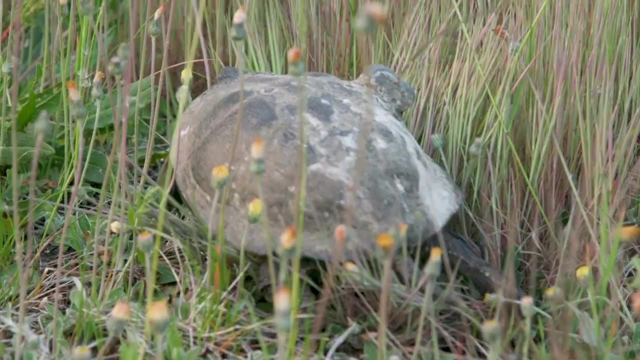 dig the egg shell. Tracking a European pond turtle using traditional methods is almost impossible. it is just coincidence. Thanks to the transmitters, however, we have learned about the migration routes, how they move their movements. This is completely different from what we thought. 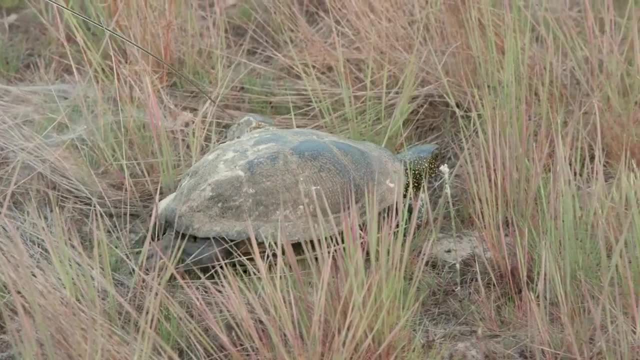 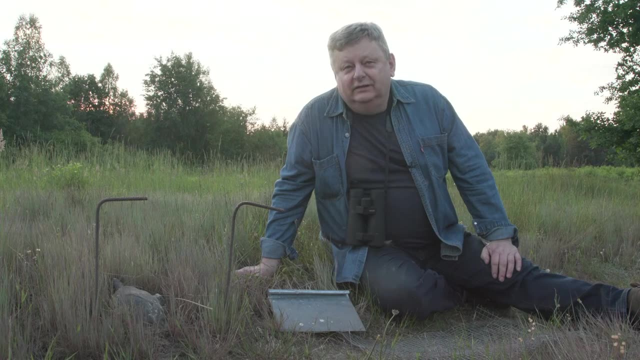 We think that if we've been observing turtles for 20 years, we know a lot about them. The telemetry research has verified this very well And, in fact, we still know very little about them. We know very little about them. We know very little about them. 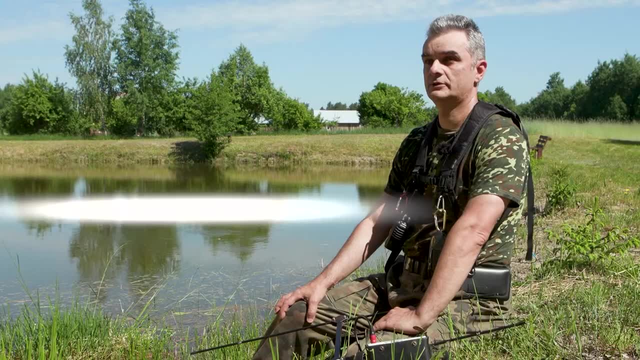 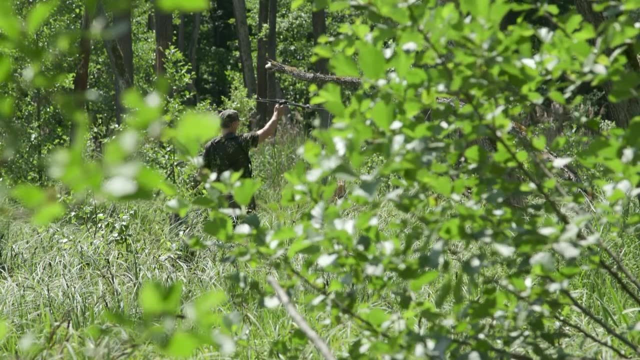 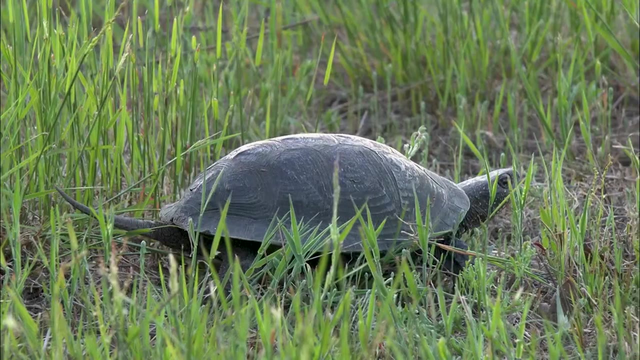 Telemetric studies, or in fact radio telemetry, because here we track the radio signal for a transmitter, allows us to discover migration routes – wintering sites – those place where they feed after breeding, characteristic of the particular species Podern sama. 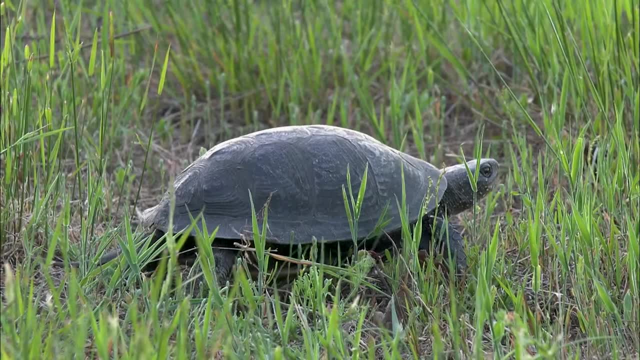 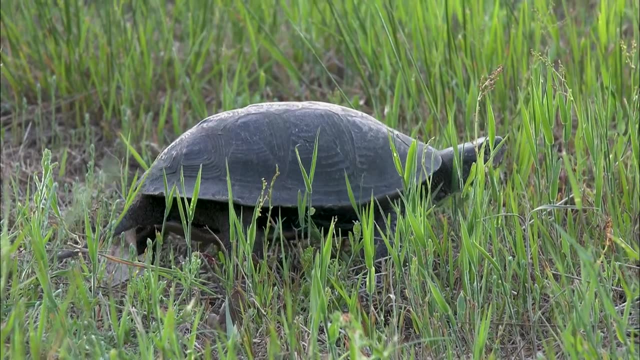 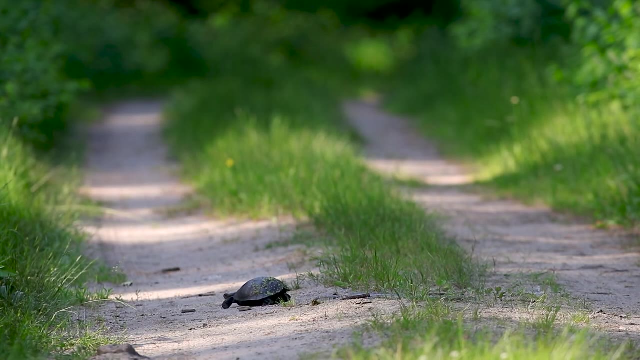 Occasionally, a female pond turtle can be seen heading for an egg laying site. Jr L- 안녕, IM am Hm. Occasionally it crosses the road. people catch it and carry it away. Reports of run-down individuals and sightings of turtles on the roads testify to the high 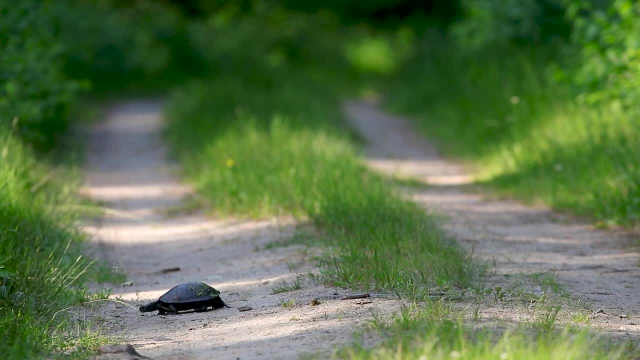 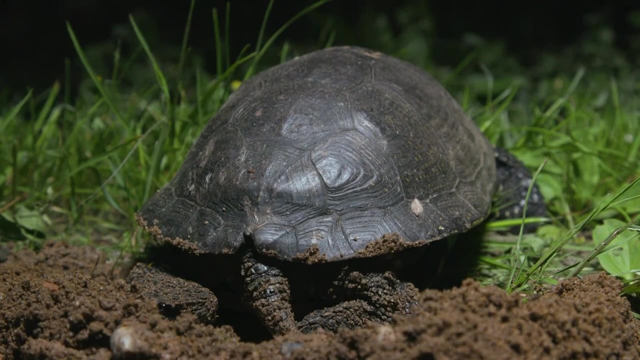 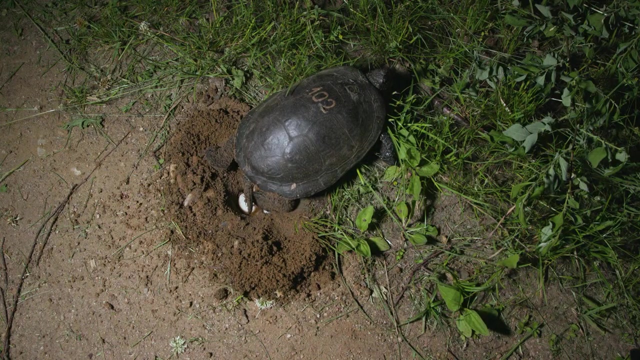 risk to this species from drivers. Recently we had a situation where a certain person came across a female on a forest road digging a nest and caught the turtle and carried her into the forest, interrupting this egg-laying process. If she leaves the water and she walked for two days, those two days she has to return. 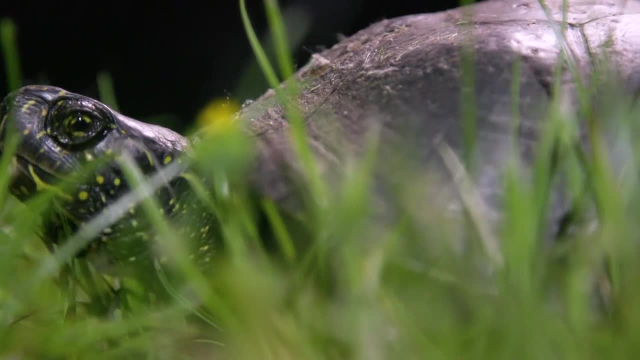 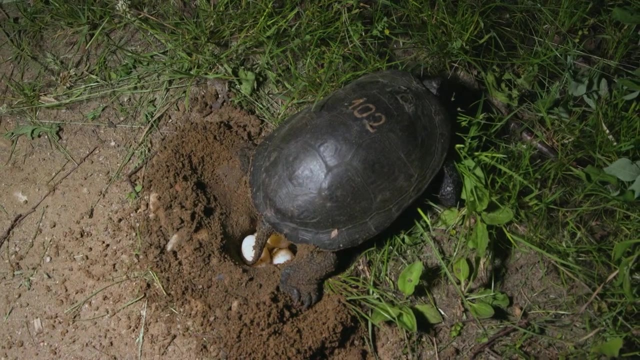 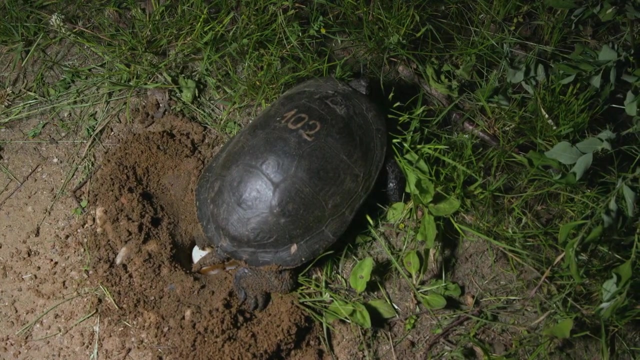 to the reservoir from which she came to get water. This doesn't seem like much, but a week lost in the case of a cool, rainy summer can result in those little turtles not hatching, not incubating, and simply the entire hatchling being lost. 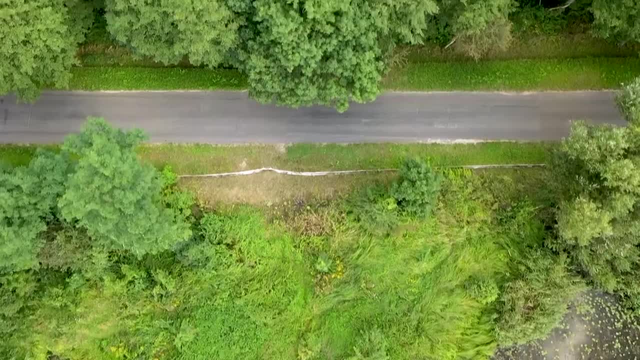 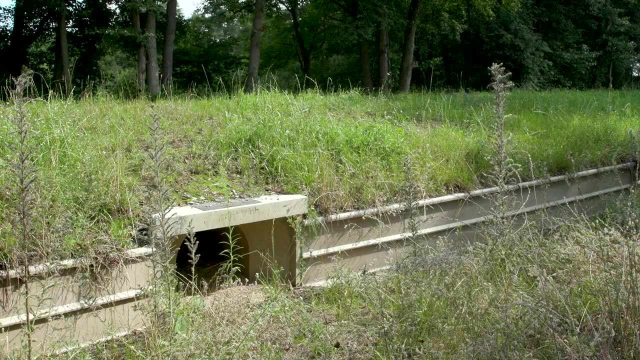 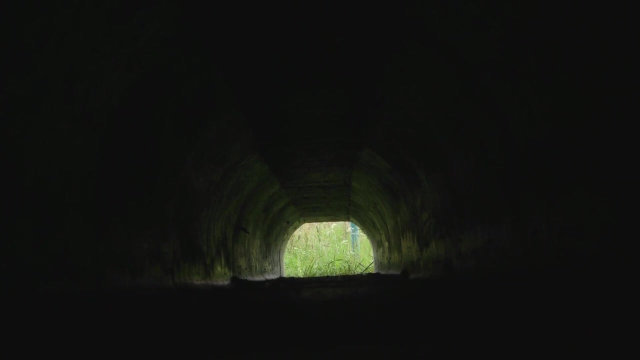 In some cases, Clearing existing passes can eliminate the need for turtles to cross the road. There are also already the first underpasses built specifically to protect migrating turtles. They also serve many other animals. The purpose of this passage was to increase safety during the migration of females to 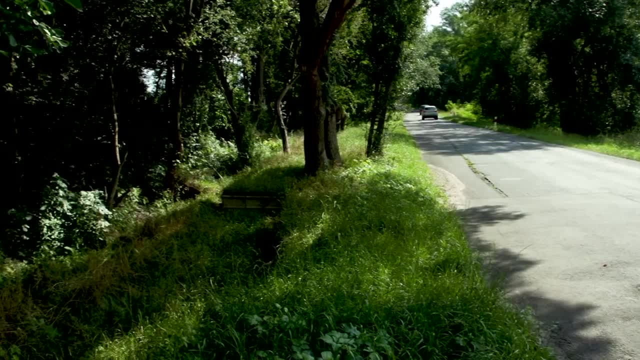 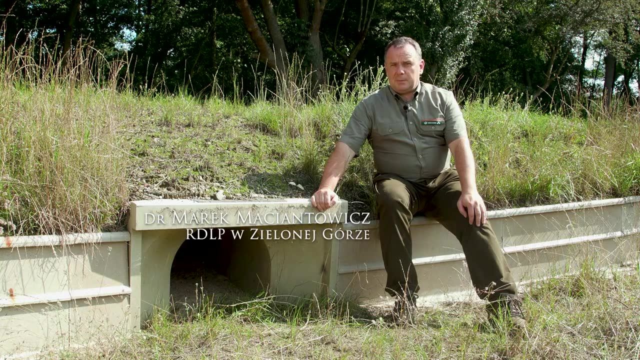 the breeding ground. The females have just been crossing this road which is right behind me, and there have been cases of them being run over by cars, Which here Traffic is not the heaviest, but still it happens and they often pass. 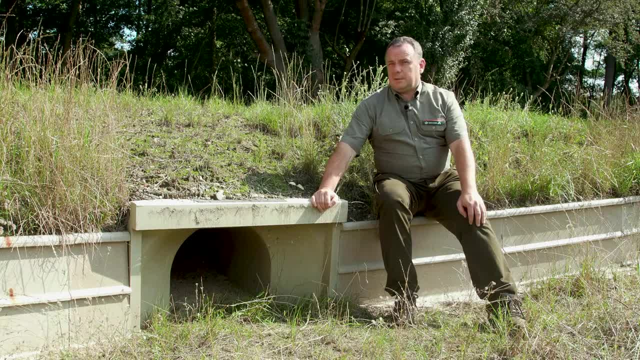 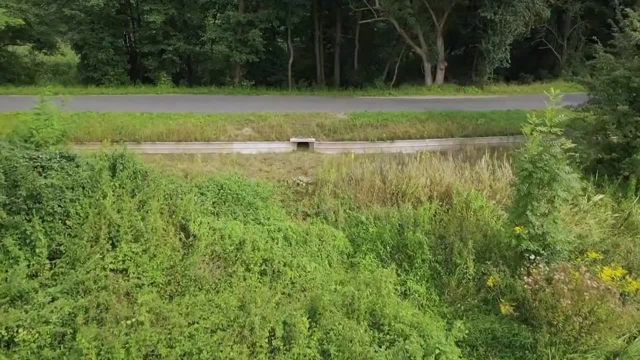 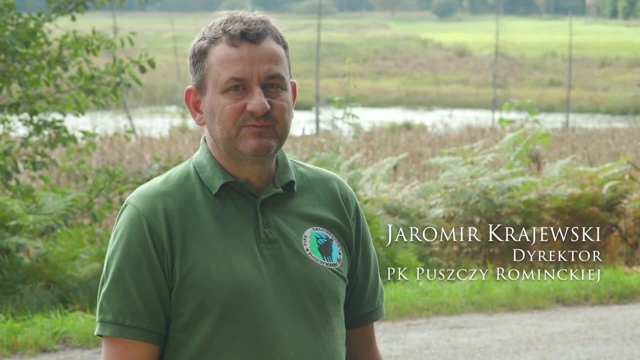 One car has just passed. Thanks to this, the turtles can safely cross this road, and we can hope that this safety will increase. There are many such crossings for small animals, but no one has yet built one dedicated to the European Pomp Turtle. 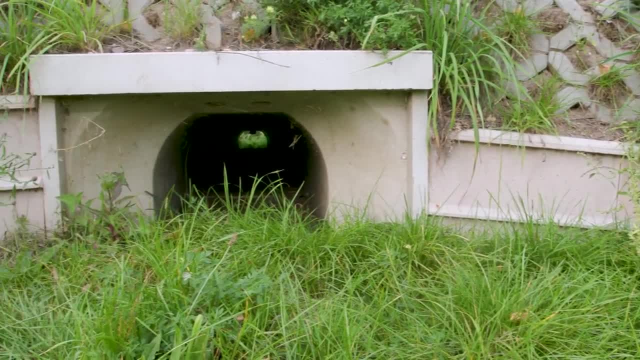 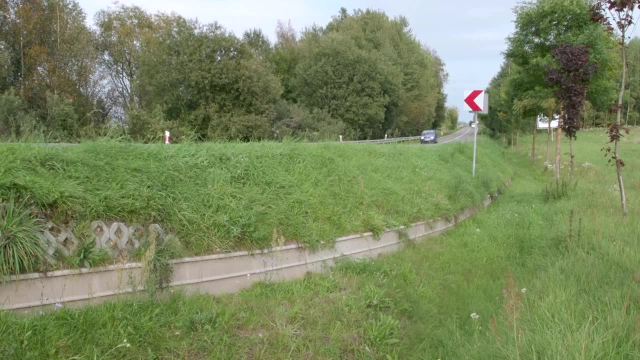 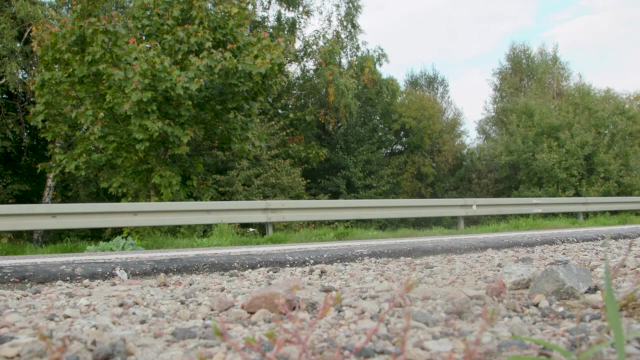 So there is no information on how such crossings should be built, Whether they are safe or not, Whether they work or how they will function. We will have done this, and the first monitoring results have shown that European Pomp Turtles do indeed use these crossings and, as a result, do not die under the wheels of speeding cars. 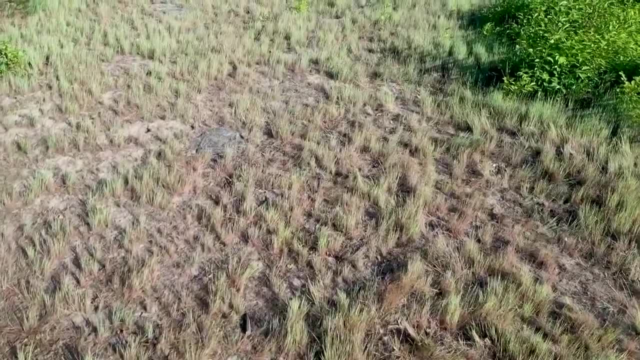 The breeding ground is usually a sandy area covered with xerothermic vegetation. It is most often a grassland with grey hair grass, Less often with fescue grass. The breeding ground is usually a sandy area covered with xerothermic vegetation. It is most often a grassland with grey hair grass, Less often with fescue grass. 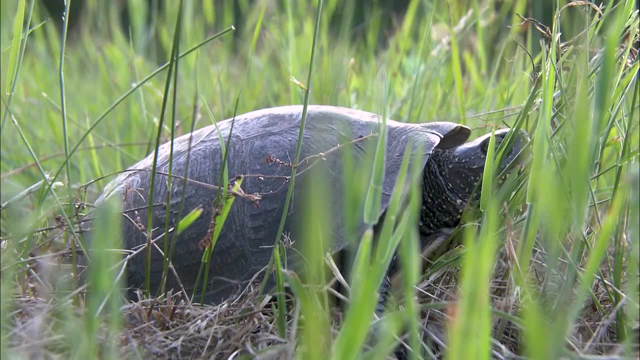 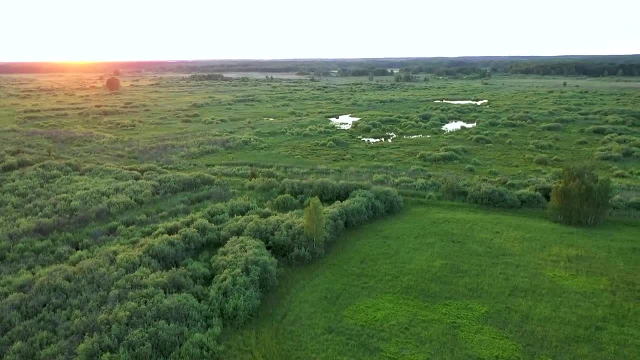 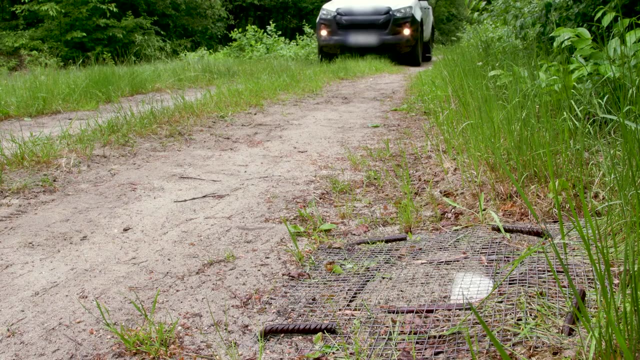 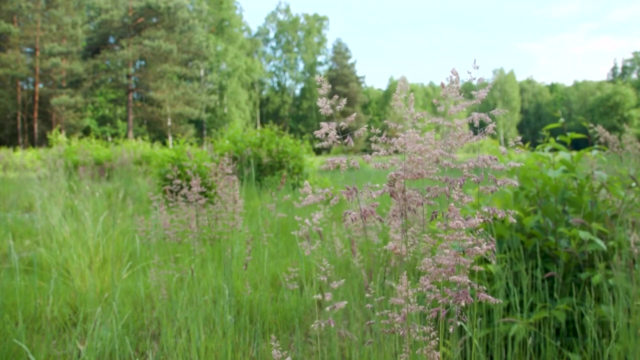 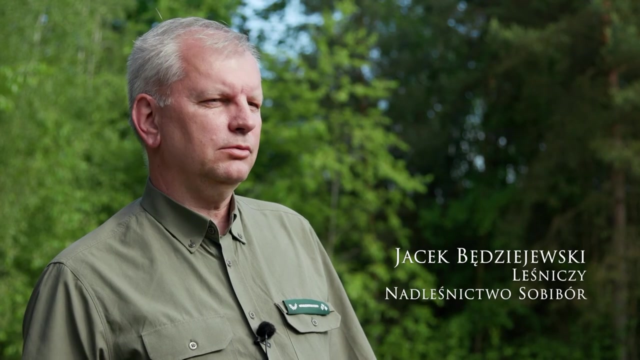 It also happens that females choose to lay their eggs in the middle of field or forest roads, farm fields, pastures and even home gardens. Turtles can sometimes even take advantage of our forest management. They use the logging that we cut down when we carry out our management activities, and 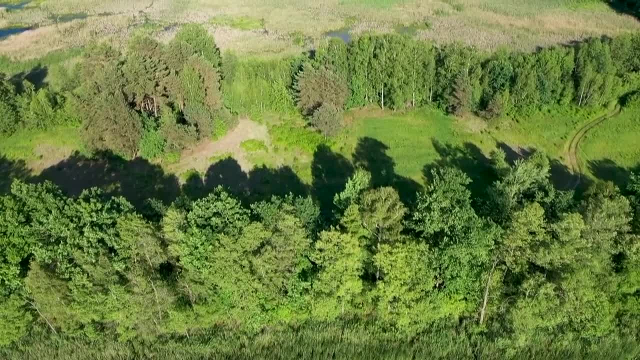 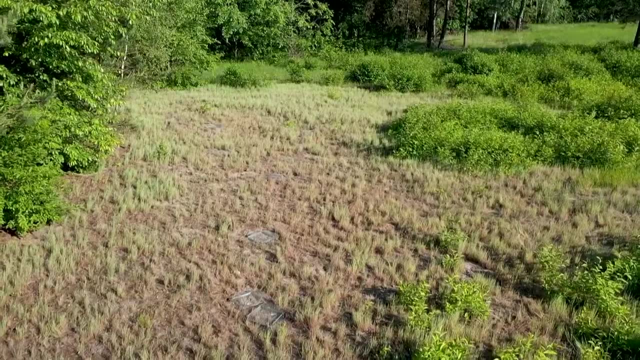 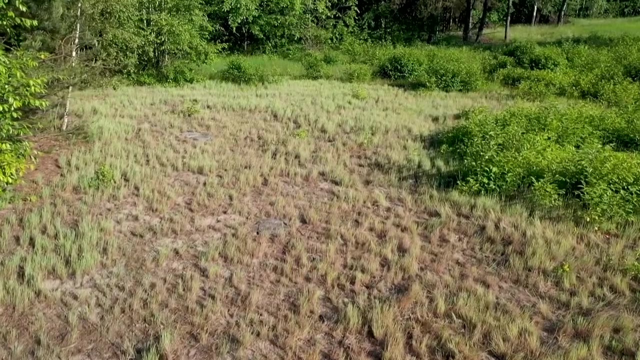 if the thermal conditions are right there, they nest, they get peace and quiet, and hence we have new generations of baby turtles. Female turtles are constant in their choice of location and, over the years, come to lay their eggs where they have not done so before. 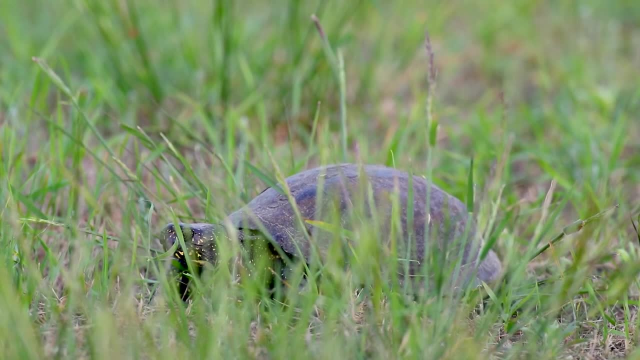 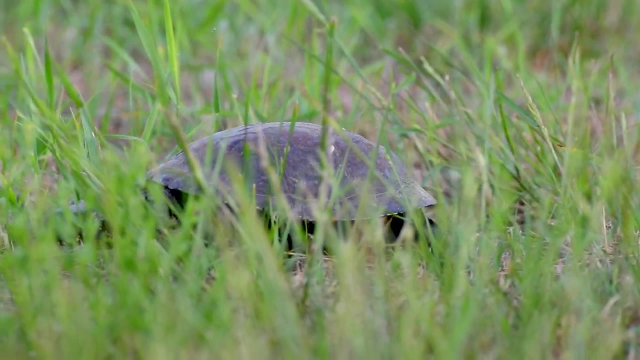 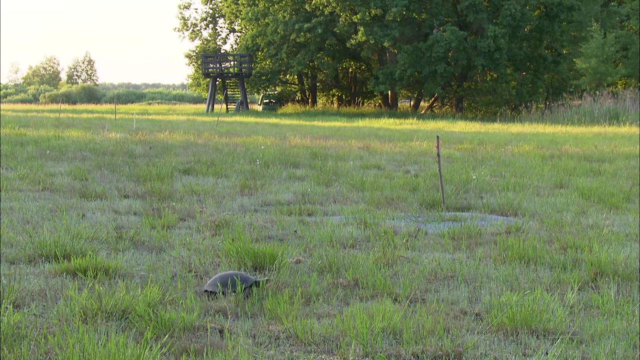 Sometimes it is only a distance of a few meters between the nesting chambers that the female digs in successive years. Turtles are quite attached to certain habitats, and it is also said that females usually go to the same place to lay their eggs, although sometimes it has happened that they change. 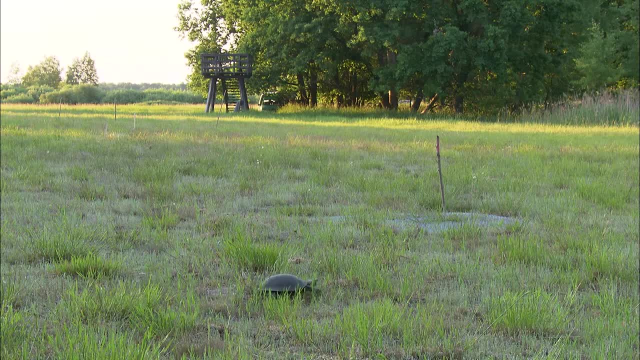 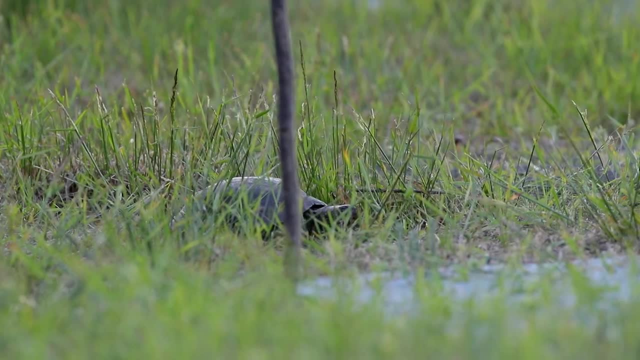 their habitat, and so, from time to time, the females look for another place to lay their eggs. Perhaps this is a certain strategy to protect the eggs from destruction, because sometimes it pays to leave them in a different place, in a place that is not penetrated by predators. 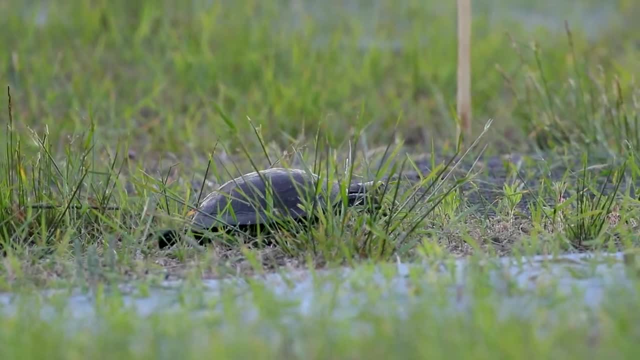 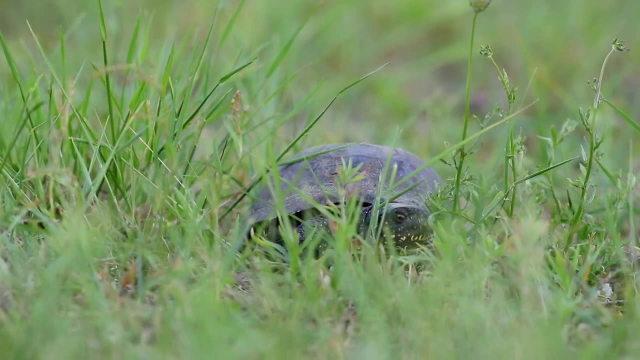 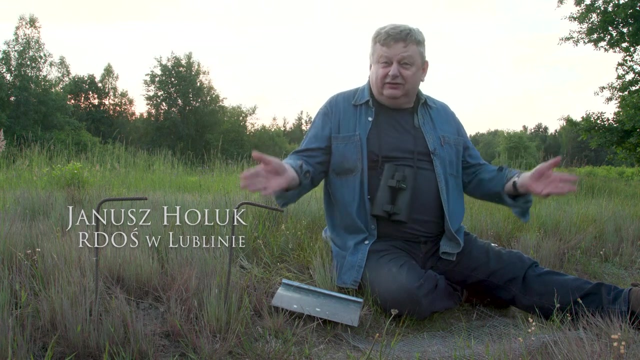 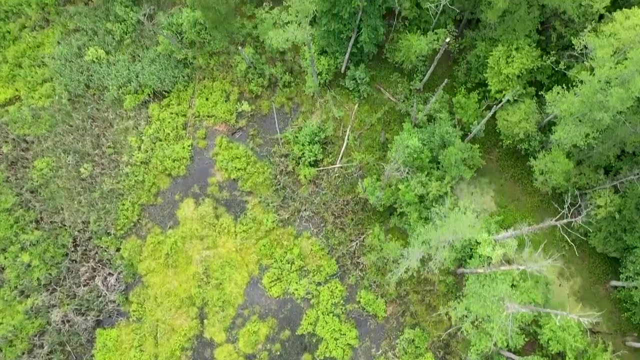 for example, because this is one of the biggest threats to turtles today. The place where the female turtle lays her eggs is chosen very carefully, Sometimes on one nesting site. she goes for four days and looks for the right place When I know there are dozens of nests here. so generally conditions are good and she goes. 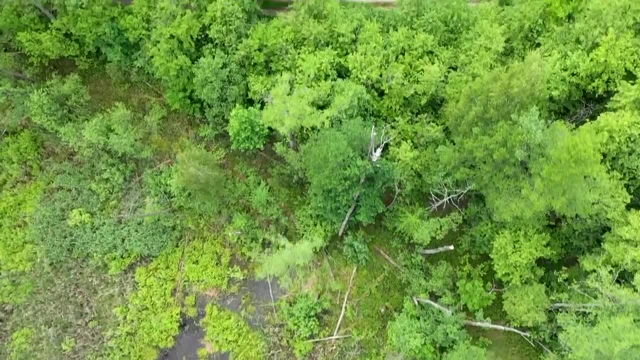 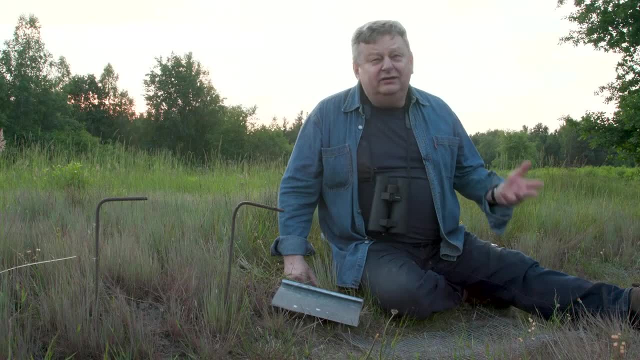 for a few days and looks for a place. The breeding ground is usually a dozen to several hundred meters from the water, sometimes further, even up to two kilometers. We have this information that it's very far away because she doesn't choose every place. 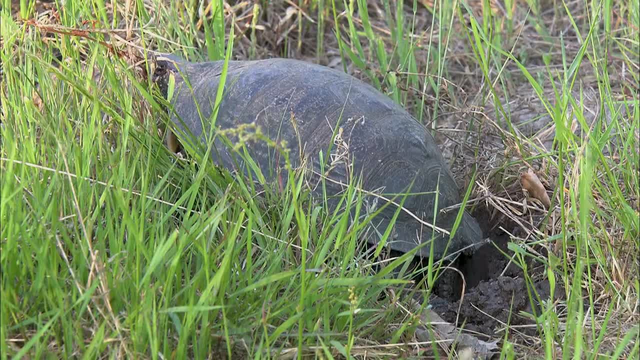 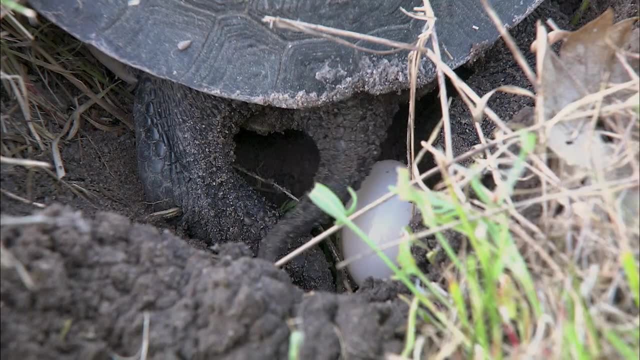 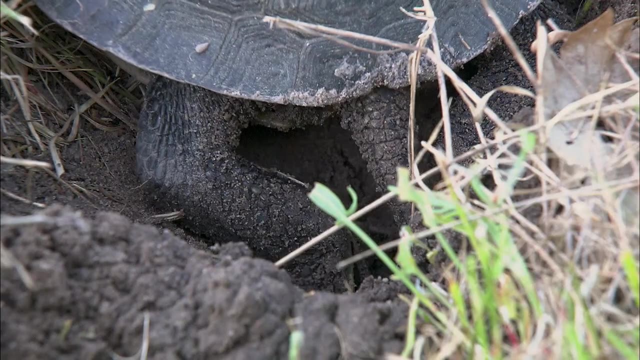 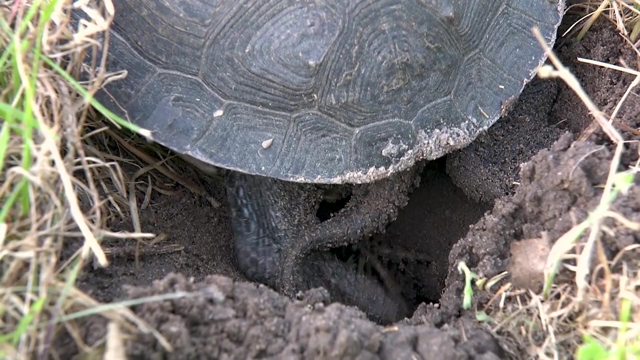 Depending on her age and size, the female turtle lays between 7 and 23 white eggs. They are usually laid between 6 and 10 pm and the whole process takes 2-3 hours. The female digs the egg chamber in a sandy spot that is sheltered by vegetation. 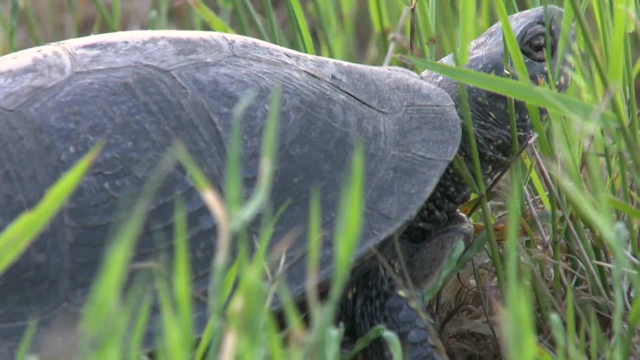 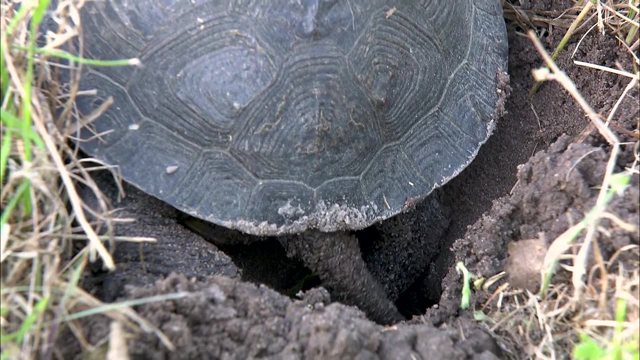 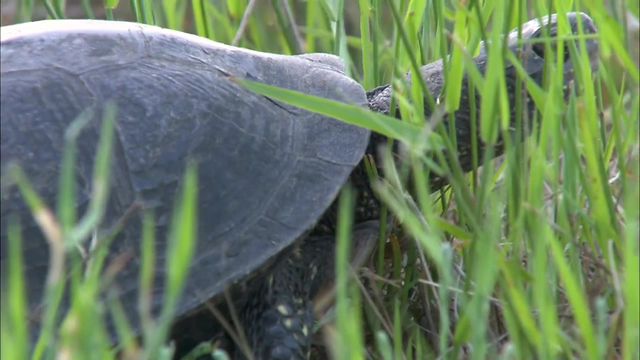 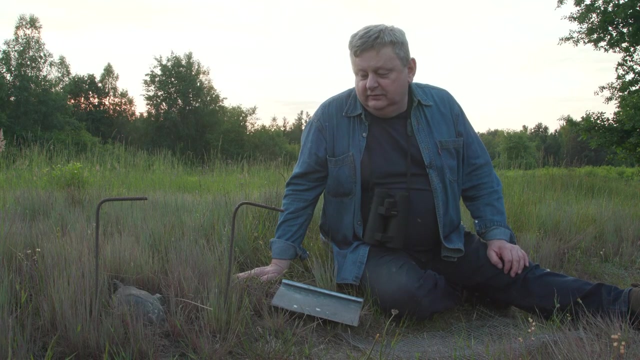 The hole is pear-shaped and up to 15 cm deep. If frightened, the female turtle usually moves away and lays her eggs elsewhere. However, once she starts digging, she becomes less shy. The female turtle is very shy. I would like to draw attention to one thing. 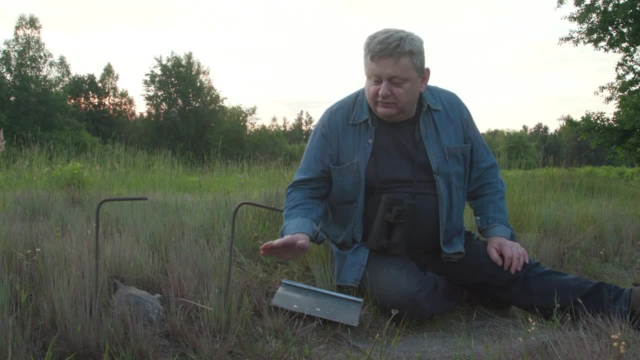 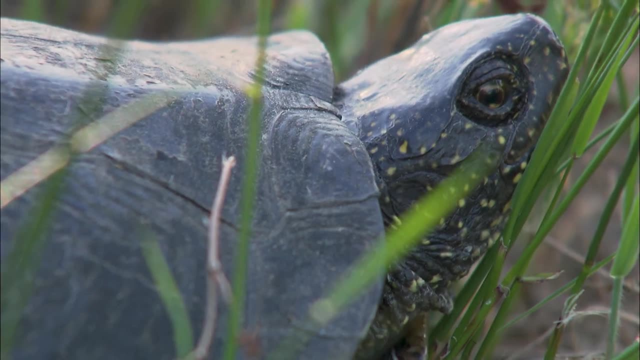 The fact that I am sitting next to this female is an exceptional situation, Because she has actually finished. she has set up her nest, she has buried her nest and she will come down at any moment. She has done her job. so I can sit next to her because, even if she goes away, nothing. 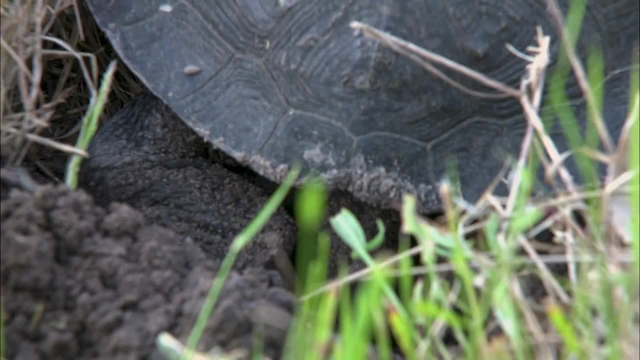 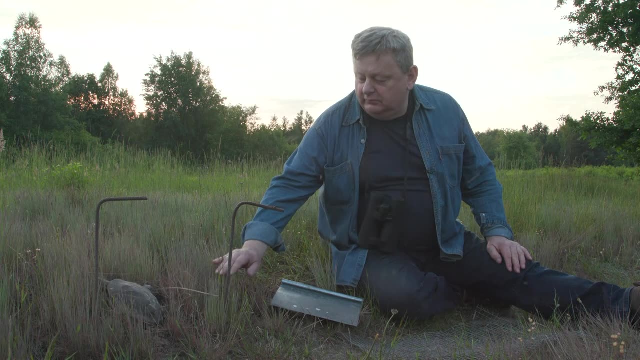 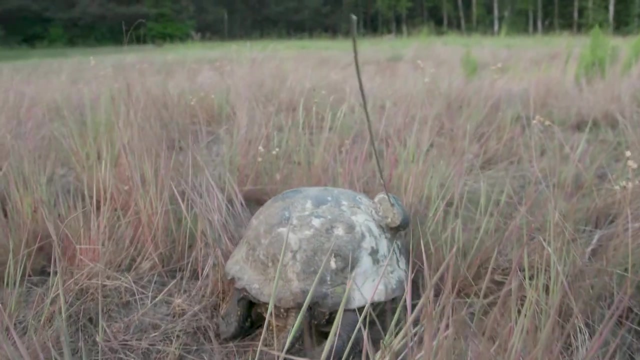 will happen. However, we appeal to all turtle lovers and observers During this period, May and June: don't disturb the turtles. Oh, she's just starting, let's take a look. There you go. you can see the transmitter. She's done her job and now she's leaving. 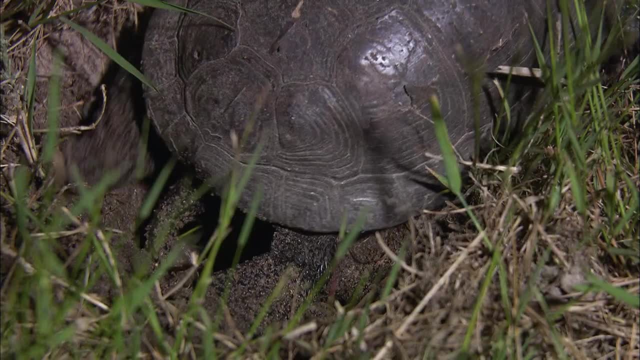 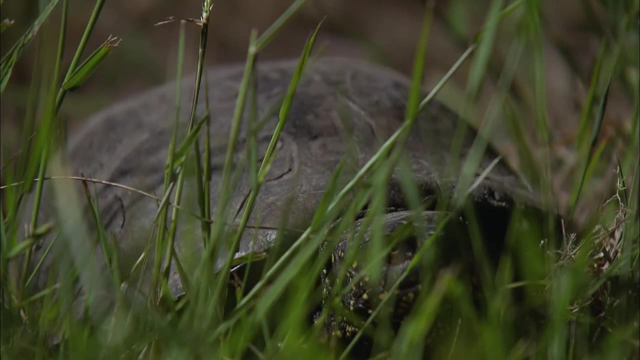 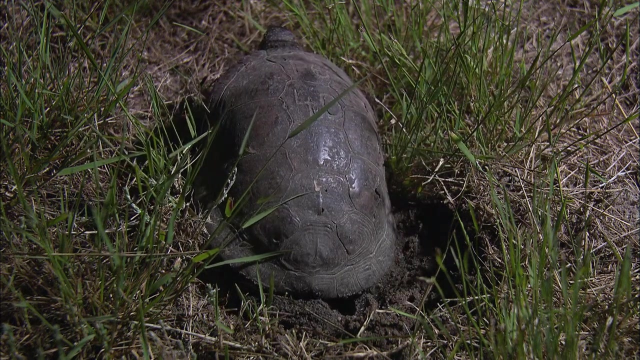 When digging, the female often softens the soil with fluid from her anal bladders. She uses her hind limbs, which work like a digger, to dig the egg chamber. She lays the eggs directly into the hole and mixes them with the sand at the bottom. 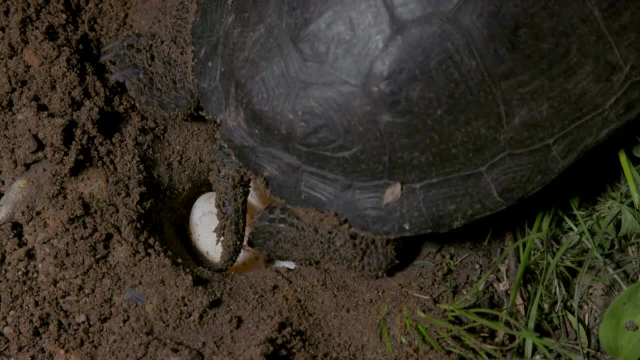 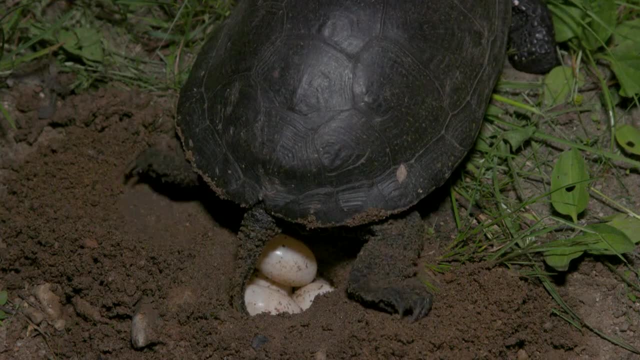 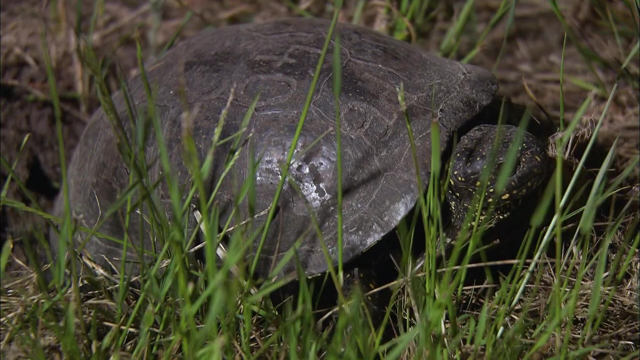 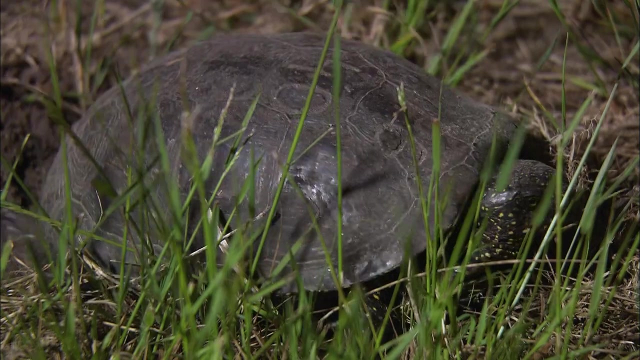 The female turtle is now ready to dig. After laying the eggs, the female masks the egg chamber by covering it up and quickly returns to the water. Female turtles lay eggs only once a season, although in eastern Poland there have already been reported cases of their repeated laying in the same season. 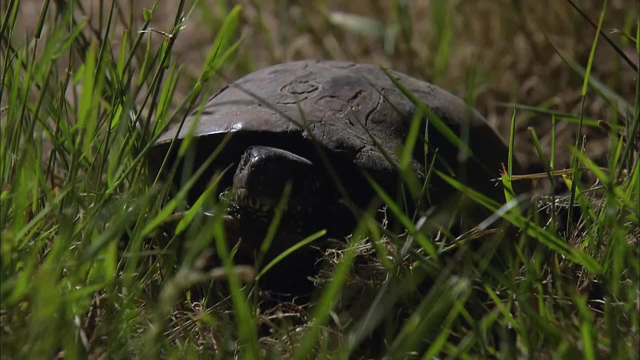 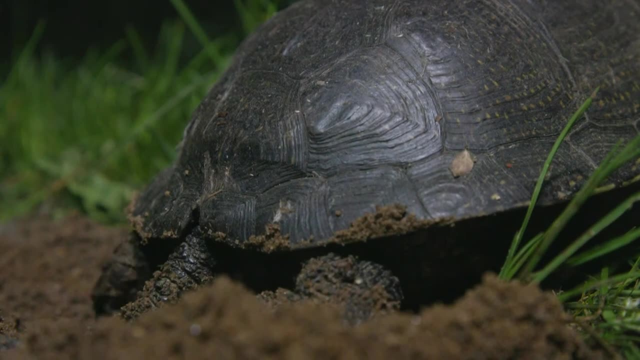 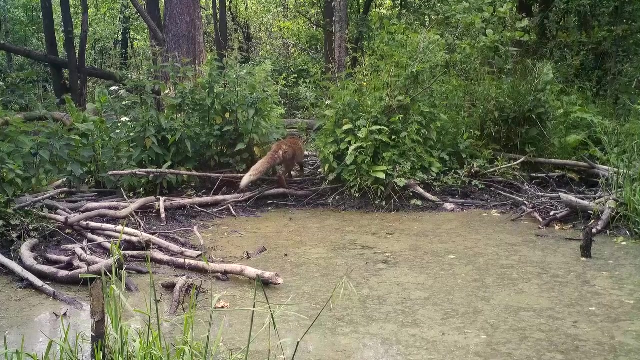 Such a situation is encountered in the countries of southern and western Europe. for example, in France, European pond turtles are very often exposed to attacks by predators. During an attack, their carapace is most often damaged, or a body part such as a leg or a. 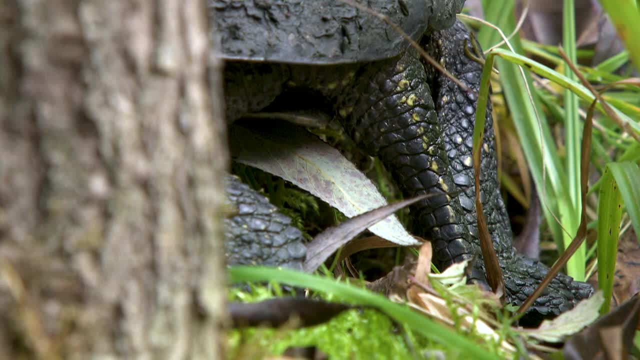 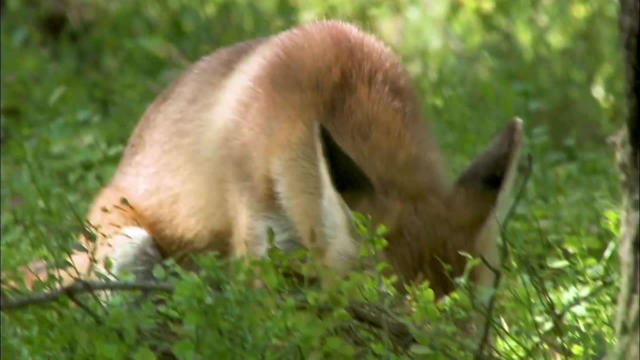 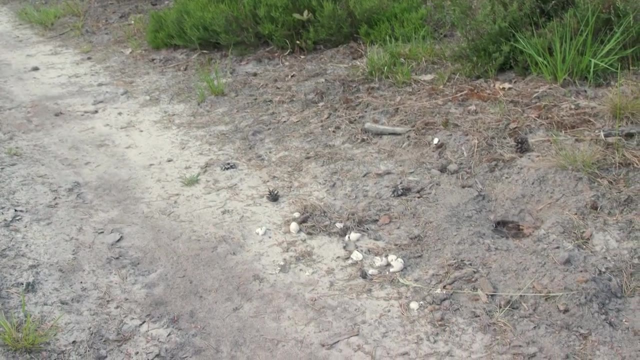 tail is bitten off. Predators also destroy nests with eggs. Foxes, raccoon, dogs, badgers or ravens, and even wild boar, are the animals that most frequently destroy nests. However, there are probably far too few places where turtles lay their eggs as more than 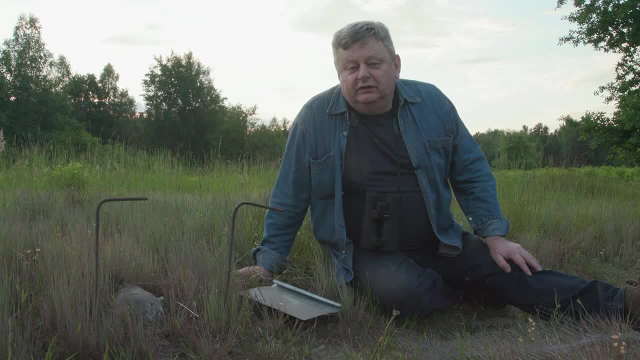 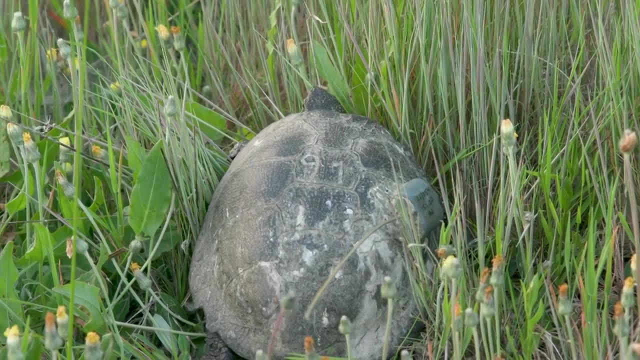 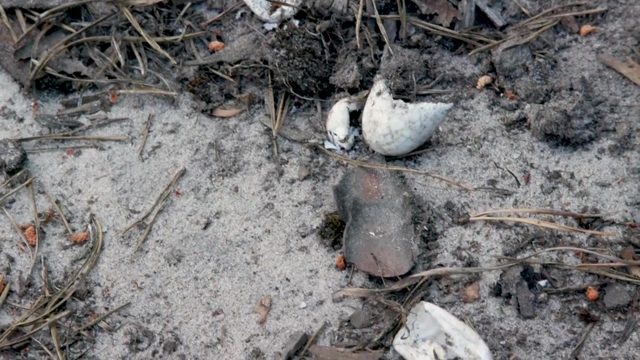 30 females sometimes go out into this small field one year. They come down from a large area and this accumulation of nests is easy to track down by predators, mainly foxes. Around 70 to 90% of the egg deposits in our country are dug up and plundered by them. 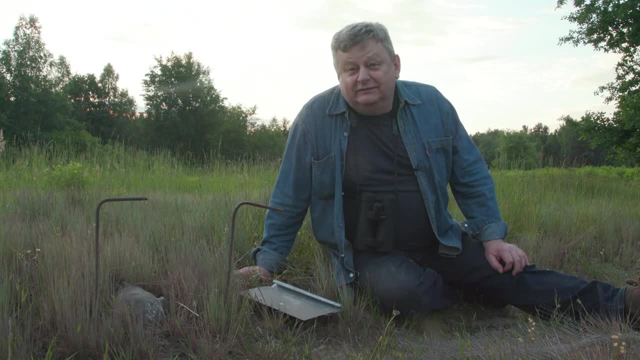 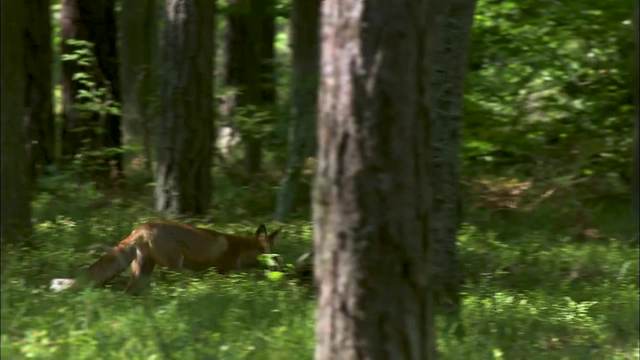 Foxes are the most dangerous, as they remember where the food base is and return regularly. They destroyed 100% of the new nests set up, so to speak. An element supporting breeding success is the protection of localised egg chambers against unwanted intruders. 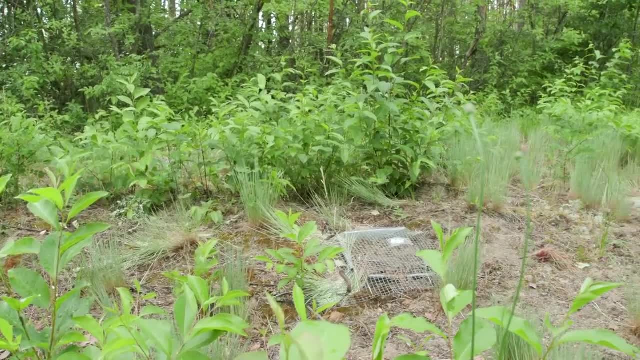 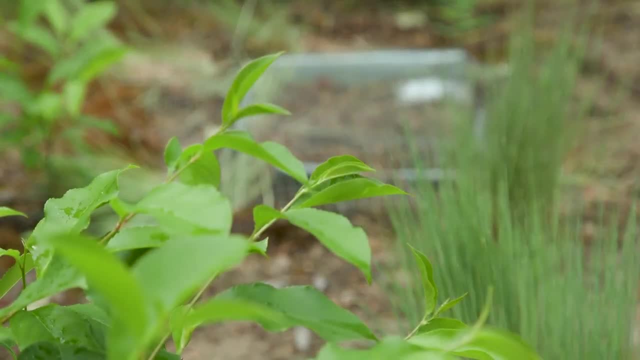 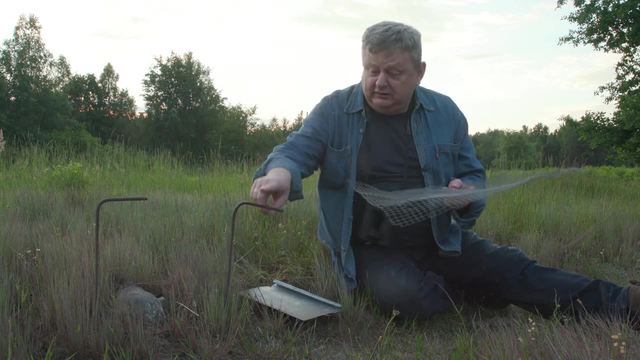 It is a simple and effective way of securing the laying site with a metal or plastic net firmly pinned to the ground. The net was made of metal, but within two to three years the foxes learned to bypass this protection. The net is nailed to the ground with these pins and it really protects from above. But very soon the foxes started digging around and actually after a few years they bypassed all the protection and again destroyed practically most of the nest. For a couple of years now we've had the idea to try this. we call it an armoured star. 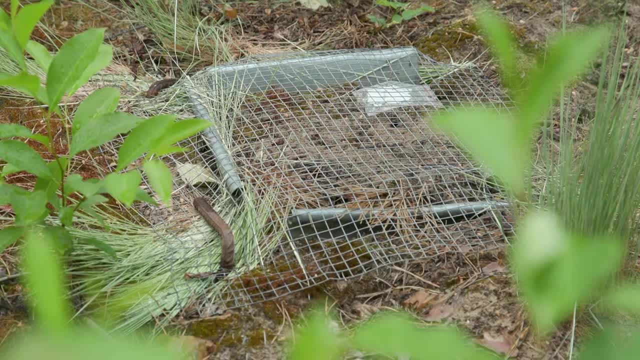 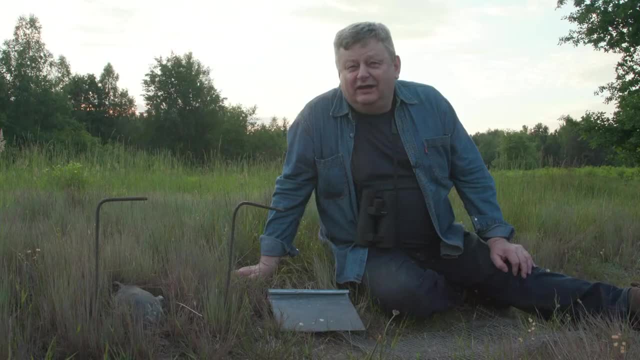 which means netting on top and four metal sheets- actually two on each side, and it really works. At the moment we have a slight advantage over predators, mainly foxes. It is important that the net has sufficient mesh size to ensure free exit for hatchling. 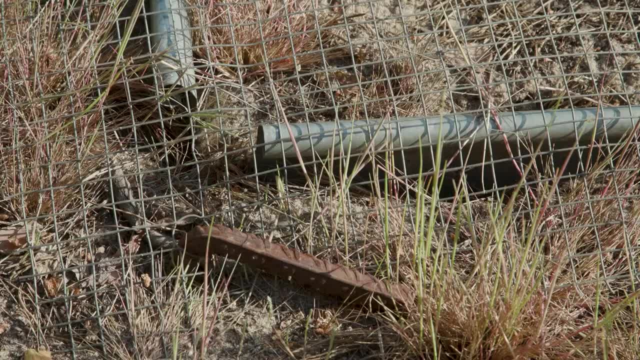 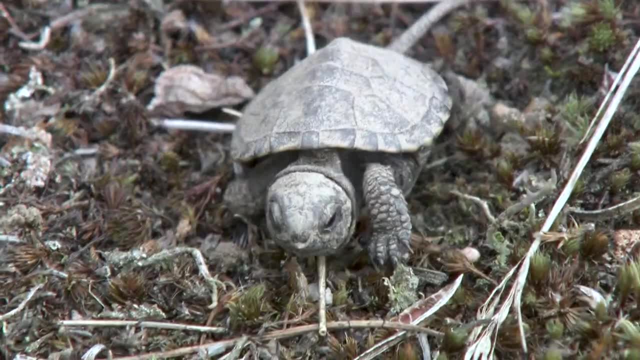 baby turtles, The minimum mesh size must be 2 by 2 centimetres. The net must be 2 by 2 centimetres, So that the diagonal is greater than 2.8 centimetres, which is the width of a hatched turtle. 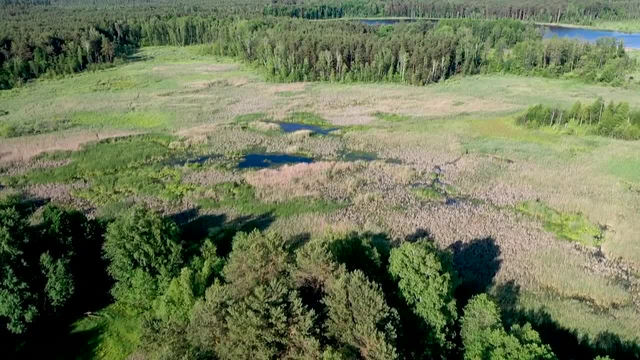 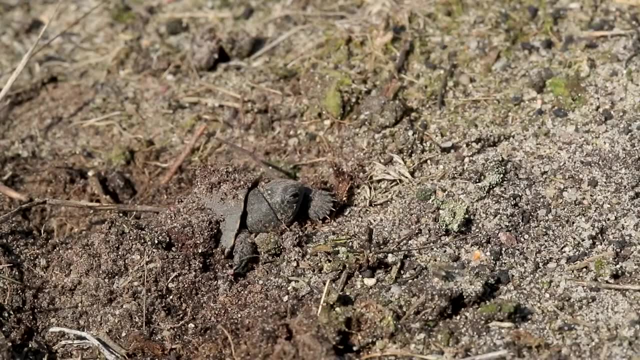 In Poland the incubation of eggs, that is, the embryonic development of turtles, takes about 100 days. At the end of August or in early September the young turtles emerge from their eggshells and go to the nearest water body or remain in the egg chamber where they overwinter. 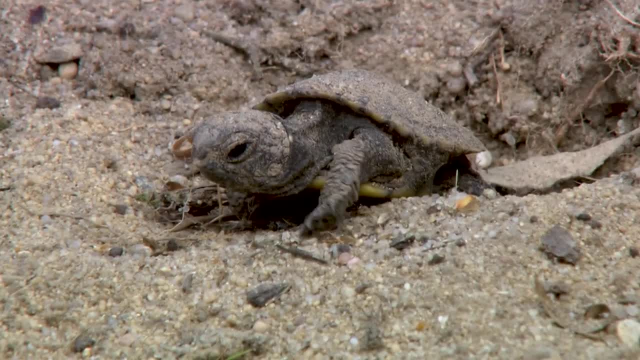 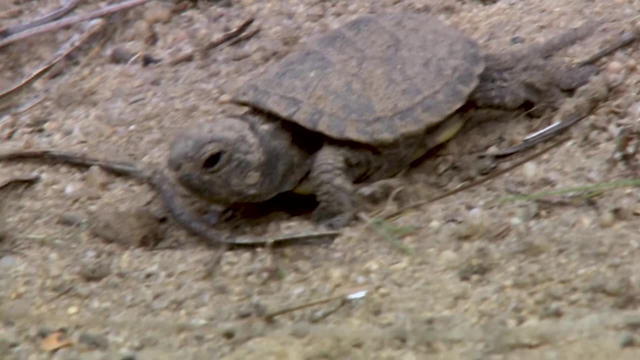 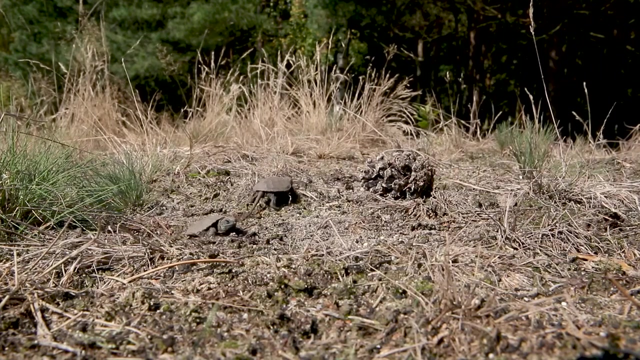 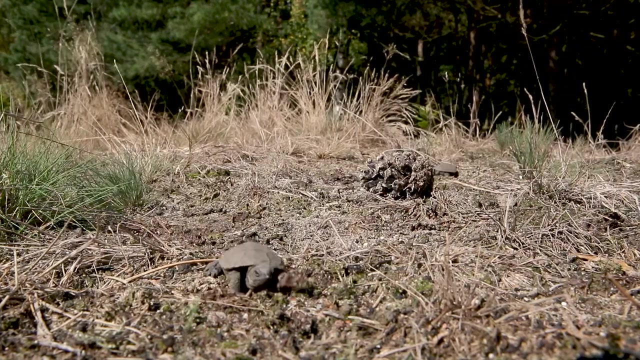 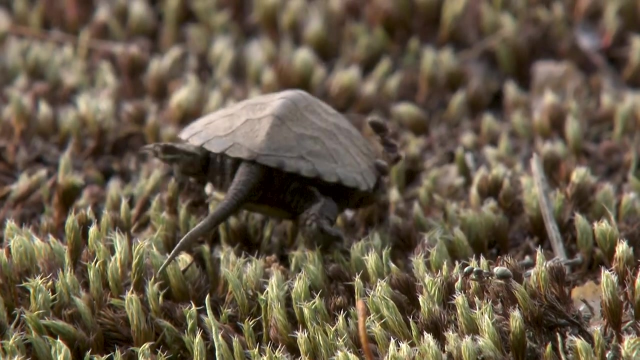 They then emerge the following spring. In turtles, as in other reptiles such as crocodiles, there is a temperature-based sex determination mechanism. Females are usually born when the development of the embryo in the middle third of incubation has been accompanied by maximum temperatures. 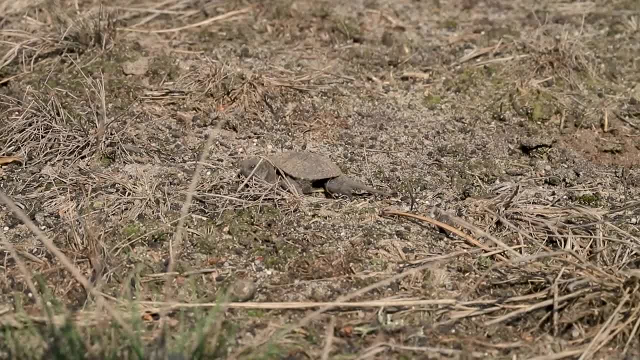 That is cold or hot weather conditions In the middle third of incubation. females are usually born when the development of the embryo in the middle third of incubation has been accompanied by maximum temperatures, That is, cold or hot weather conditions. Females are usually born when the development of the embryo in the middle third of incubation 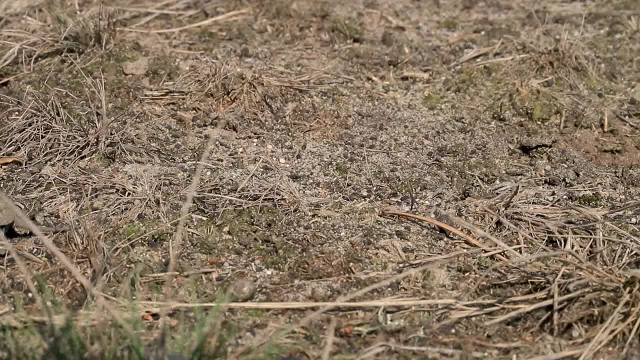 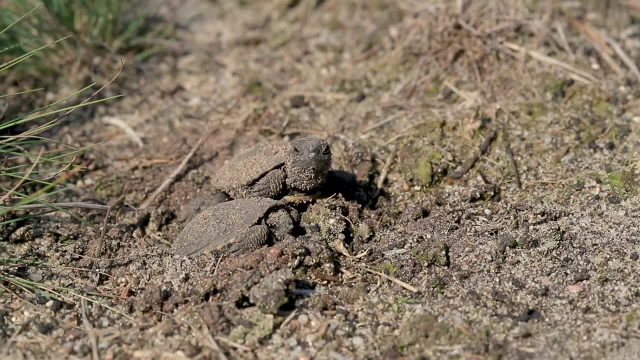 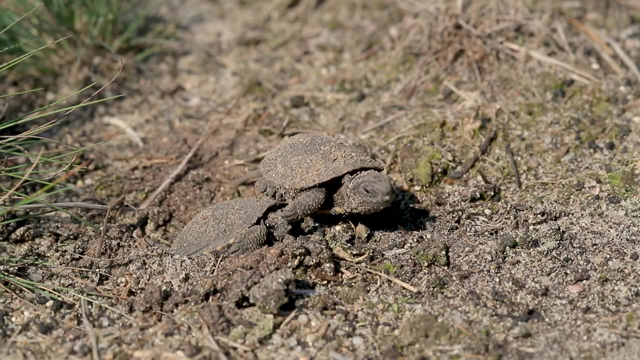 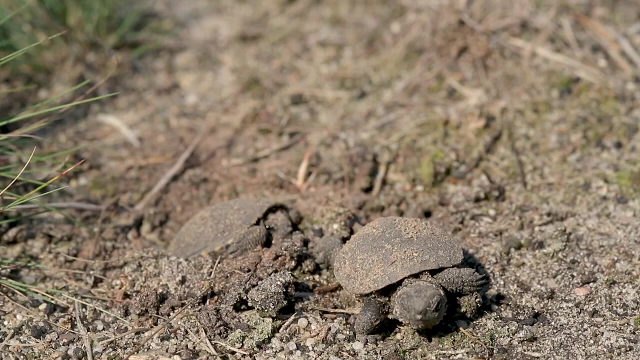 has been accompanied by maximum temperatures, That is, cold or hot weather conditions. At typical temperatures, which are not abnormal, males are born Baby turtles that start out on their own, still have a completely soft shell. They often fall prey to predators. 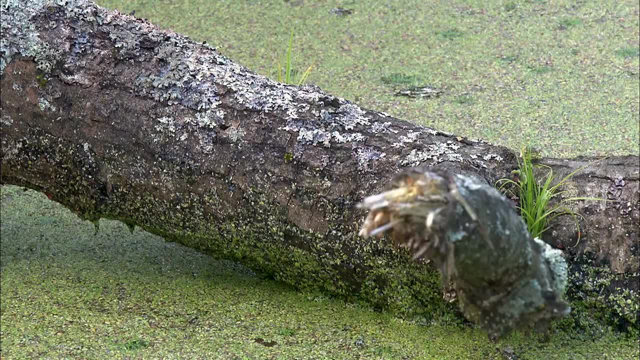 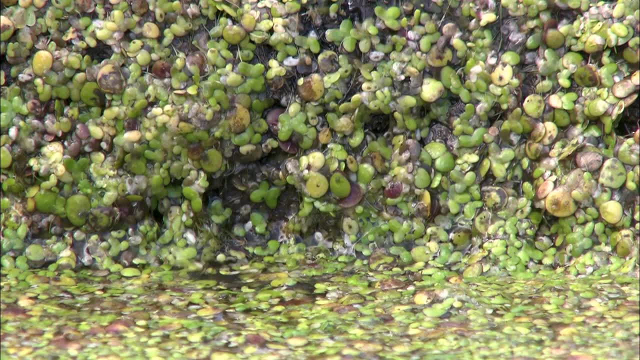 For example, solitary fish mammals, water birds and even large beetles such as the great diving beetle. Larger turtles are prey for foxes, wolves, raccoon dogs, otters, black storks, grey herons, white-tailed eagles and pikes. 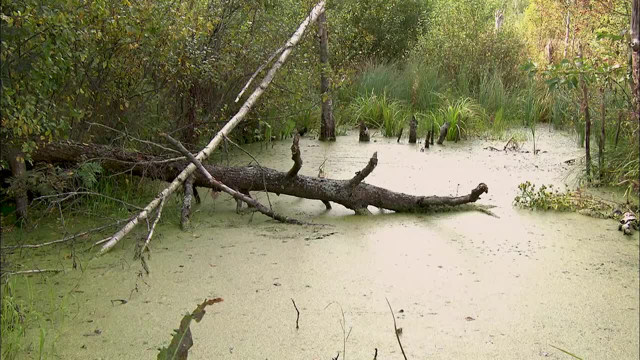 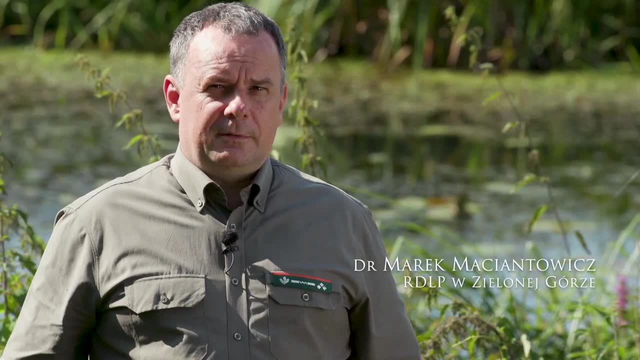 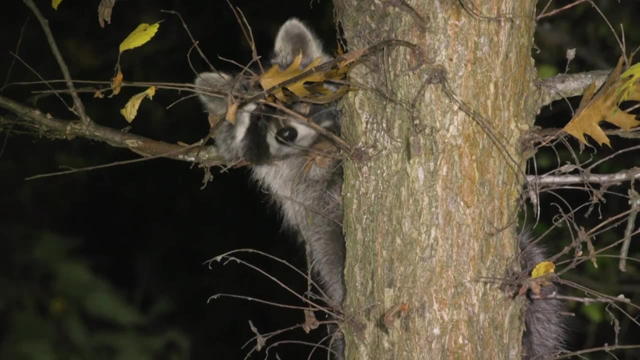 Therefore, they like to find shelter in wet alder forests and drainage ditches. A major threat in western Poland is the appearance of the common raccoon. This is a species that has started to appear in Poland for some time. It is expanding from the west towards the east. 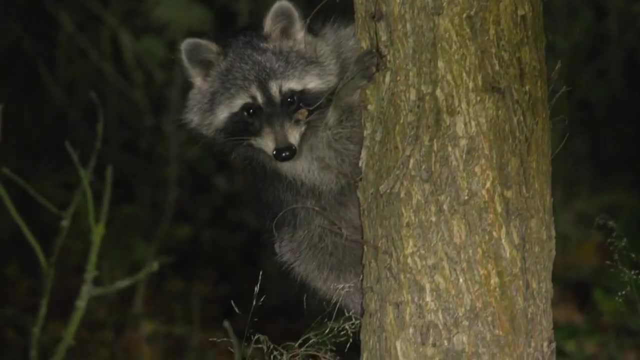 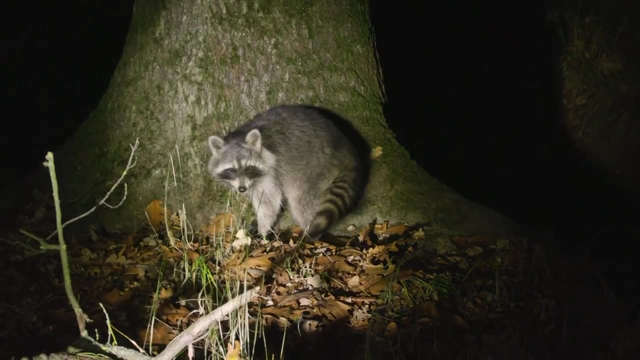 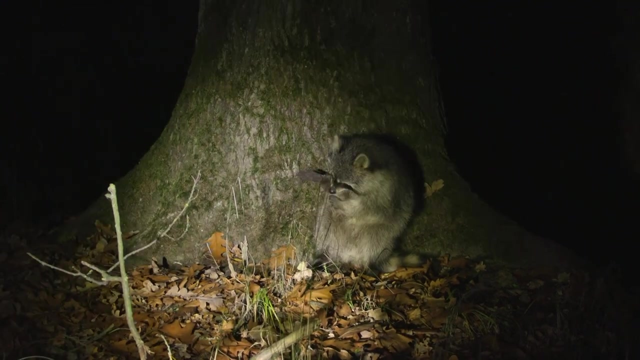 This is a problem, as the common raccoon is an animal that feeds quite intensively and can penetrate different environments. In Germany there have been observations that raccoons can tear the shells of adult turtles and slowly this species is becoming a big problem here in western Poland, for example. 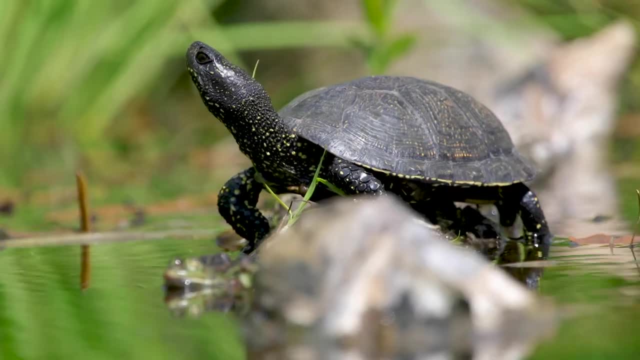 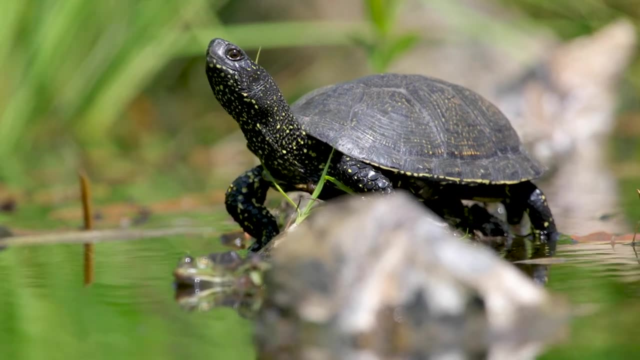 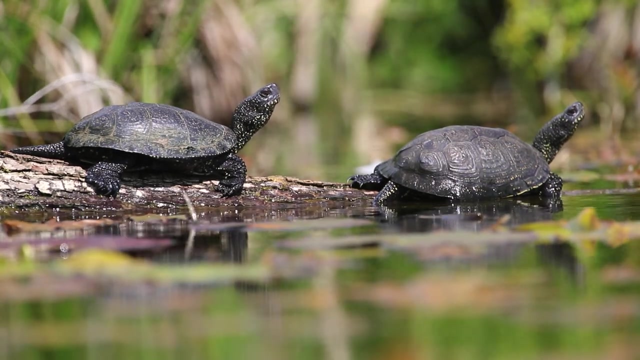 The European pond turtle is most active in the mornings between 8 and 11 am and in the afternoons between 2 and 4 pm. During this time, they usually bask on land. At night, however, the turtles do not come out of the water at all. They feel best at temperatures between 18 and 31 degrees Celsius. 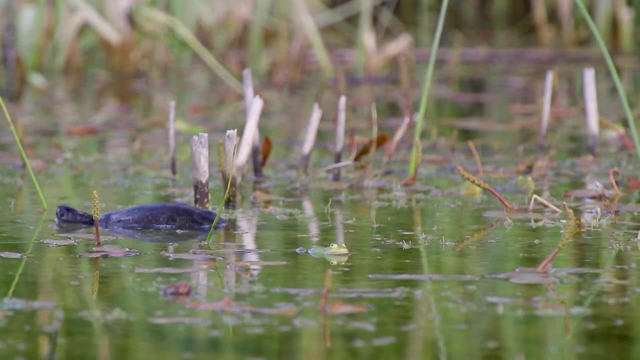 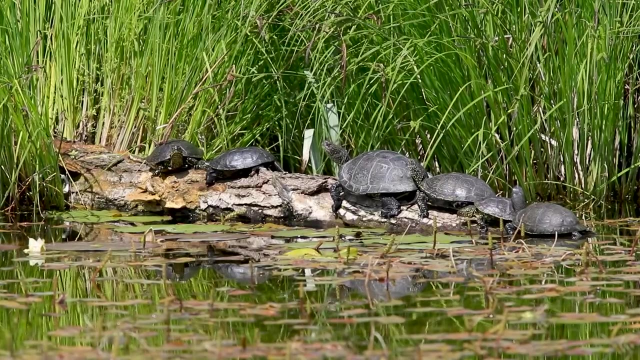 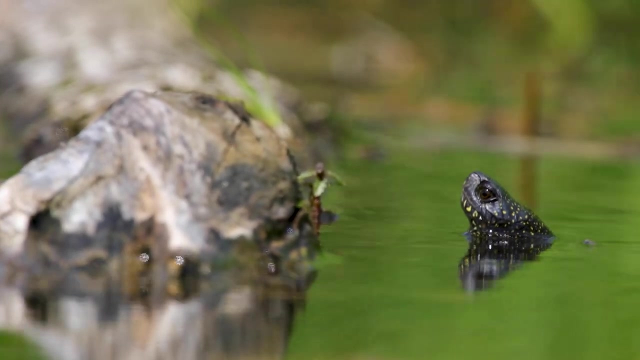 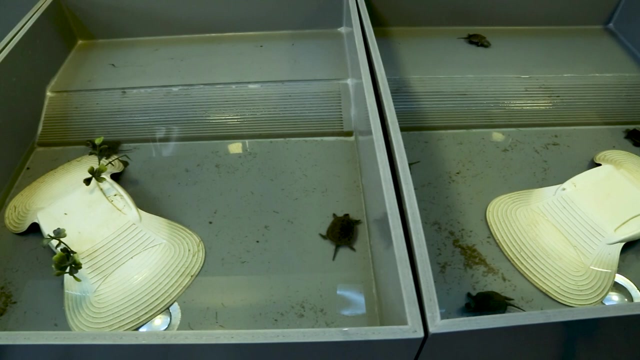 And when the temperature exceeds 37 degrees celsius, the turtles overheat, so they enter into the water at temperatures above 34 degrees celsius. Breeding of young individuals is one of the elements of active conservation of the species, especially where populations are scarce and threatened with the loss of stability. 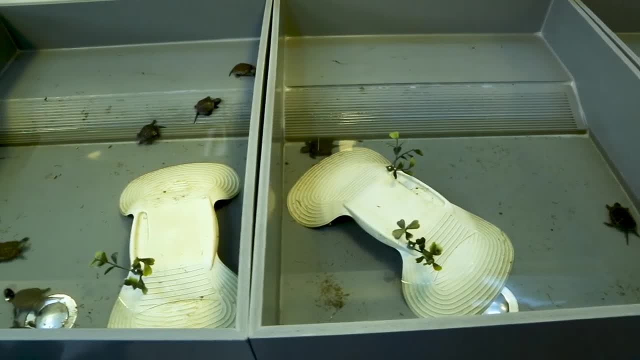 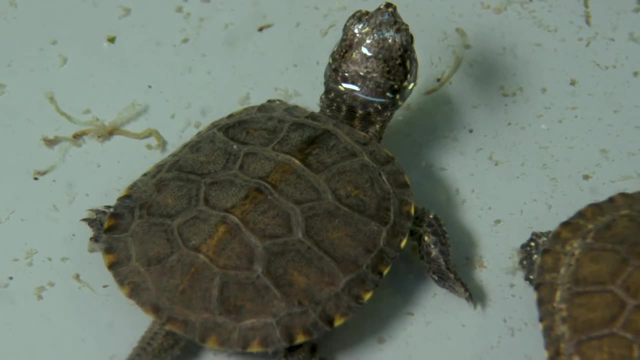 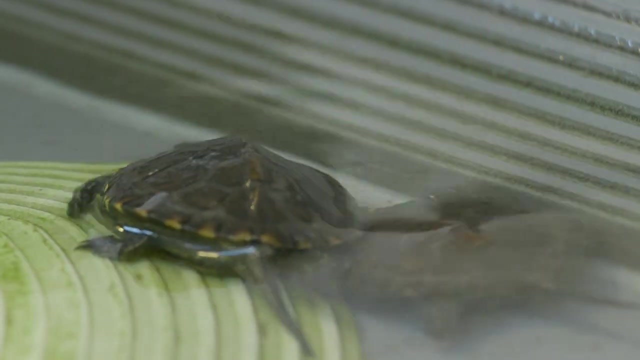 Turtle breeding programmes have been carried out since the last, a long time ago, 1980s. The main goal of these activities is to increase the chances of survival for young individuals in the first year of life. In Poland, breeding takes place for one year. In some European countries it sometimes takes two years In this way. 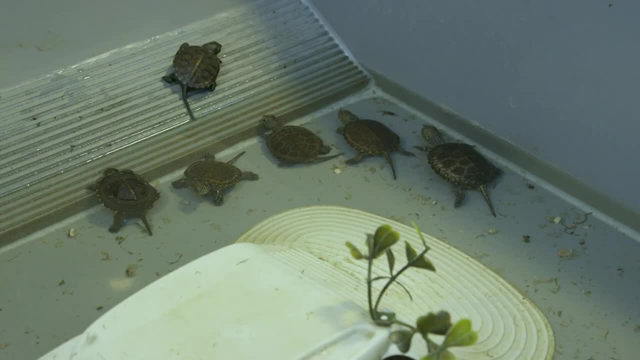 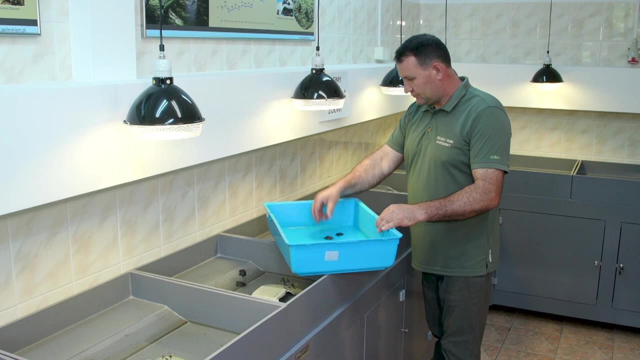 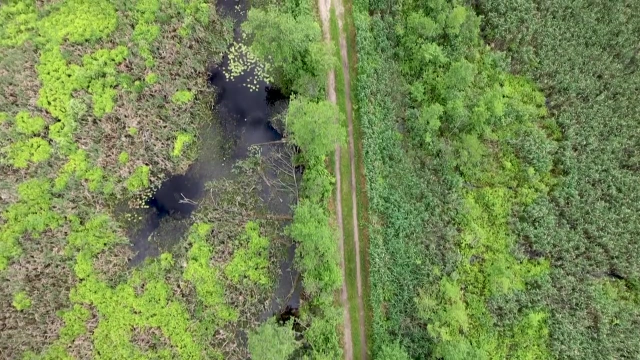 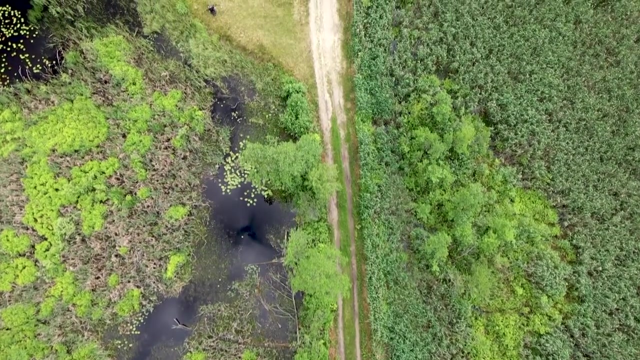 during the critical period of life, young individuals remain beyond the reach of predators. Under artificial conditions, the survival rate is approximately 90%, According to the current scientific approach. the method of protecting the European pond turtle by digging up and incubating the eggs should be used only. 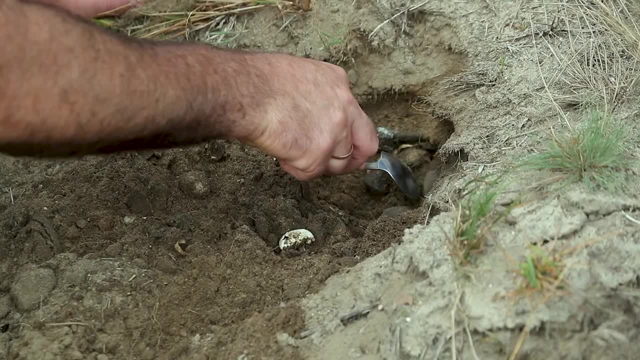 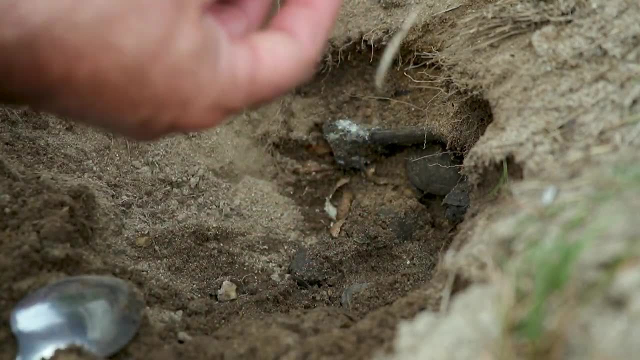 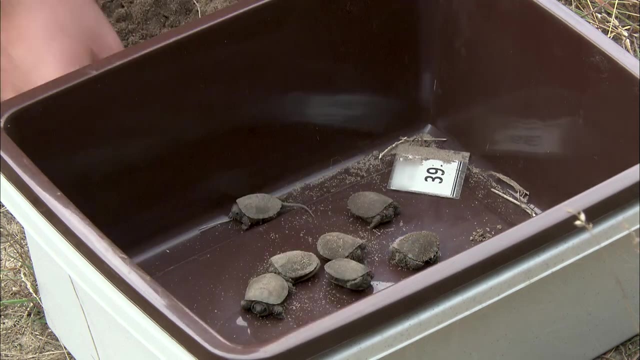 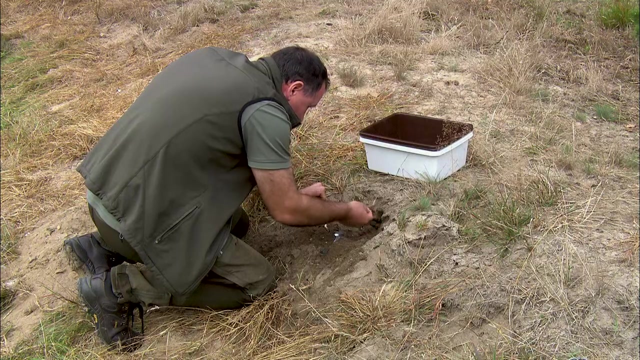 exceptionally, when the female lays her eggs in a place where they are highly endangered, that is, by agricultural works. One of the first European pond turtle breedings in Poland was carried out in Kraków by Dr Maria Zemanek. Between 1990 and 1996, a total of 160 young 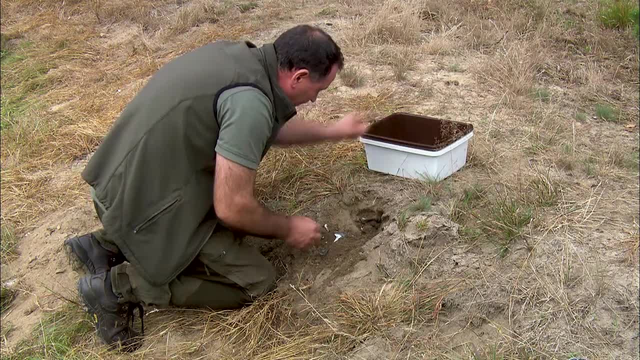 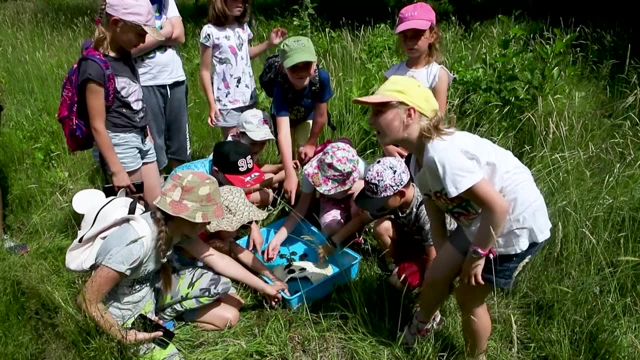 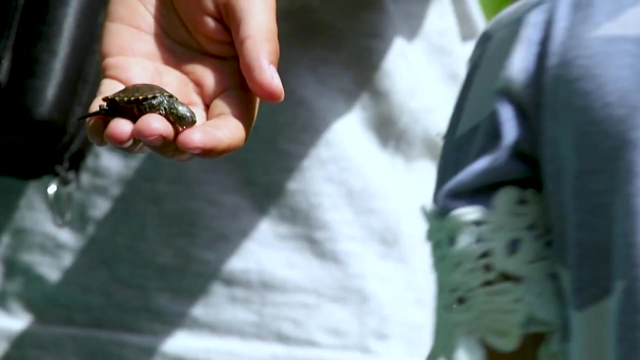 turtles were released in the then Radomvoy Vodeship and by the year 2000 this number had increased to 439 individuals. In Polesie National Park there has been for a dozen or so years the European pond turtle protection center, which deals with, among other things, the 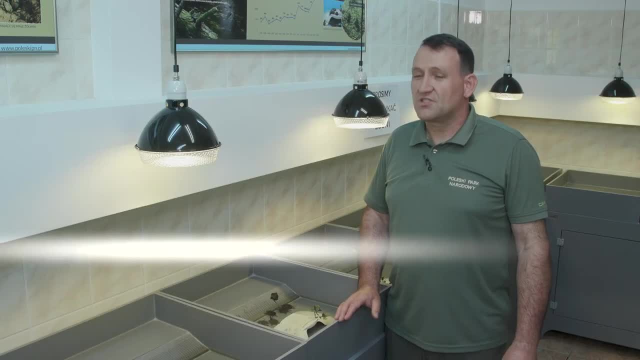 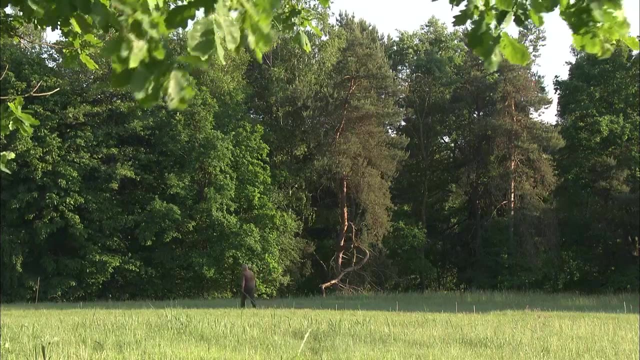 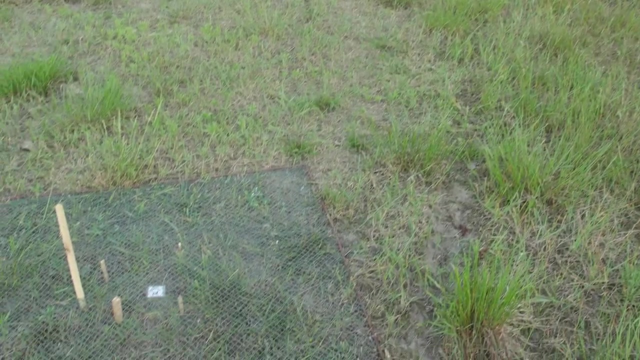 breeding of young turtles. During this period, we have released more than 20,000 young animals. We have protected over 2,000 deposits with nets against predators. Annually, more than 2,000 young individuals have been hatched in recent years. 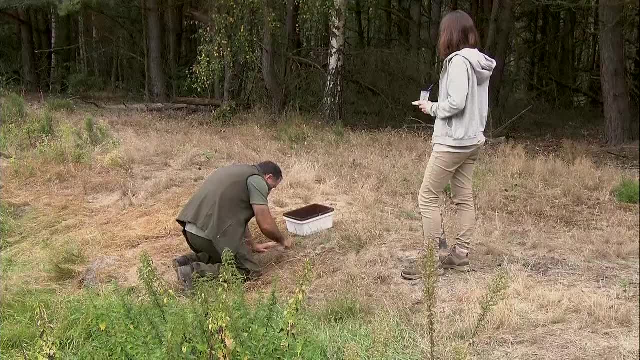 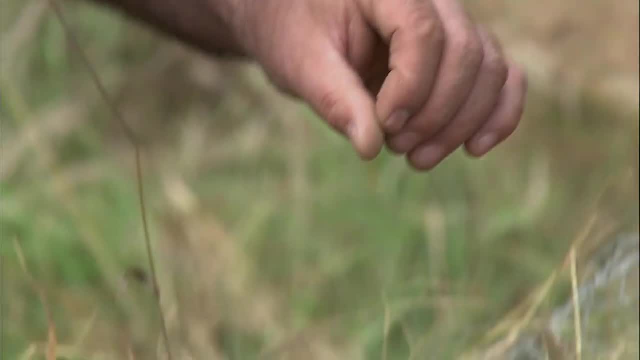 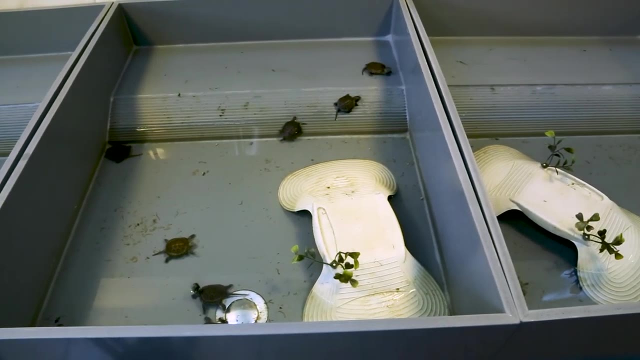 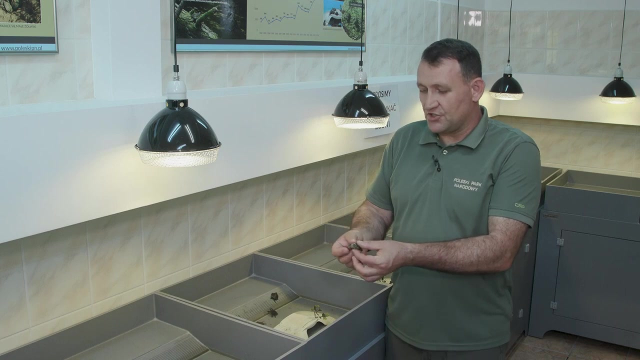 Most of these turtles are released immediately into natural bodies of water in the autumn and some of the turtles that hatch latest or were incubated were brought to the center here. There is such a small proportion, around 300 animals a year. These individuals spend the winter here and are fed. Special conditions are. 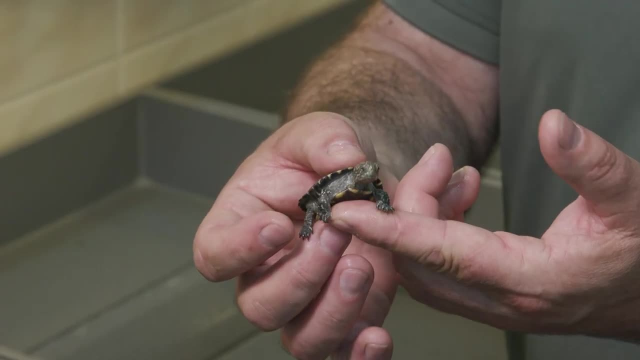 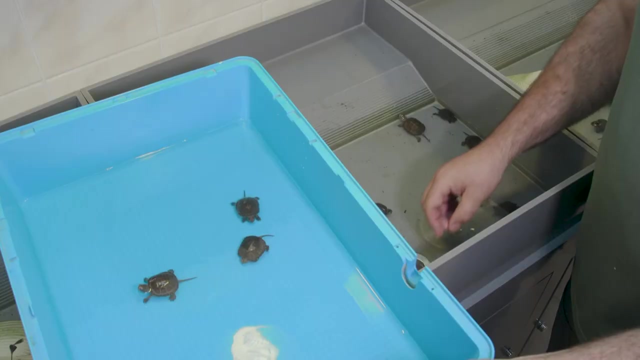 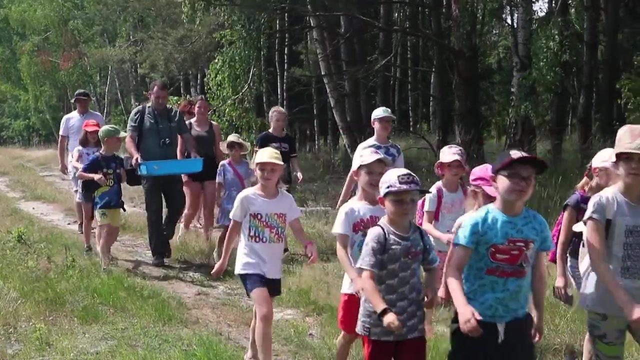 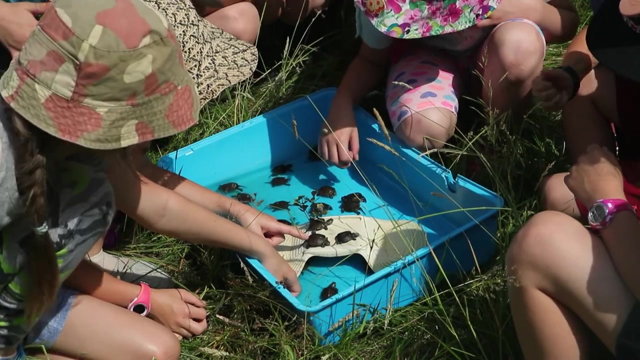 created for them here, and they are released in spring. As a result of active protection, 440 young one-year-old turtles are added to the local population between 2000 and 2001.. The total number of released juveniles is approximately three and a half thousand. in Poland There are six breeding sites in. 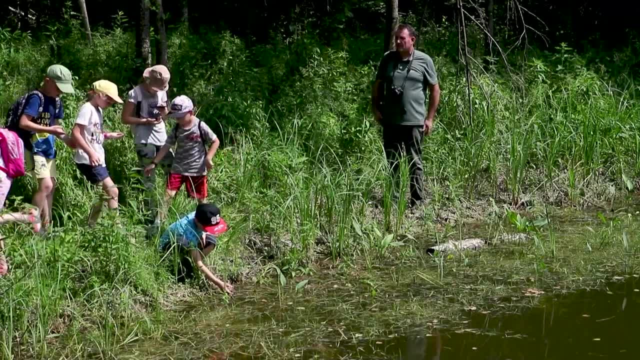 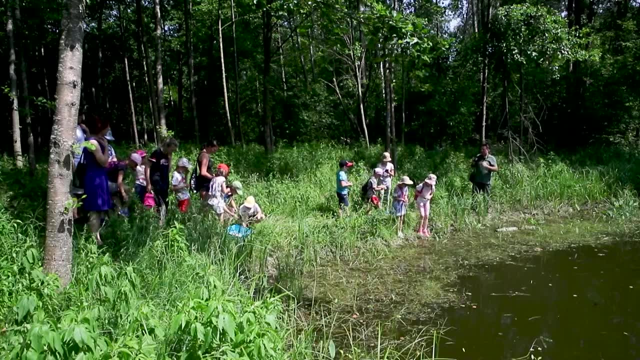 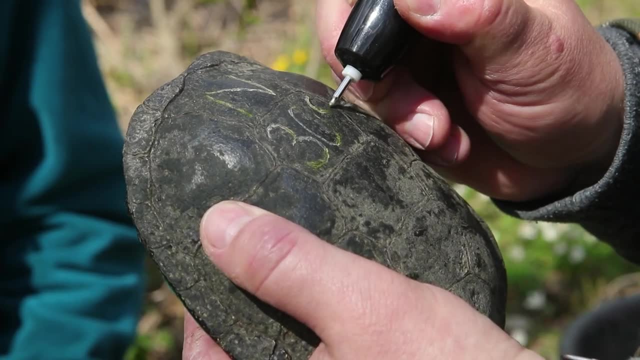 Polesie National Park, where females go out to breed and lay eggs, secured over 241 females since 2017. to date, they are marked. This allows us to know exactly when they lay, whether they move from one site to another. We also know that there are double hatches within one year and we have 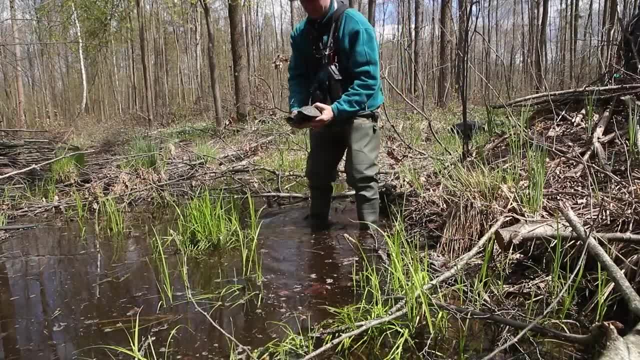 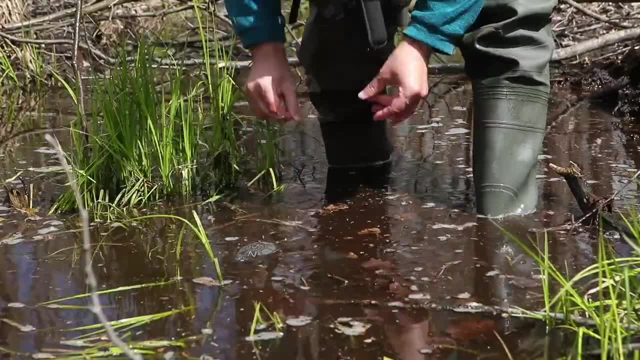 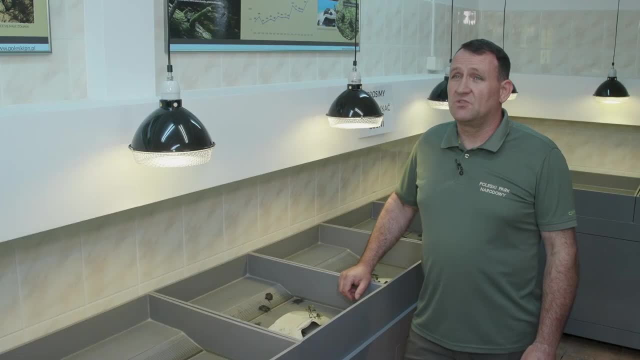 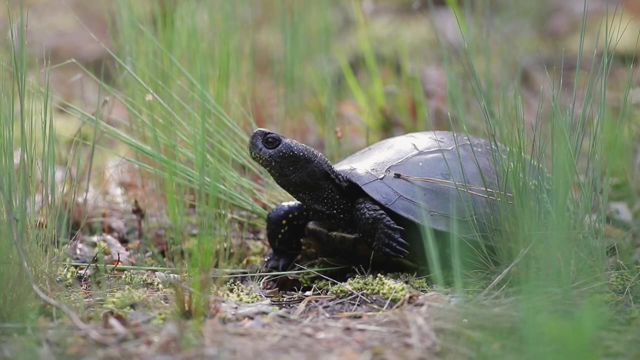 precisely this kind of full quantitative monitoring of these protected deposits. Funding for active protection of the European Pond Turtle in Polesie National Park comes from various sources. These include the National Fund, the Provincial Fund for Environmental Protection and, in recent years, the Coordination Center for Environmental Projects. 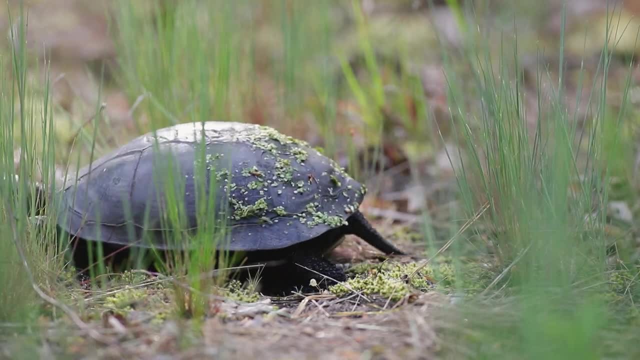 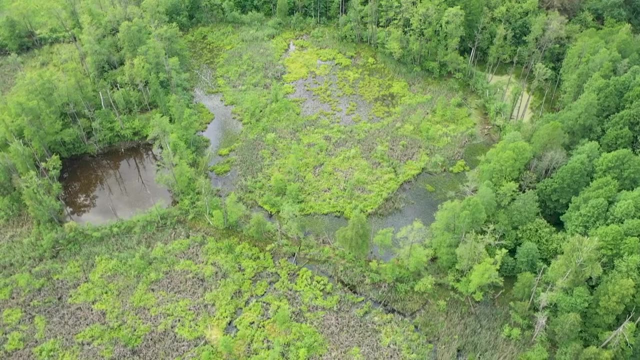 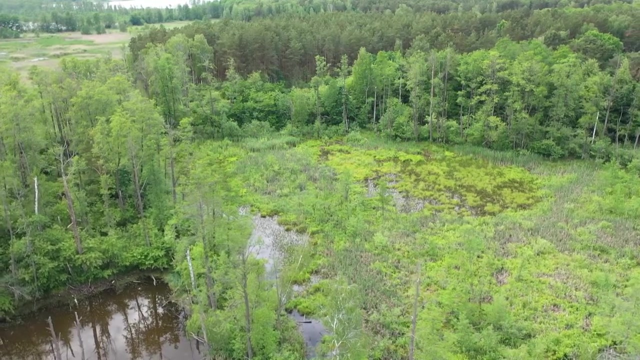 We are currently implementing a five-year protection program which will be financed by CCEP for two more years. All active protection in Polesie National Park is financed from these sources. Habitat degradation is currently the greatest threat to the species' existence throughout its entire range. 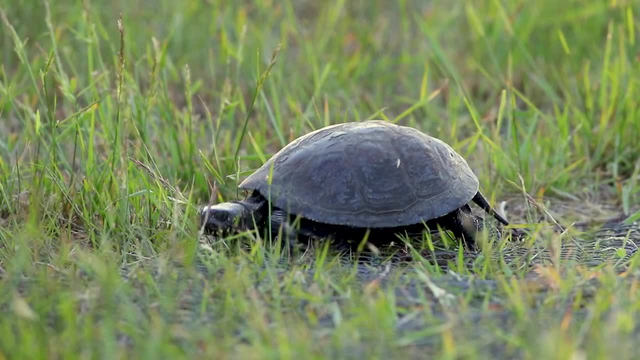 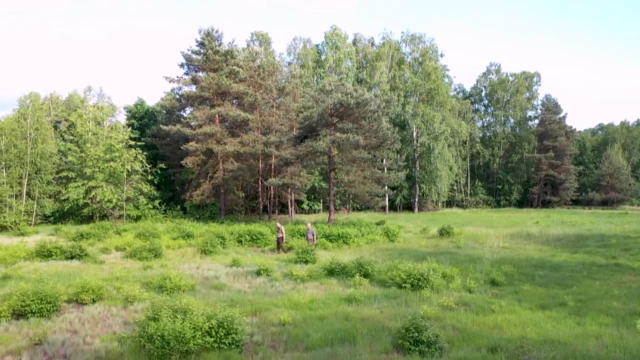 Particularly unfavorable changes have taken place in the highly industrialized countries of Western Europe, where the species' range on the continent has decreased by leaps and bounds. In Poland, the disappearance of biotopes in which the European Pond Turtle lives is also very rapid. 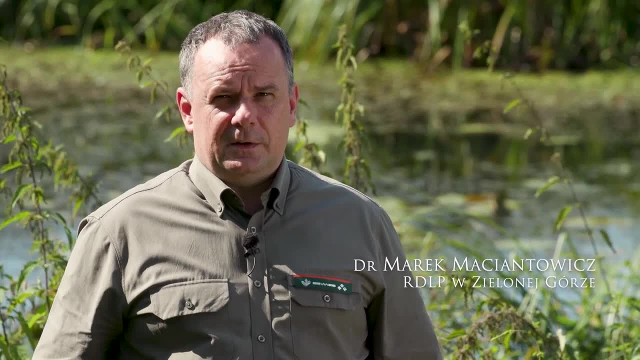 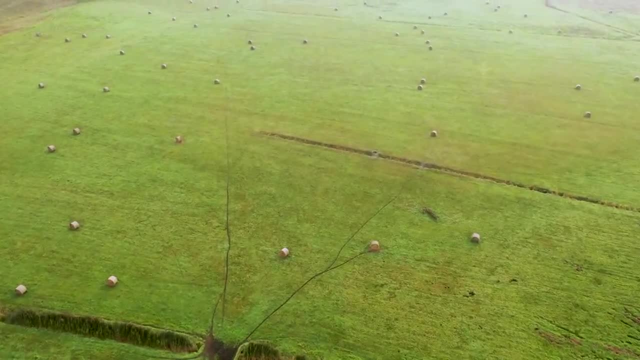 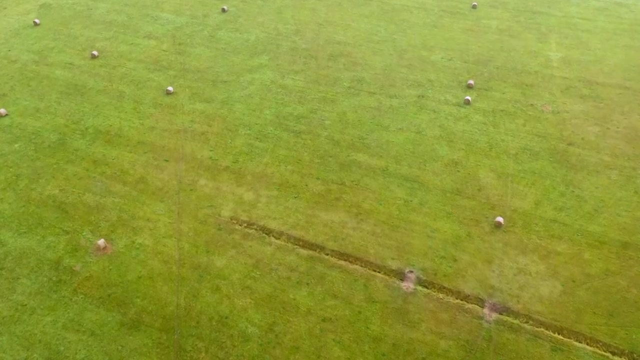 One of the most important threats is the loss of habitats, falling groundwater levels and generally drying up of reservoirs. In the post-war period, the slogan making wastelands productive was promoted, which meant draining marshes and peat bogs In the western part of the country. post-German devices regulating water levels were destroyed. 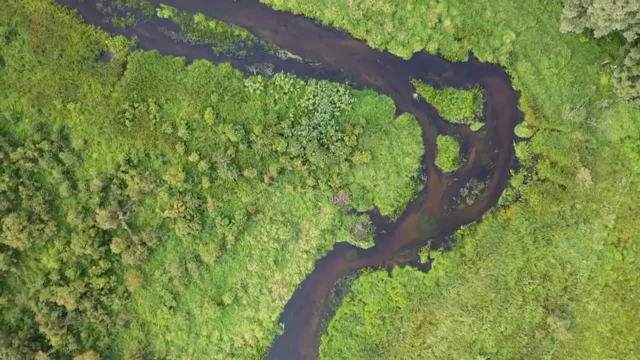 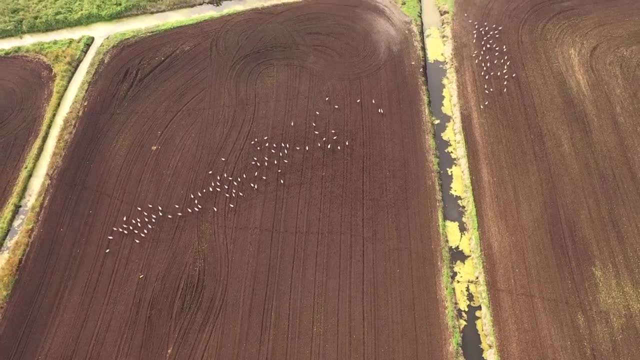 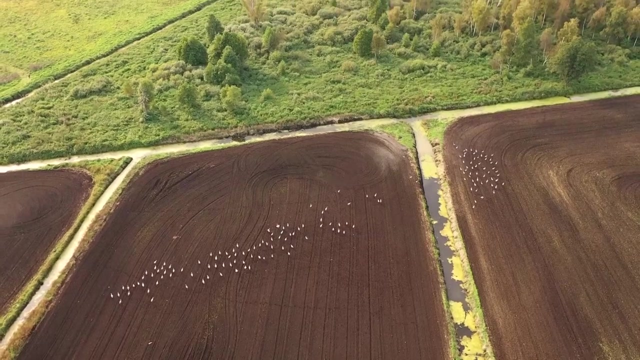 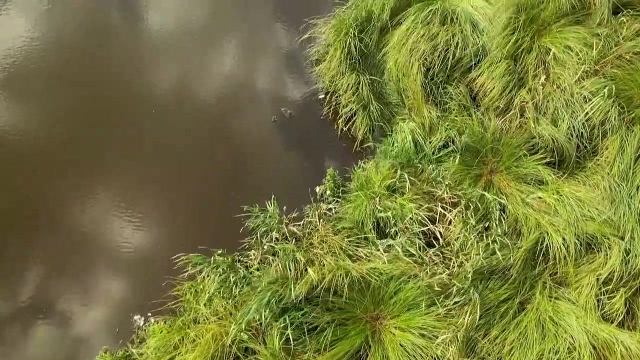 This resulted in significant degradation or disappearance of wetlands in large areas. The greatest impact on habitat degradation has been exerted by the draining of marshes, the regulation and construction of rivers and the devastation of habitats associated with human activity. One of the contributing factors is also water pollution by sewage. 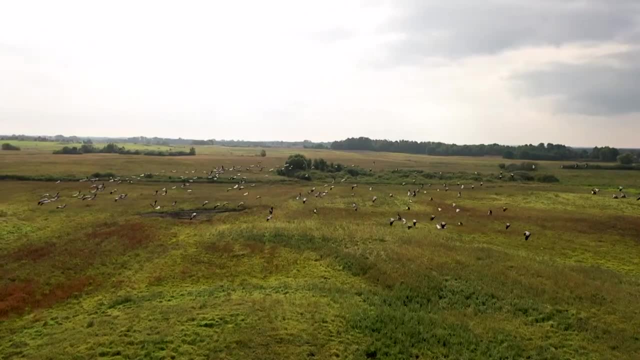 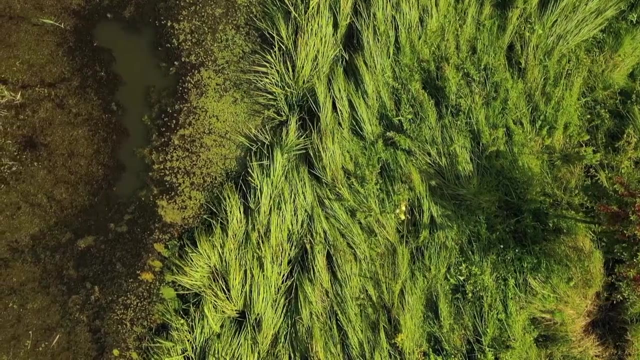 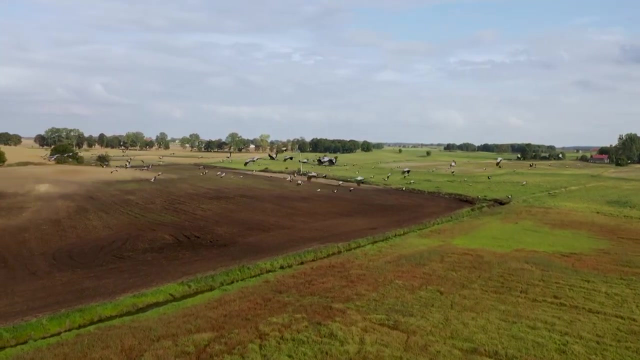 The use of increasing amounts of fertilizers in agriculture, especially potassium and nitrogen fertilizers, results in their increased flow to lakes and small midfield reservoirs, increasing their fertility. This results in the creation of anaerobic conditions, accelerated overgrowth and shallowing of reservoirs until they completely disappear. 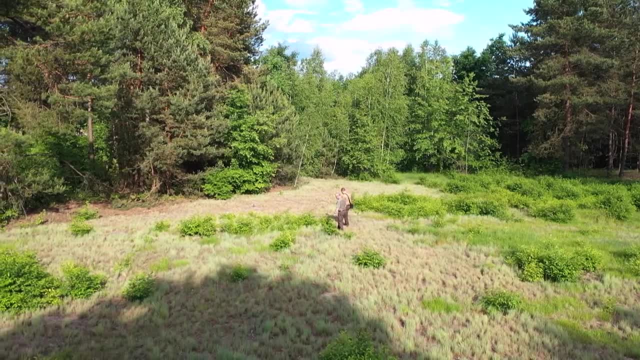 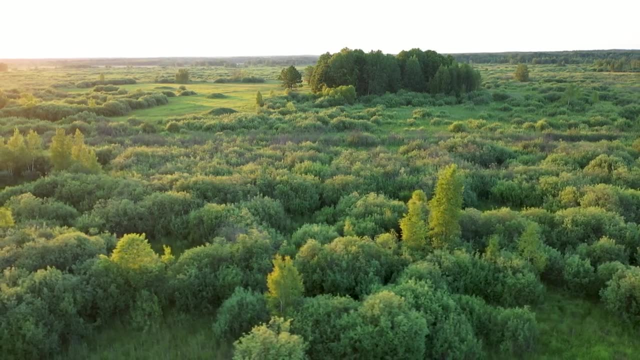 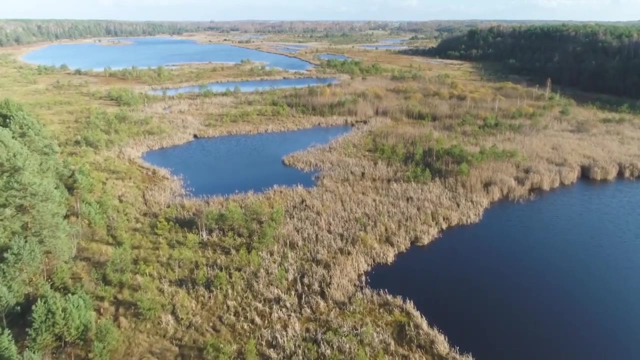 Another serious problem is the disappearance of breeding grounds. It is caused either by natural succession of small seeded species – pine, birch and black locust – or by planned afforestation. In the latter case, the land manager is usually unaware of the fact. 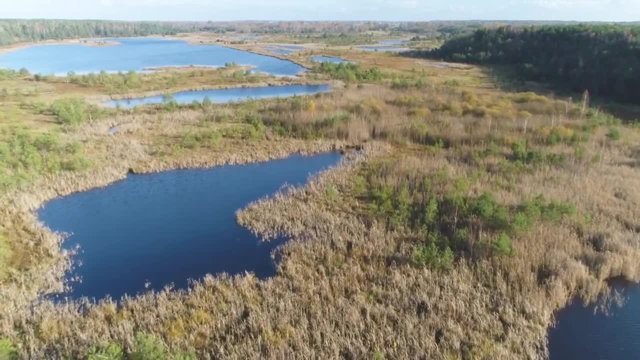 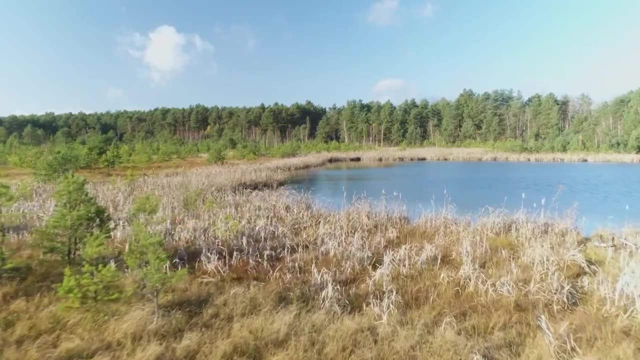 that a dry hill or grassland is a long-term site for laying eggs and is extremely valuable from the nature conservation point of view. The land manager is usually unaware of the fact that a dry hill or grassland is a long-term site for laying eggs. 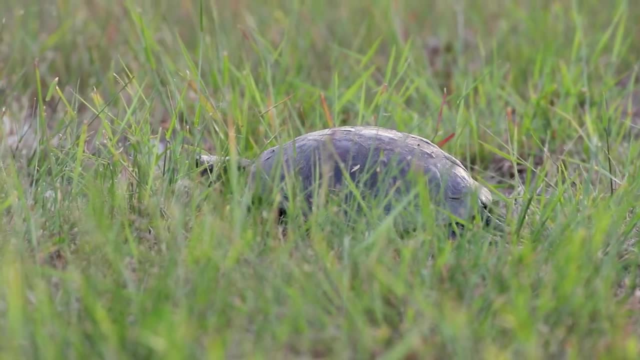 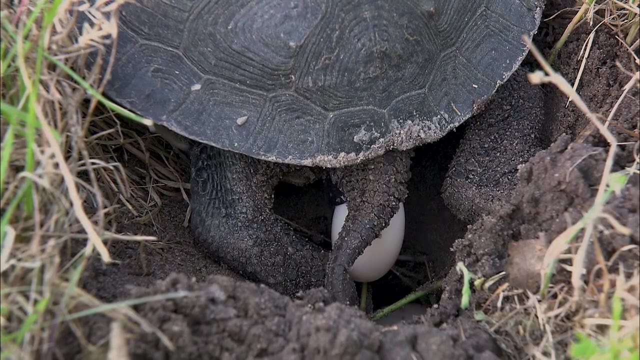 and is extremely valuable from the nature conservation point of view, A European pond turtle breeding site, One of two in the Żółwiowe Włota Reserve. You can see from these nests here that the breeding season has already begun. The turtles come out to this area lay their eggs. 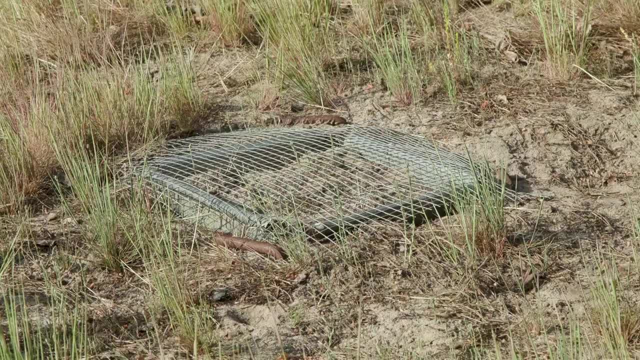 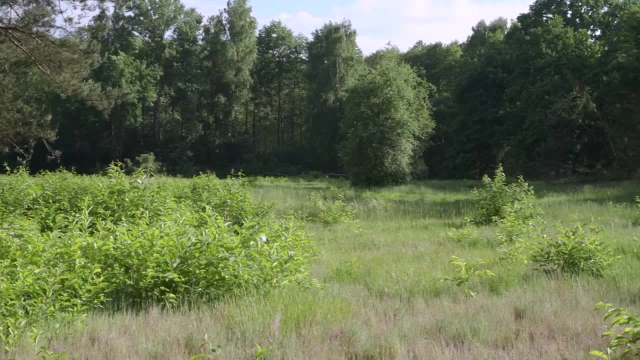 and then people protect them so that predators don't destroy them. On the other side of the nests we see, unfortunately, the wild black cherry tree. Back in the 1980s there was a field here. Foresters sowed rye and other cereals all over the area. 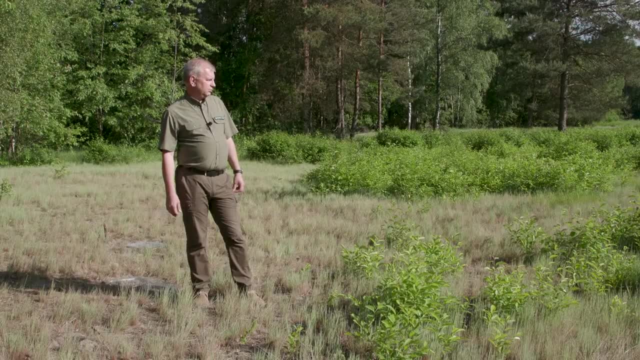 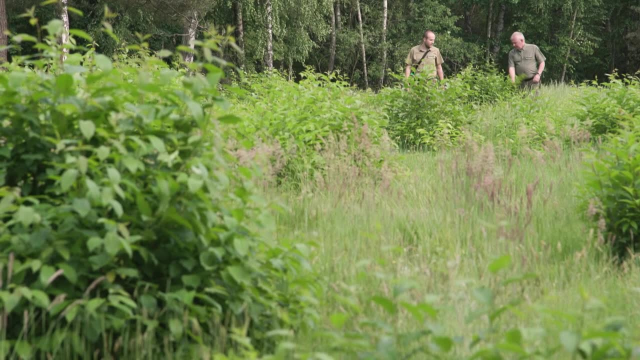 and the turtles laid their eggs here. Now, unfortunately, no one cultivates the land. there is a reserve here and the black cherry does not ask if it can grow and grows as it pleases. When it grows bigger it will shape the places where the turtle eggs incubate and it will 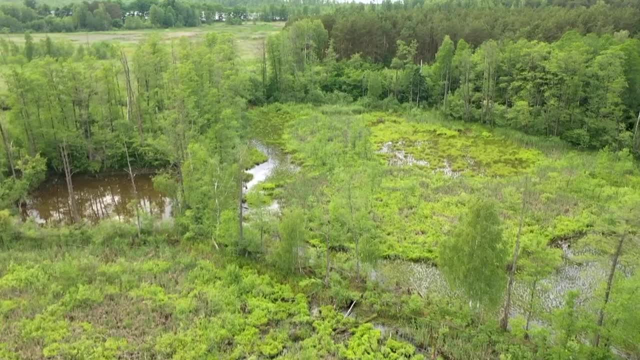 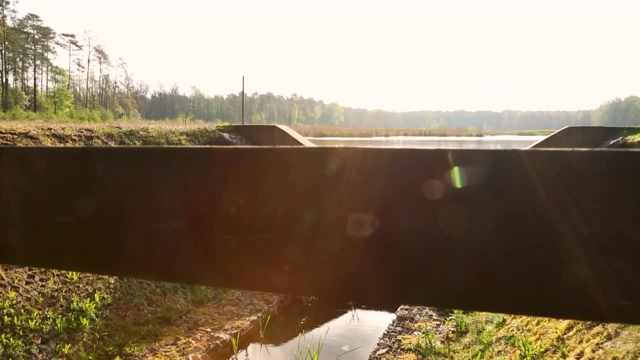 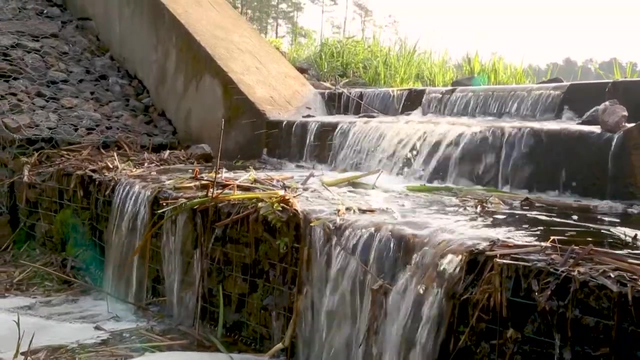 have to be cut down and left outside the reserve. The most important measure that shapes turtle habitats is stabilizing water levels. The most effective method is the construction of various types of water facilities that slow down or completely stop the outflow of water from the water bodies. 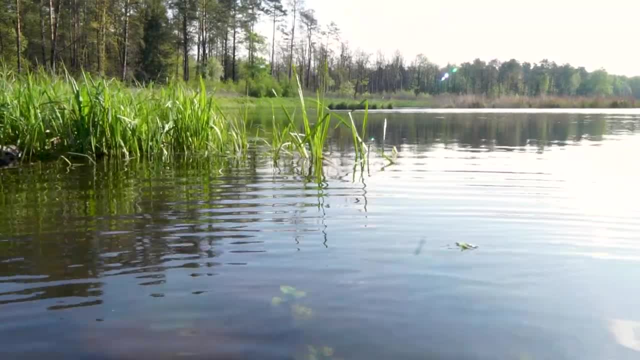 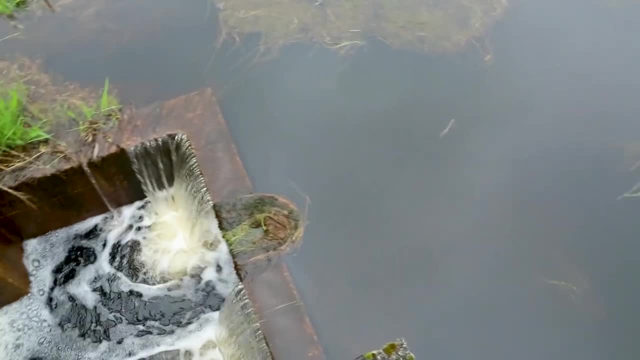 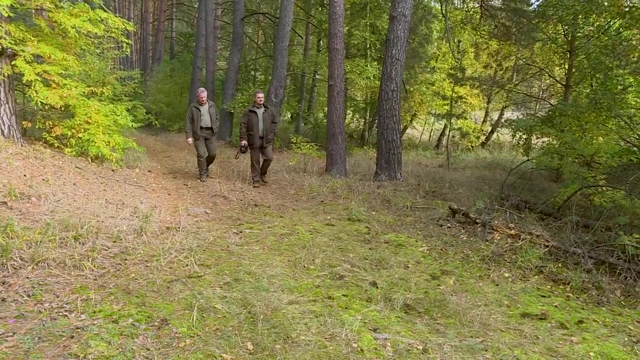 On the adjacent ponds. it is important to keep the dikes, as well as the monks in the dikes, fully operational. This maintains sufficient water throughout the summer period. If existing sites are threatened, alternative habitats are sometimes created, for instance by digging new bodies of water to which the turtles move after a certain time. 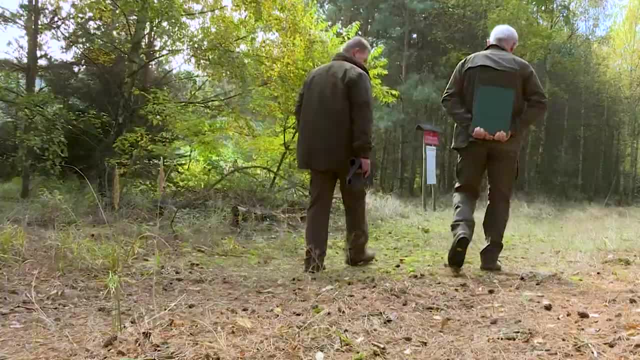 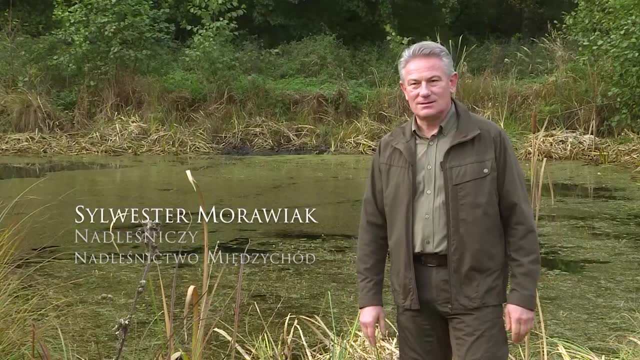 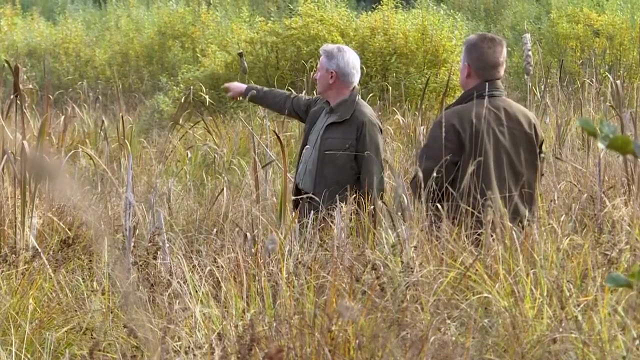 We are on the area of Międzykult Forest District in the Żmijowiec Forestry. This area is now an ecological utility bagienko zamieślin. The ecological utility itself was previously a wasteland. 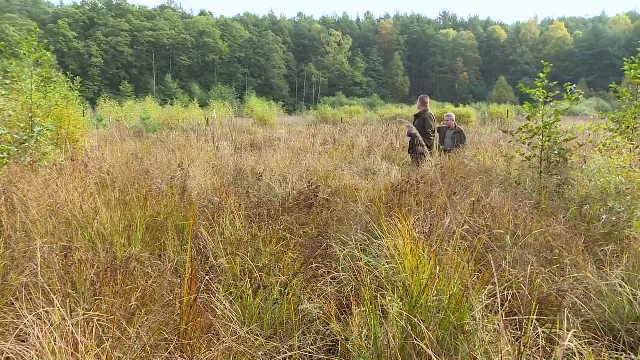 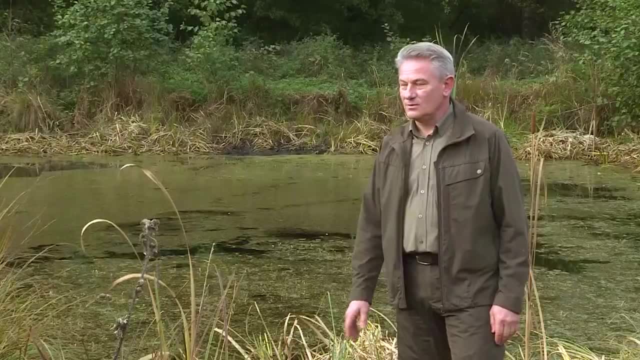 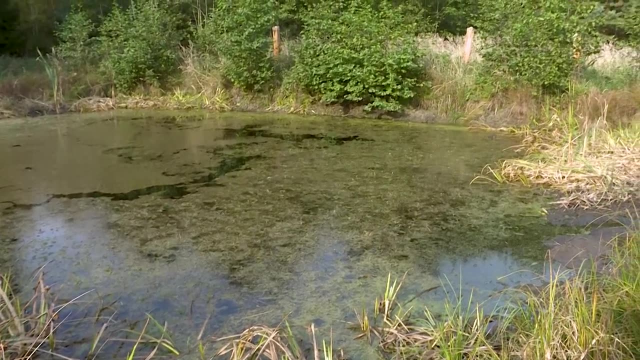 It was only when the first individuals of the European Pond Turtle were observed in 2007 that we started to take an interest in it. that is, to maintain the existing conditions and improve them. We created an artificial water reservoir to stabilize the water environment. 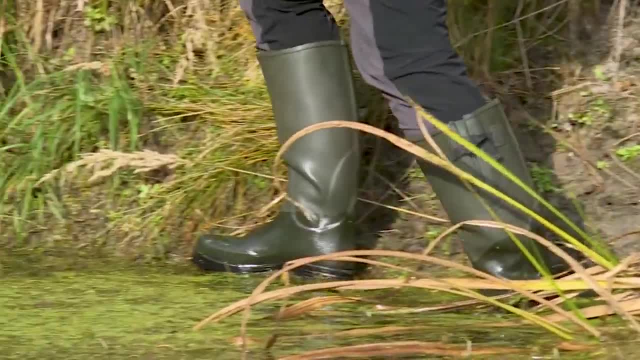 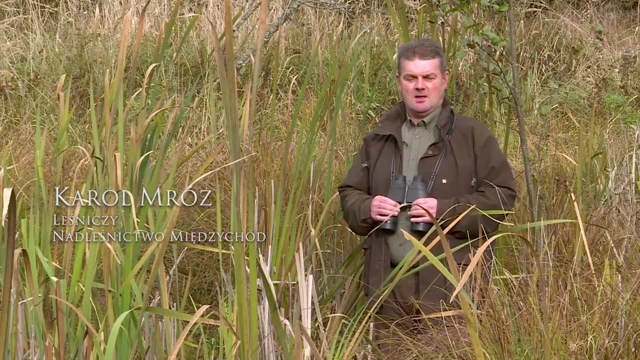 The whole genesis of the discovery of this place was not entirely accidental. A hunter- the now deceased head hunter of the local hunting club- had just reported that while staying here on the hunting box, as he called it, he often saw stumps moving. 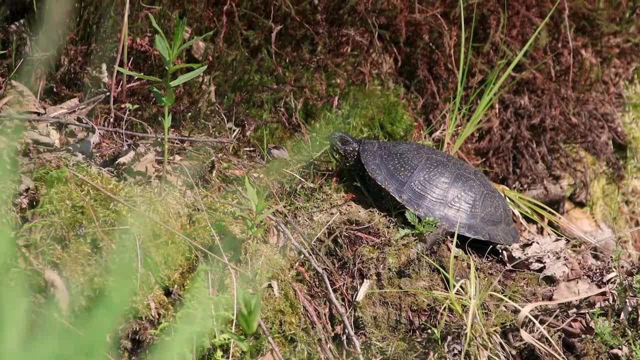 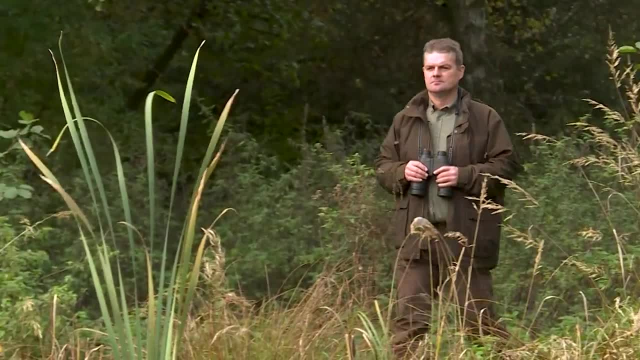 This information gave me much to think about and I decided to confirm it. In the spring of 2007, I was marching along this bog and at one point I noticed an object that looked like a German helmet- a German military helmet- and I decided to check it. 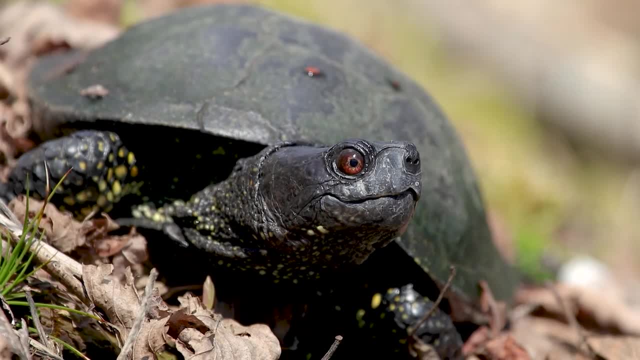 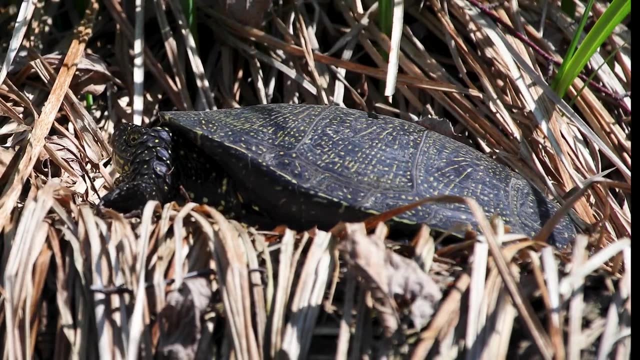 out. I jumped over a clump and it turned out that it was not a helmet, but the carapace of a turtle which was basking in the spring sun. Over the following years, I wanted to confirm the occurrence of the turtle, so that for 14. 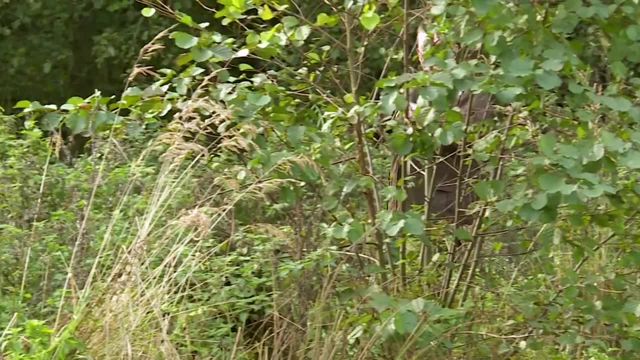 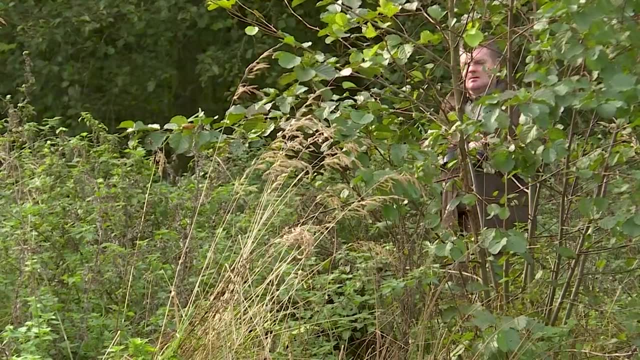 years I managed to find turtles here many times. The turtle is still alive. The turtle is still alive. Even turtles can survive in a trench, especially in spring. On one occasion, the most I managed to observe at the same time in a cluster was three individuals. 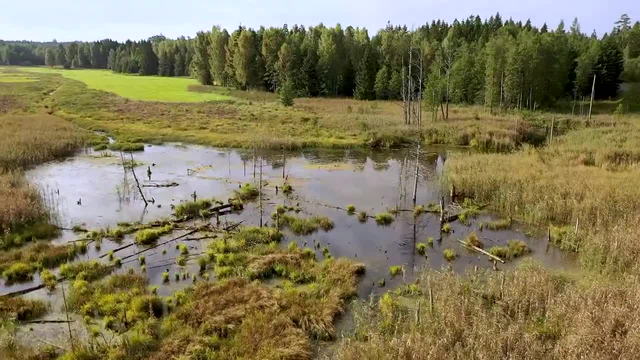 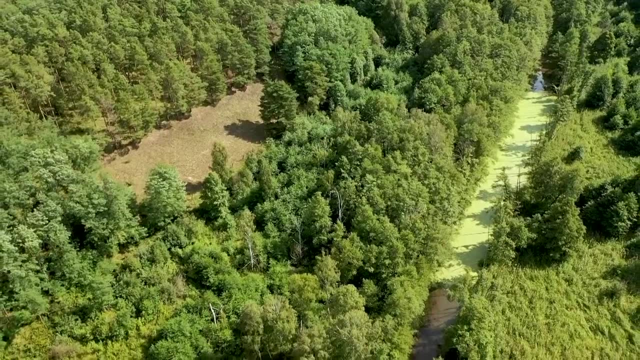 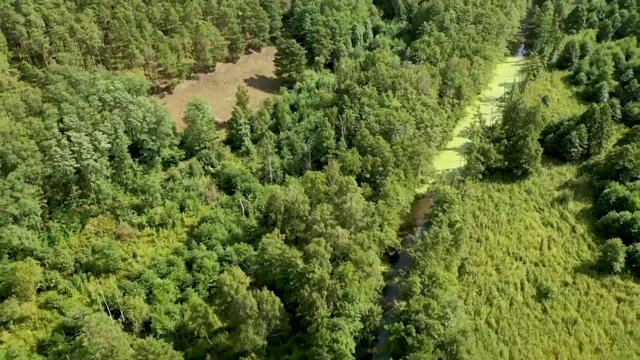 If eutrophication causes reservoirs to become shallow, they can be mechanically deepened. This process can also be prevented by extending the ecotone zone consisting of shrubs and herbs around the reservoir. We hope that the turtle can survive in the trench. 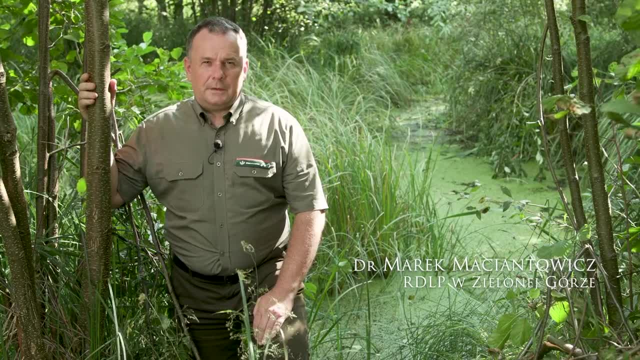 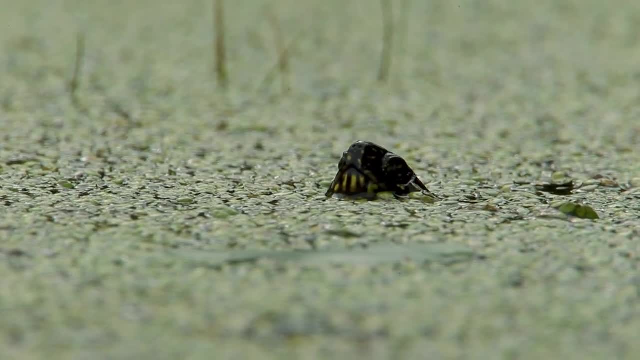 We are within the reserve and Natura 2000 area of Młodno. This is an area of an increasingly overgrown lake, now a peat bog where turtles have been found for many years. There is not a huge population, more like single individuals. 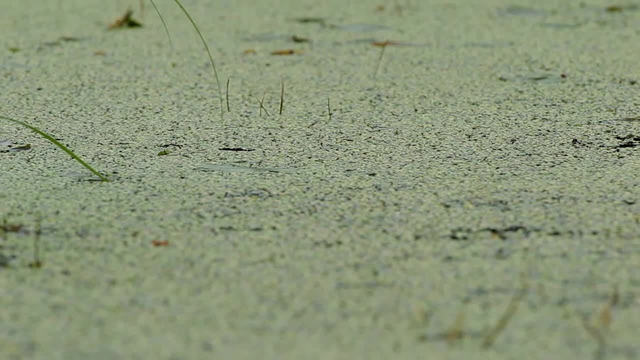 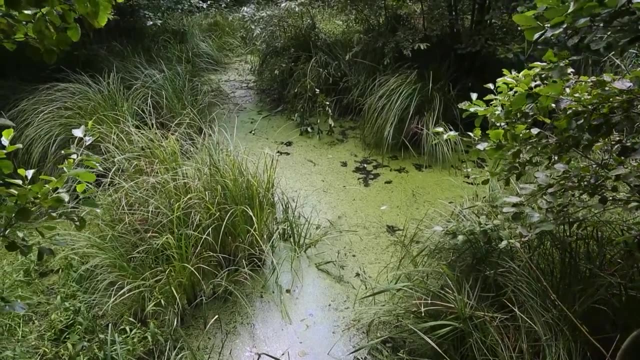 but due to the shallowing of this reservoir, two ponds have been built as part of the Natura 2000 project. We can see that nature has managed very nicely here and it has created an ideal habitat for this species, An extremely important element in the conservation strategy of this species. 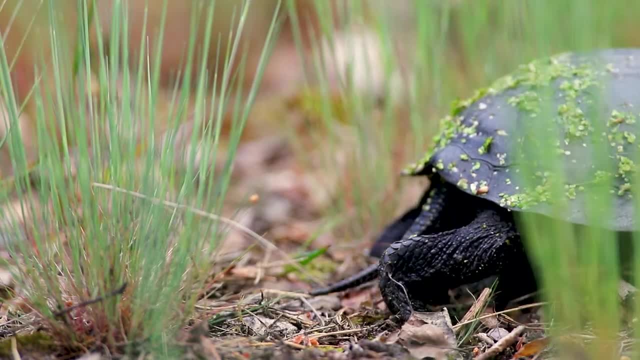 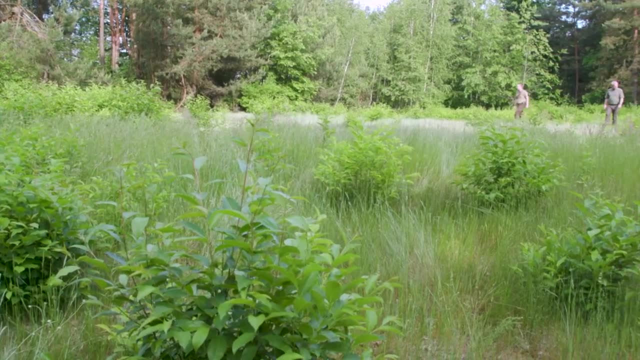 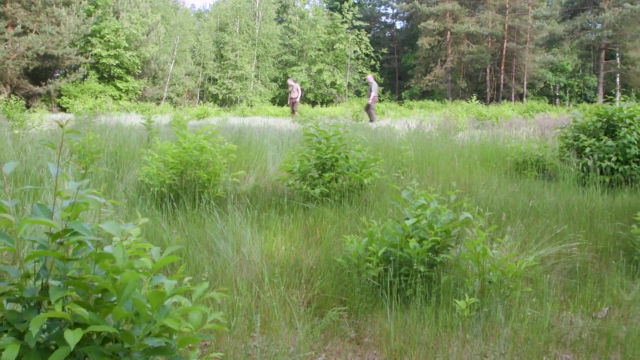 is the care of the breeding grounds. In some cases, it happens that these places become overgrown and lose their functionality. As a result of shading, incubation conditions deteriorate and, in the long run, the age structure of the population may be disturbed. 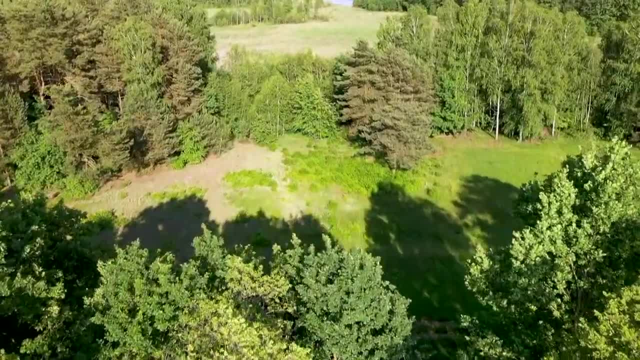 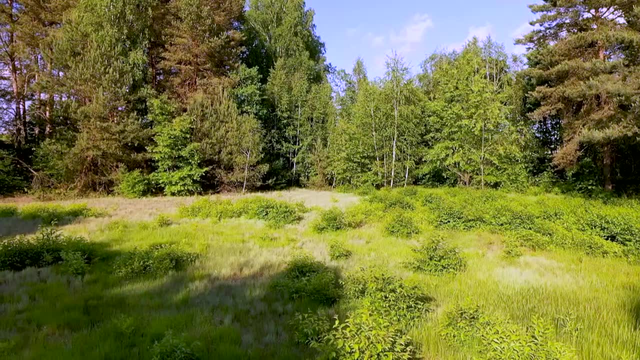 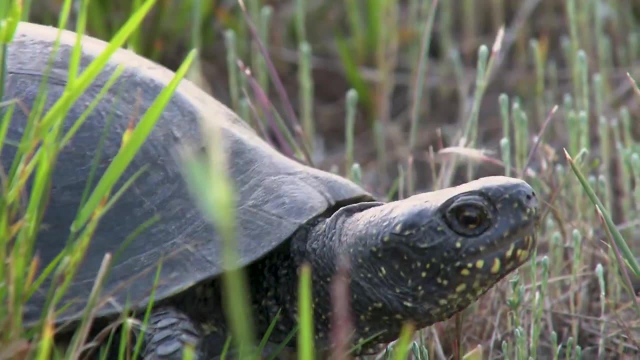 There is then a clear generation gap. Therefore, from time to time, active protection measures are taken by just removing these shrubs and improving thermal conditions on the breeding grounds. Not all trees are cut down, of course, as the females sometimes use the shelter of small trees. 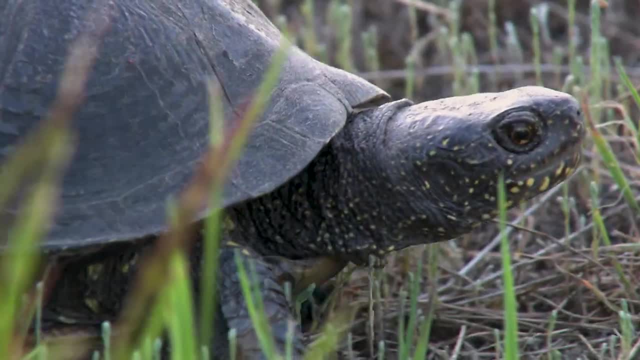 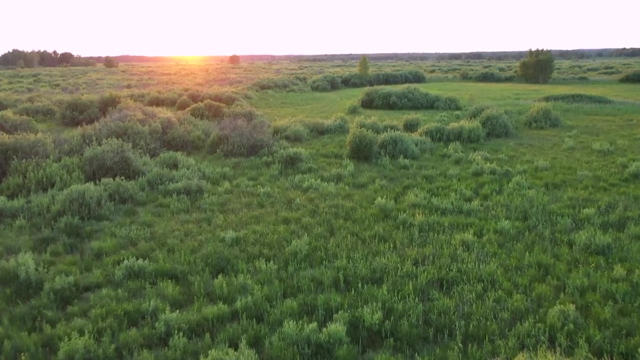 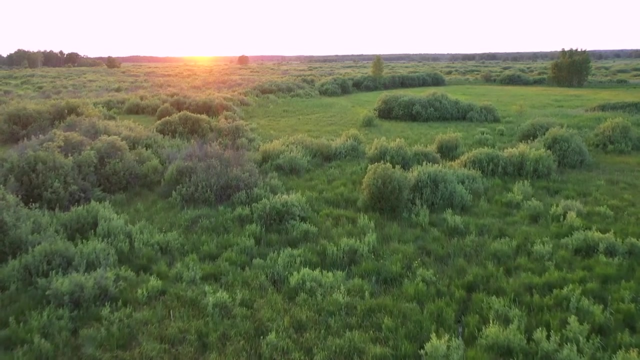 such as pines, while waiting to go out to the breeding grounds. In the case of the European pond turtle, a whole complex of habitats needs to be protected, as the absence of one habitat threatens the existence of the entire pond. The breeding grounds are actually the most threatened. 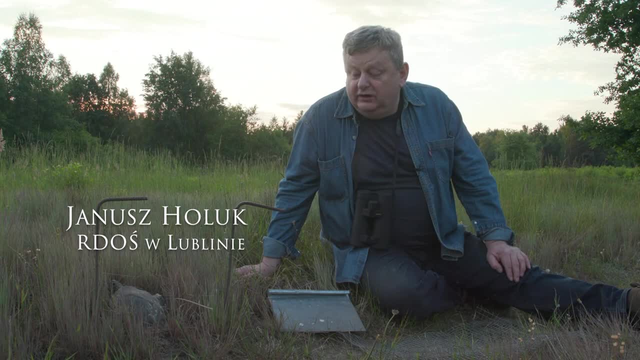 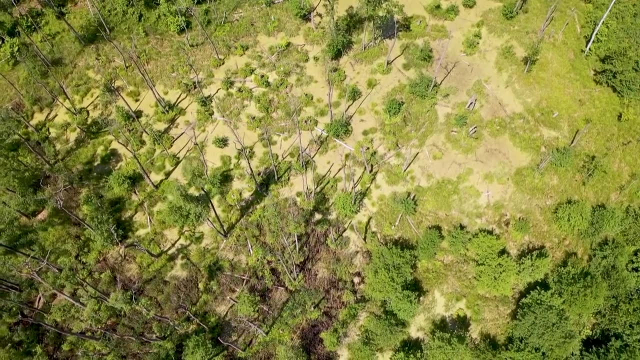 Part of the turtle's habitat is no longer a wetland habitat but the breeding sites. It is in wetland habitats that turtles spend their entire lives. They only go out on dry land to lay eggs, or when the marshes dry up, they move on. 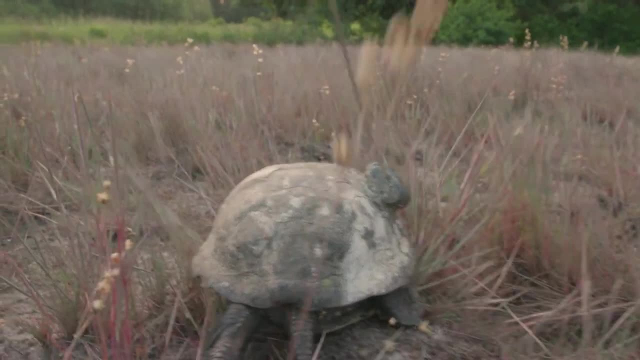 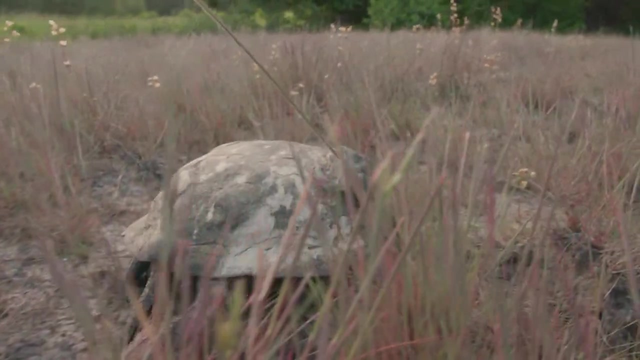 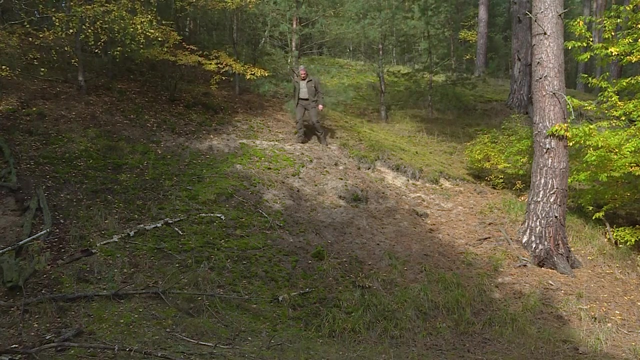 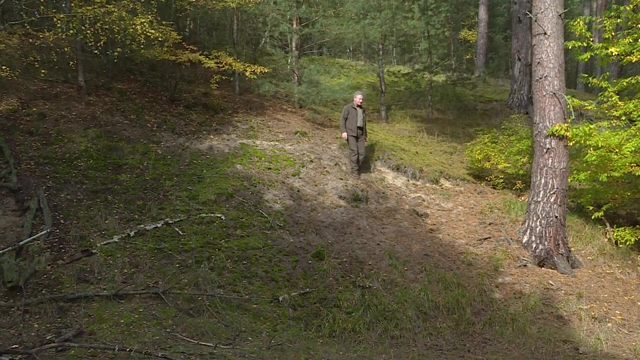 as was also shown nicely in the telemetry studies, Due to the location of a significant number of European pond turtle sites in areas of the state forests, individual forest districts undertake measures to actively protect the habitats of the species in their respective territories. The tasks we set ourselves have been completed. 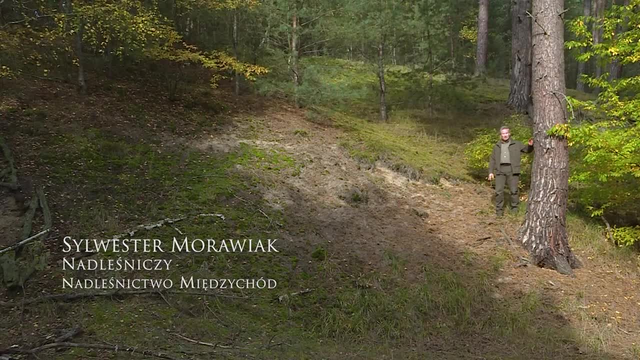 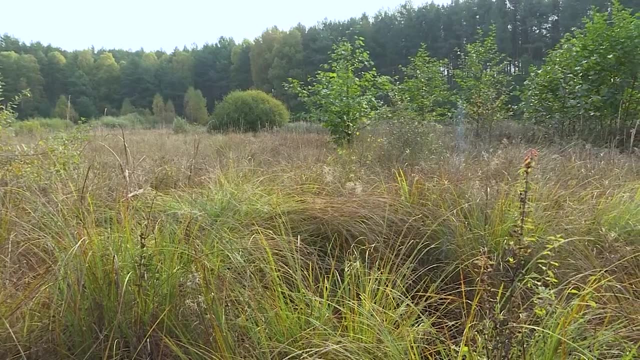 but in recent years, due to the lack of water in the forest- and not only in the forest- this peat bog has begun to dry out and we plan to restore these conditions in the bog itself. We also came up with the idea to create conditions. 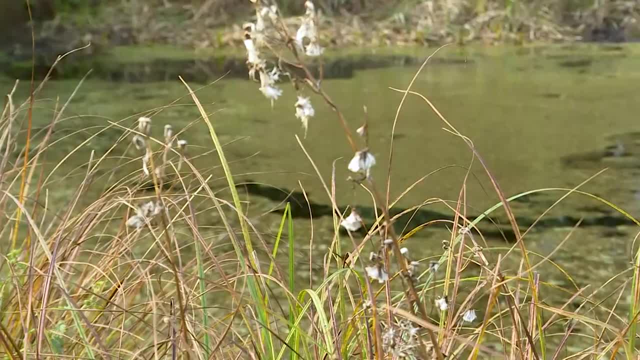 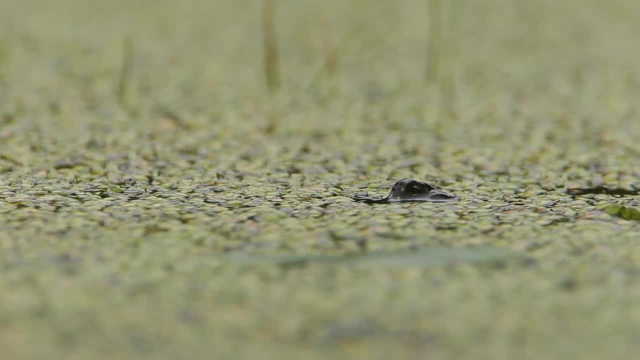 for the turtles to have somewhere to procreate as well. This is a very good exposure, a southern exposure. Following consultations with specialists and after our plans have been approved, we would like to make this place much more exposed so that there would be plenty of light. 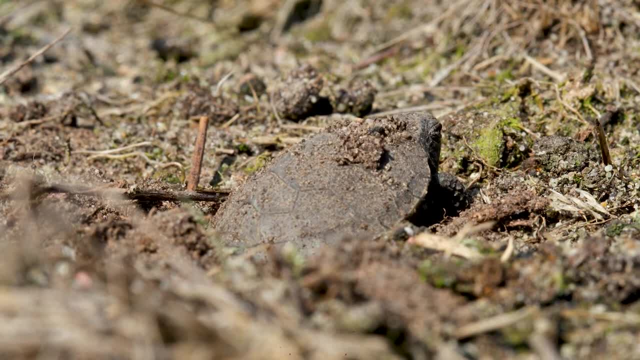 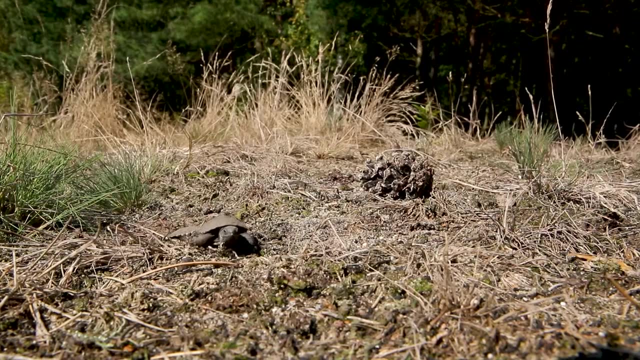 and at the same time we would also like to do something within the peat bog itself. The direction is to maintain at least open water reservoirs. as the result of the fall of water, There is less and less water in the drainage ditches. 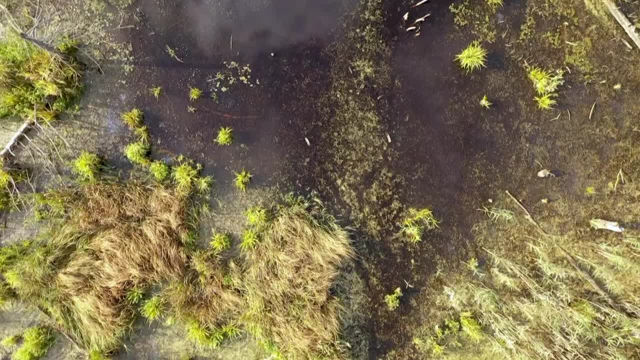 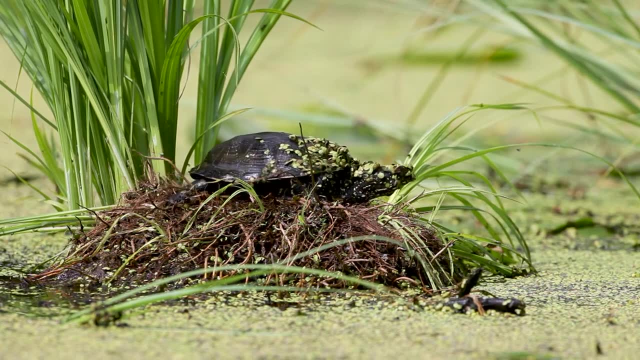 but, looking at the deteriorating conditions, we are also planning to restore and build another reservoir. It will be connected by a ditch to the existing one, and this will be an element which will allow us to think that the turtles will not lack water here in their natural environment. The season of falling into winter numbness begins with the first frosts at the turn of September and October. Turtles usually overwinter at the bottom of water bodies buried in a thick layer of organic sediment. There have also been observations of turtles overwintering. 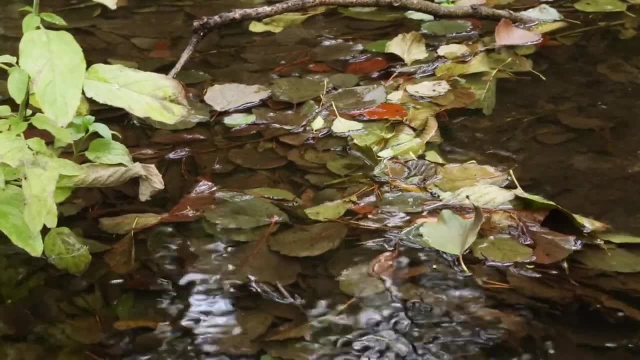 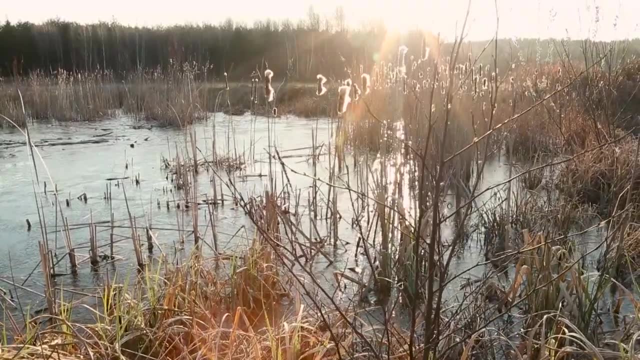 in shallow water among fallen alder leaves, in reed beds, sedge beds and boggy mud. In sporadic cases they overwinter on land. Turtles usually overwinter in the same water bodies where they have been throughout the season. 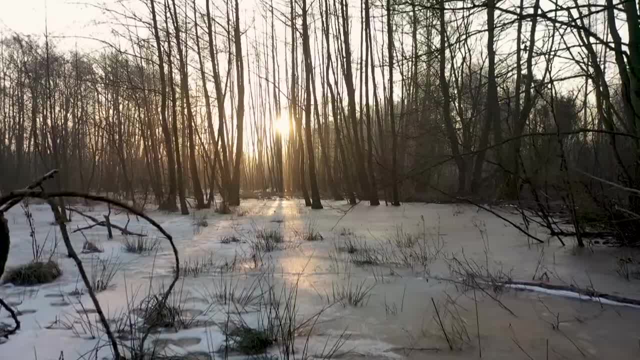 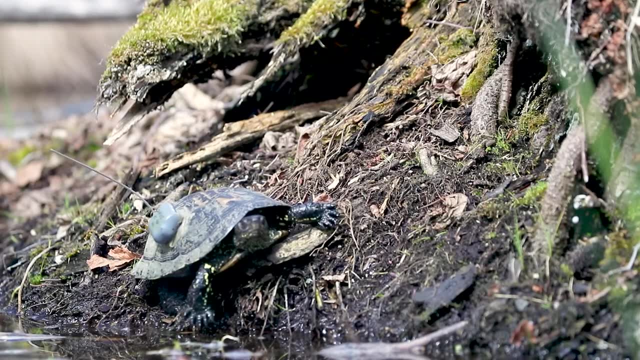 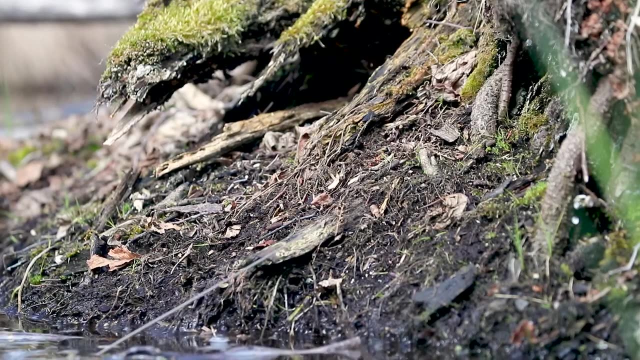 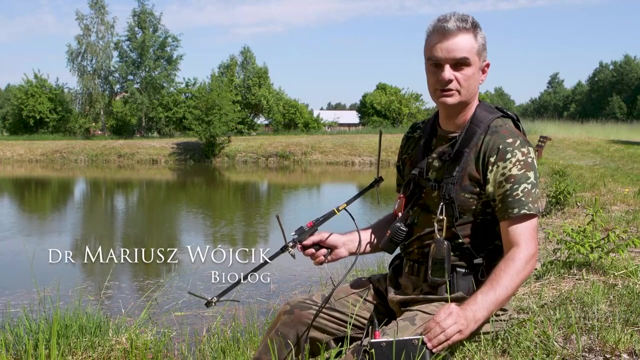 Sometimes, however, they migrate to other places. It is not known why this happens. Most information on overwintering sites has been obtained through telemetry studies, as transmitters also send signals from underwater. Each turtle has its own distinctive transmitter, so once the receiver is activated, 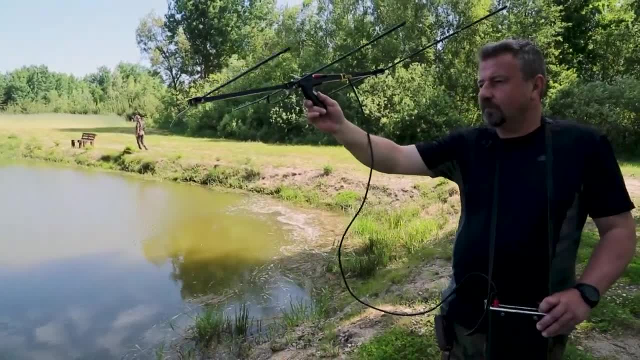 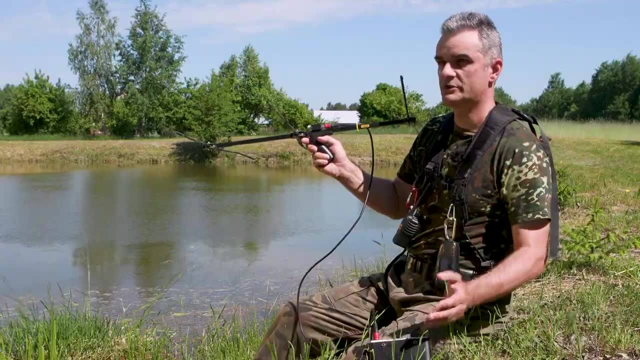 it can select a specific turtle number from the bank. We can see that this turtle is not far from here and now. the signal of the second turtle. This signal is stronger, so it means that the individual is closer, Except that at this point, of course. 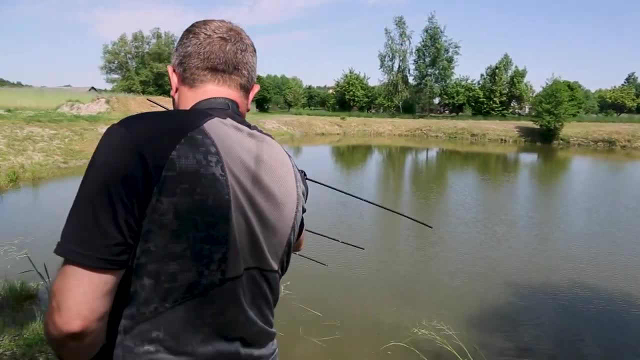 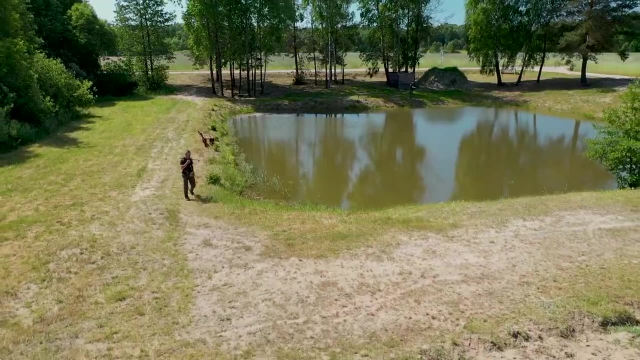 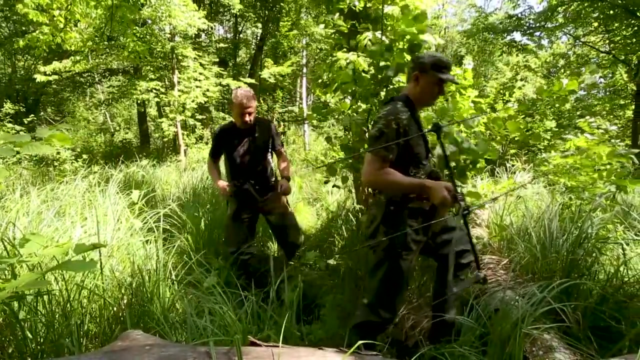 they are underwater. From the collected telemetry data, it is known that group wintering of several individuals in one place occurs. However, it is not known whether this is the rule. This is a new observation in terms of the biology of this species, obtained by using advanced techniques. 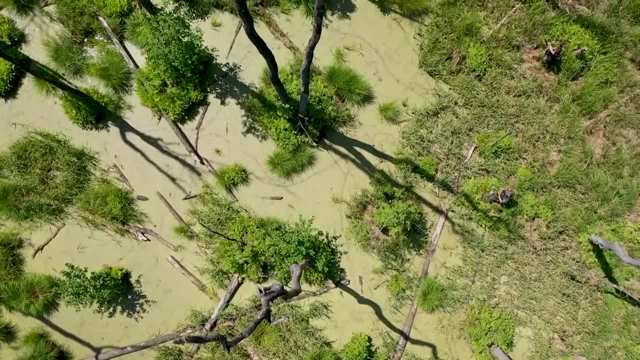 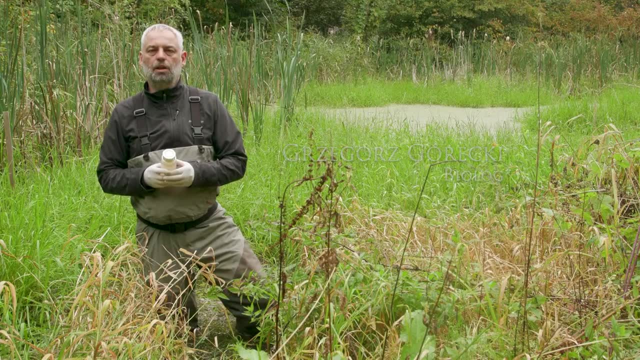 A few years ago, we tried a rather innovative method for detecting European pond turtles, which until now has only been used to detect animals from the fish or amphibian groups. It is the detection of DNA from water, so-called environmental DNA testing. 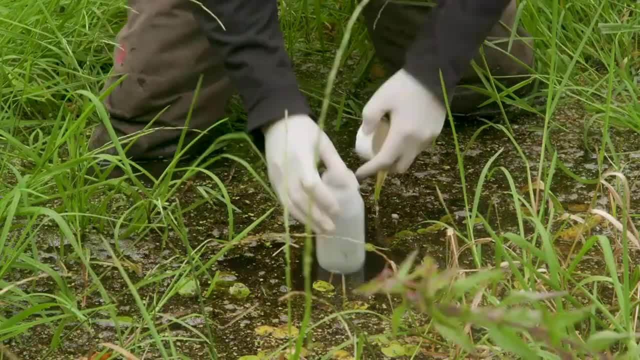 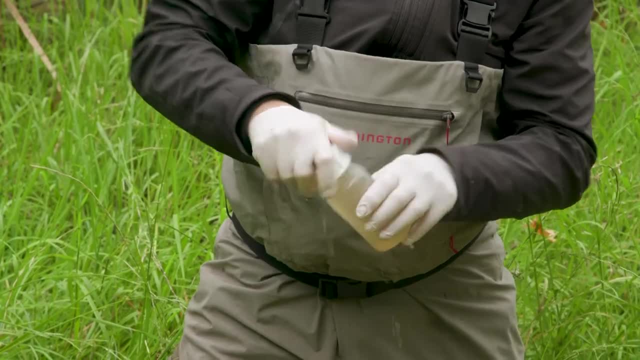 This is the most advanced method of environmental DNA testing. This involves taking a small amount of water, about 250 ml, and then filtering it out and in the laboratory. genetic testing allows us to detect traces of the DNA of the species we are looking for. 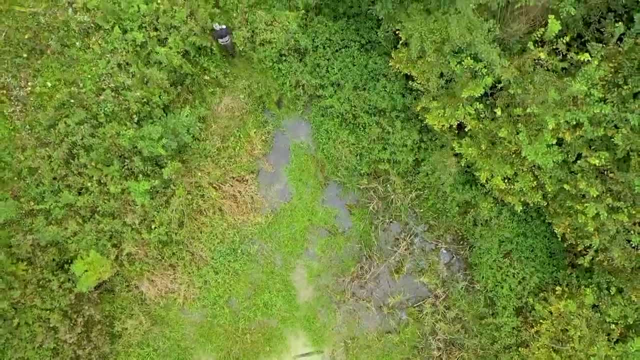 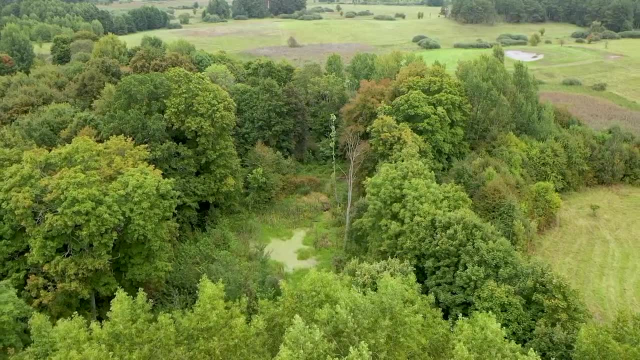 In this way, we are often able to find sites of pond turtles that are otherwise very difficult to observe. The second method, which we have also tested here and which works very well in areas that are difficult to access, is drone searching for European pond turtles. 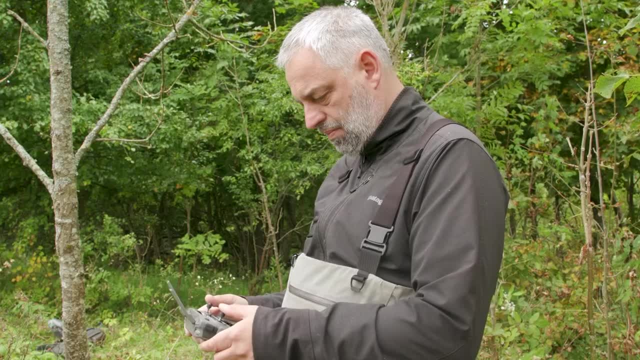 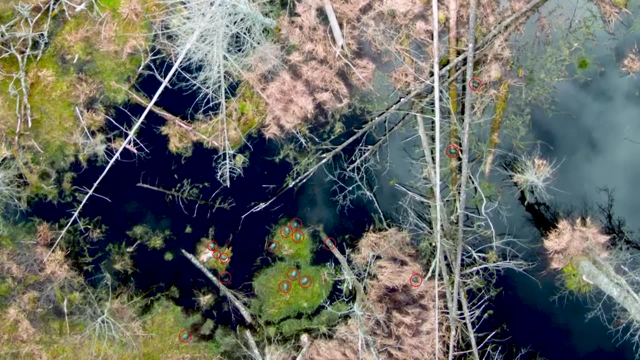 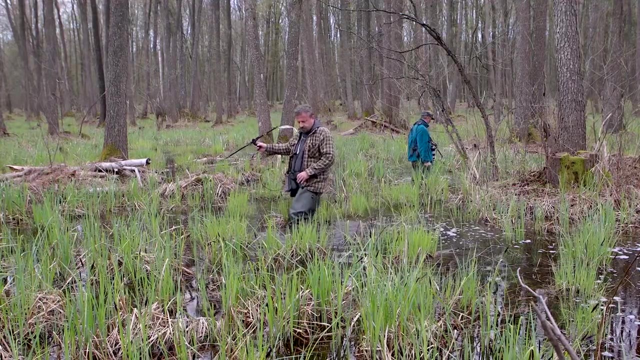 Using such equipment. turtles can often be seen from a height of 40 or 50 meters. You can see them quite well. you can even distinguish the male from the female by size or the young individuals. The location of wintering grounds is important for the proper protection. 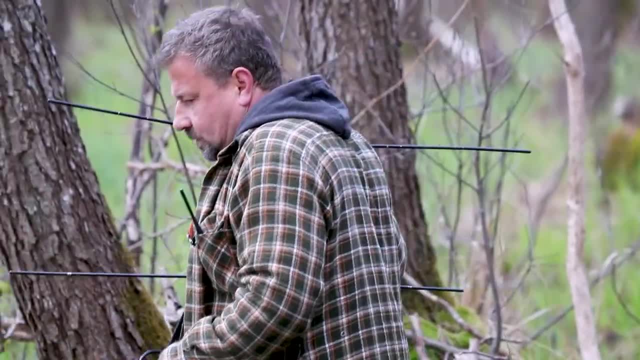 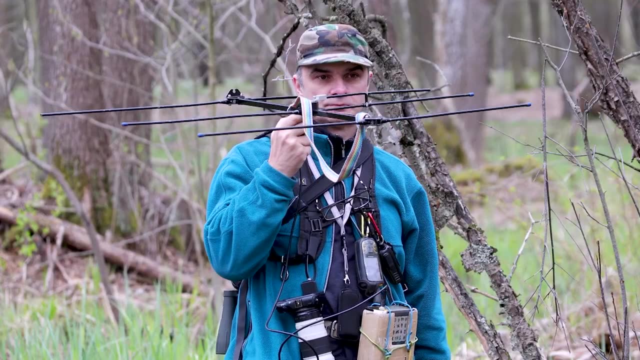 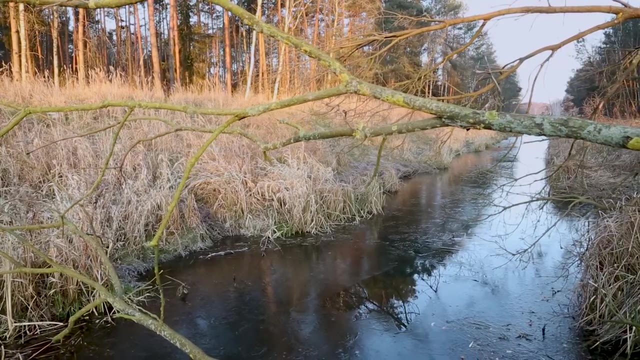 of European pond turtles. It helps to avoid unfavorable events such as the filling up of a reservoir, drainage works, etc. which may lead to the extinction of the entire population of Europe. During their winter sleep, turtles do not feed and their life processes. are significantly slowed down. Heart activity drops to two beats per minute. The turtle actually switches everything off. Everything is switched off. only a little candle is burning somewhere. This is just enough to slowly move blood through the hibernating body. However, 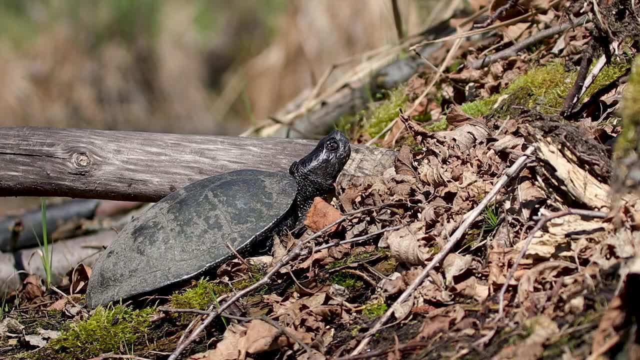 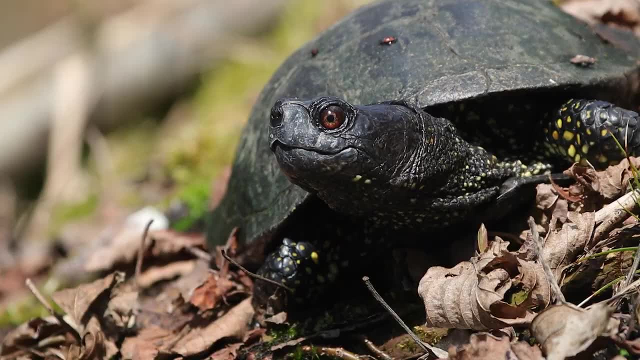 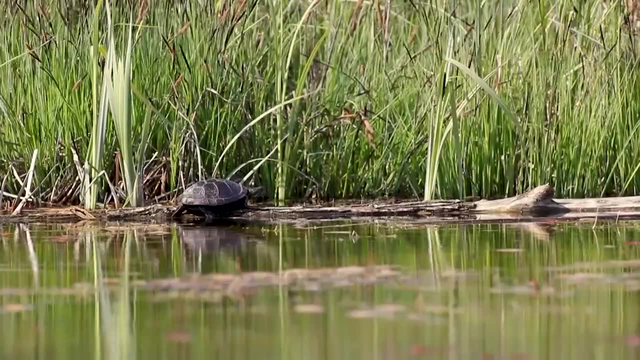 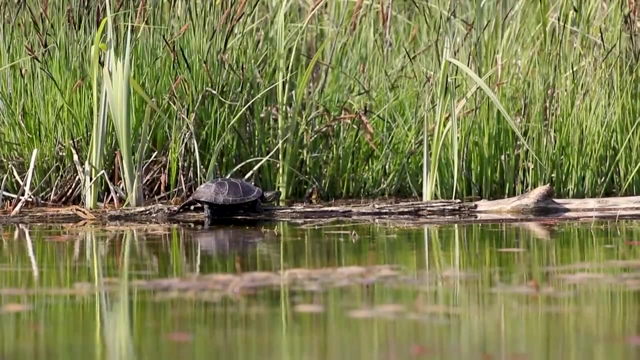 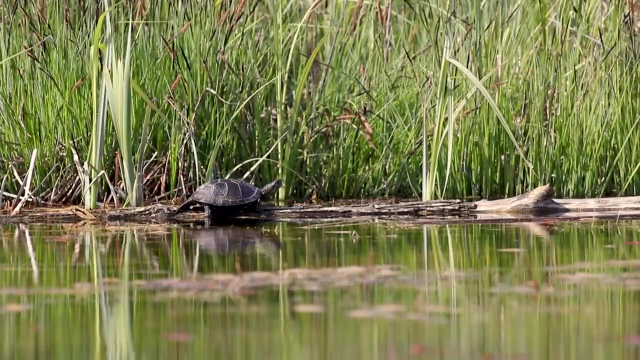 there are sporadic problems that can cause the turtle to die. For example, there are sporadic reports of turtles showing activity under the ice. The European pond turtle has been under strict species protection in Poland since 1935.. It is listed under the EU Habitats Directive. 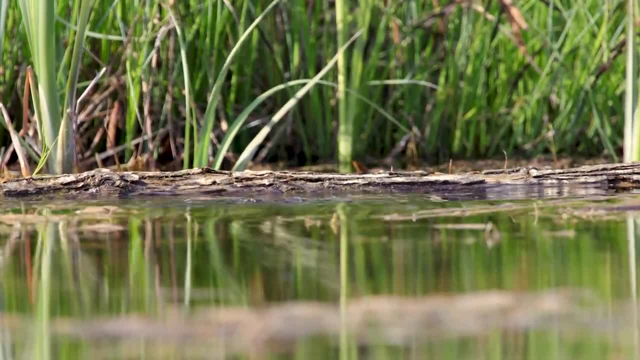 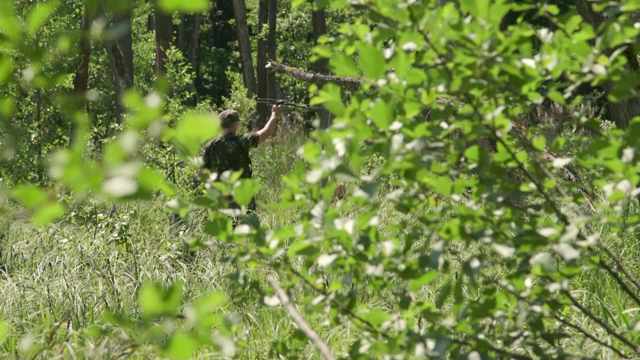 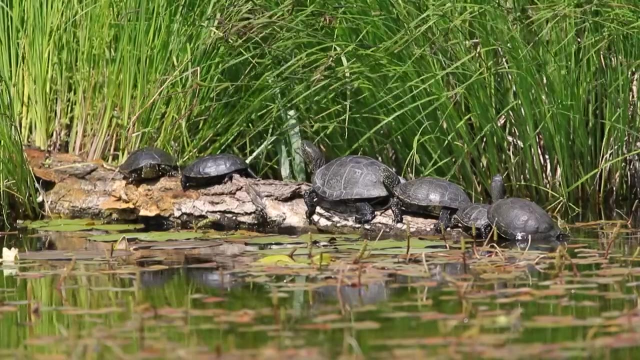 and protected under the Natura 2000 network. However, despite its protection, as a result of significant changes in the environment and land use, its range is gradually shrinking and further sites are disappearing. The turtle cannot be protected without preserving the environment in which it lives. 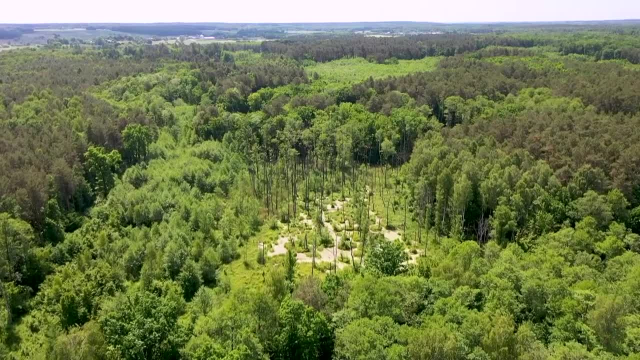 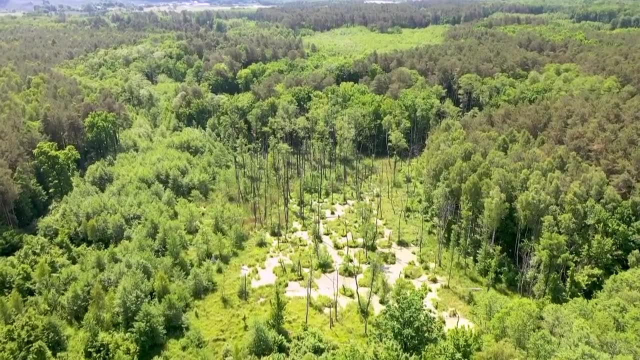 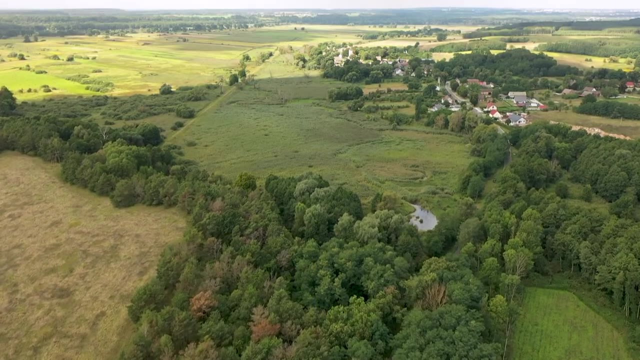 That is why projects for the active protection of the turtle have been carried out in Poland for many years and have involved foresters as well. We are now in Rybocice, on the territory of the Rzepin Forest District. It is the richest and most numerous site. 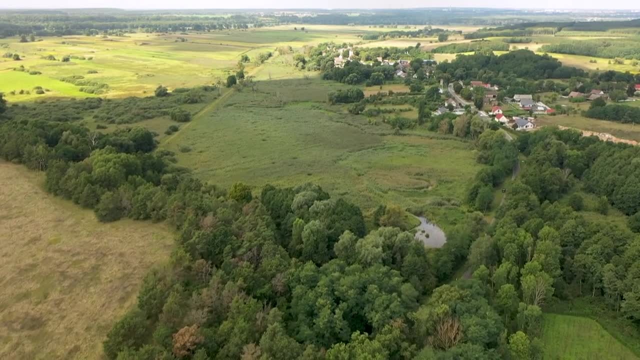 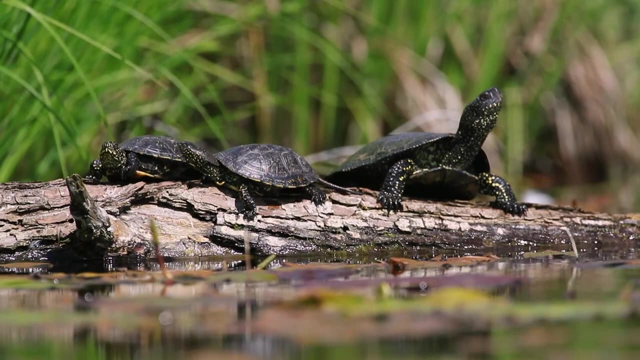 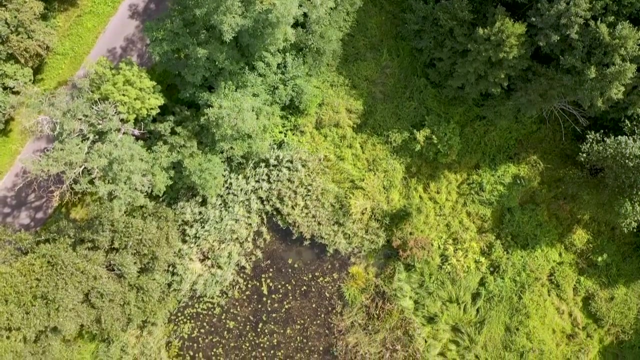 of the European pond turtle in western Poland. We have about 100 individuals identified here, so it is a really rich and numerous population. As part of the life project, several activities have been carried out here, generally related to small retention. Larger water reservoirs have been dug. 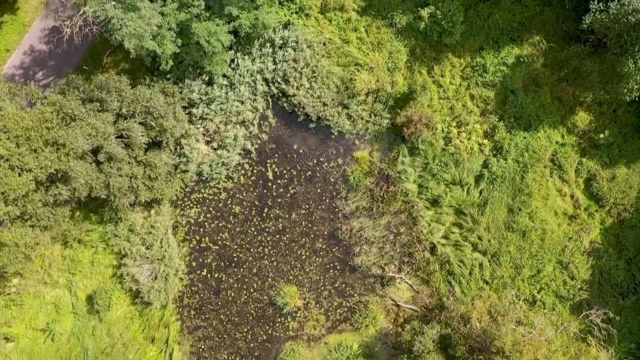 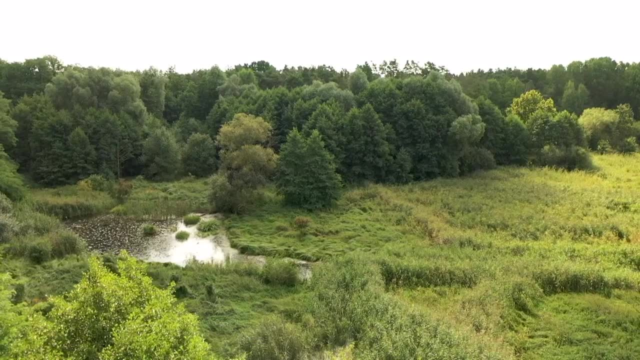 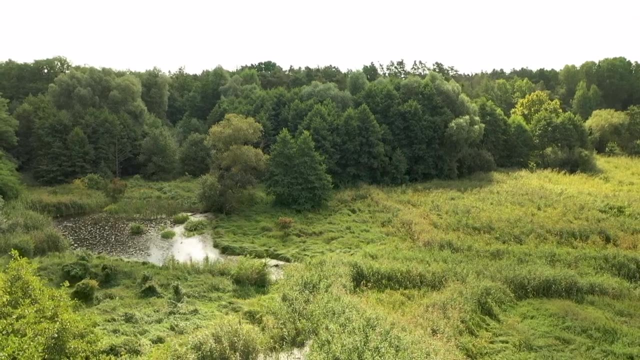 for older turtles, but also small reservoirs for smaller turtles. Dykes were built on existing ditches to improve the moisture conditions. The water level has risen and this has improved the habitat for the turtles. The breeding ground is periodically cleared of self-seeding plants.